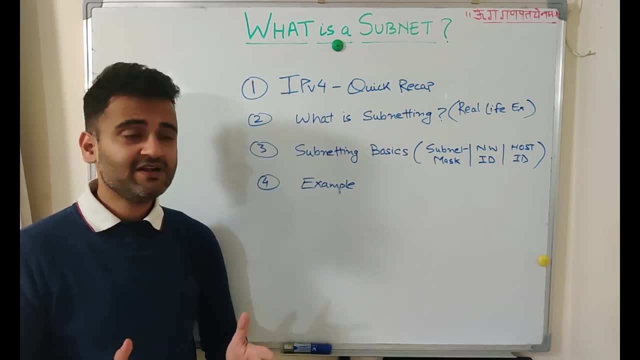 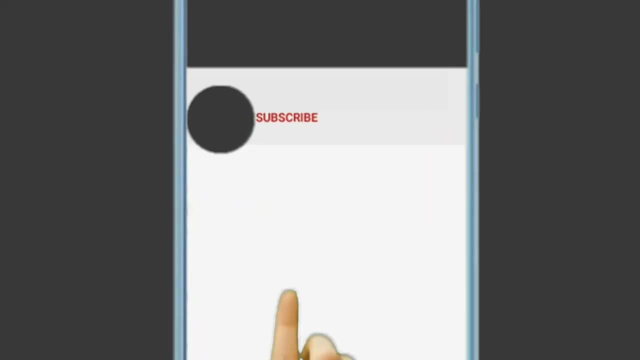 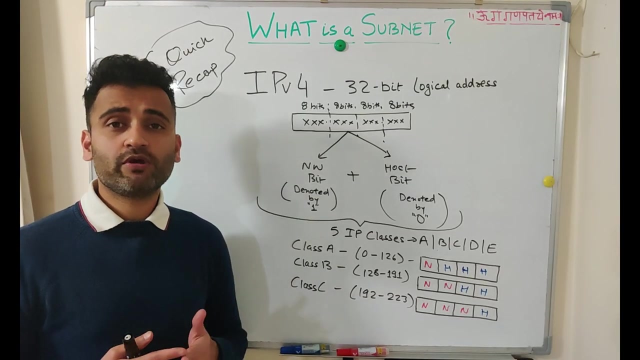 cider range and all those concepts, and at the end we will take a simple example to understand it into reality. so let's get started. please subscribe to my channel and hit the bell icon. so, friends, let's do a quick recap of what we learned in our previous video. again, this will 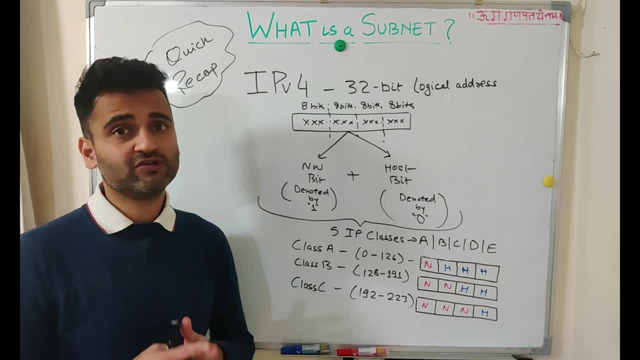 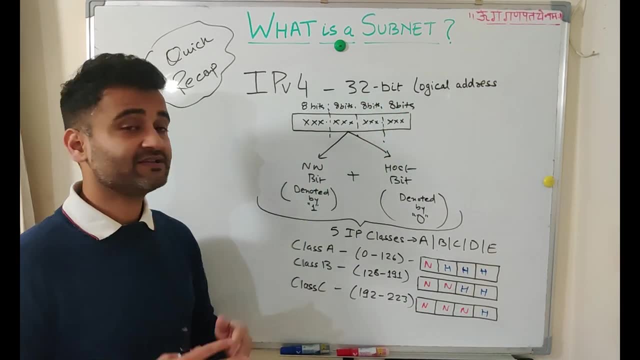 be a very, very quick recap, so i would highly recommend that, if you are new to this concept, go and check that video in detail. so an ipv4 address is a 32-bit logical address wherein you have dotted decimal notation to give give a unique identity to. 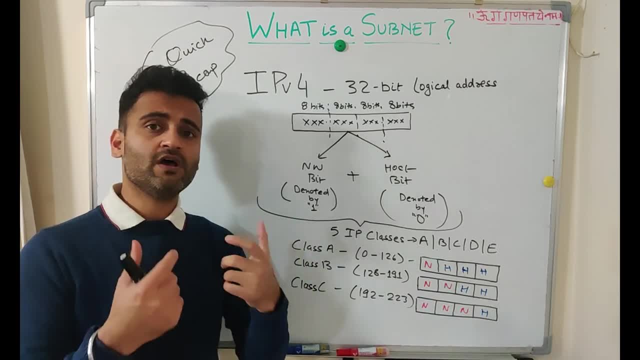 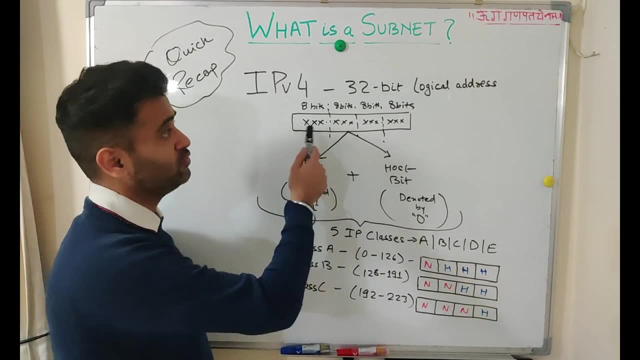 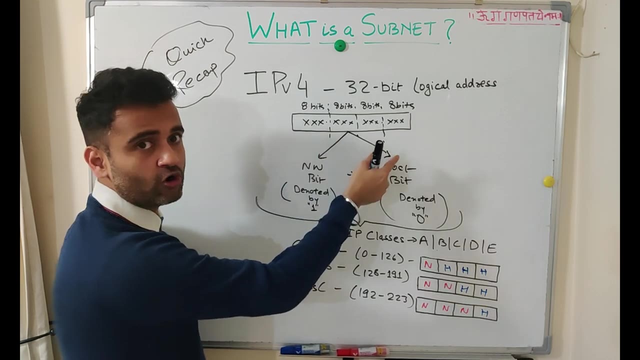 device over the network. so every network device would have an ip address with which it would be identified uniquely over the network. again, these are divided into eight bits and, uh, you know, every, uh, every particular set is called as a octet. okay, so we have four octets, so eight into four we have. 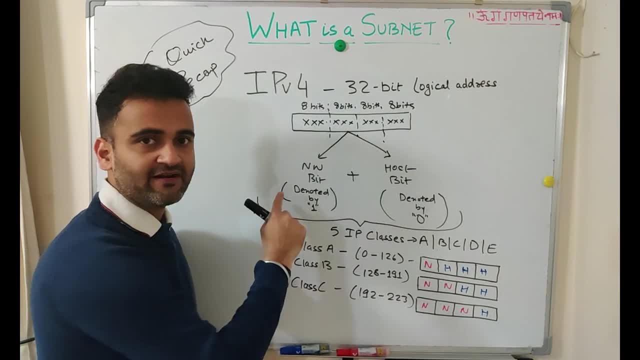 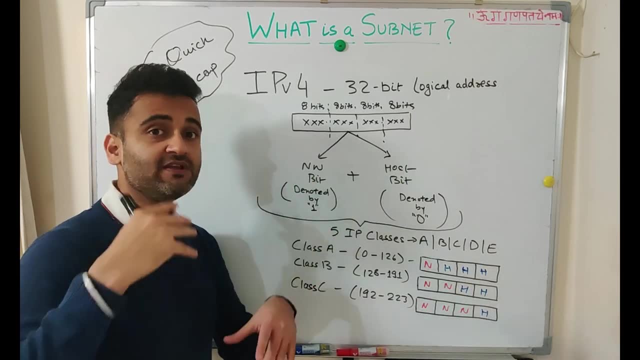 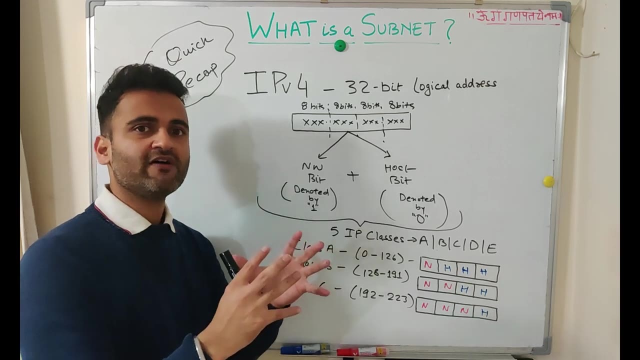 32-bit logical address. now this particular ip address will have two components. one would be your network bits, another would be your host bits. now how it will vary we will understand. but understand that every ip address is a combination of some network bits and some host bits. so if you have 32 bits, you can have 16 bits of network and 16 bits given to the. 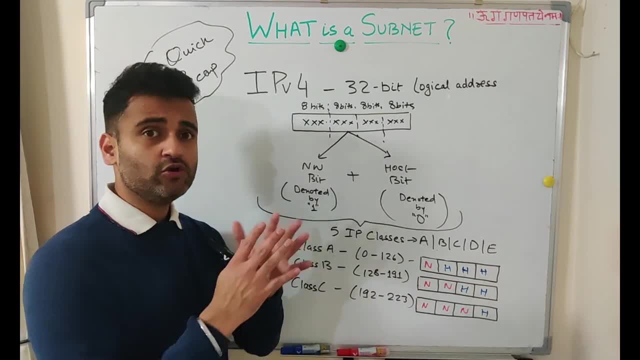 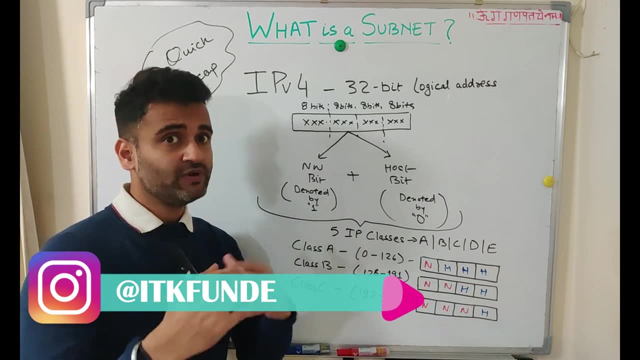 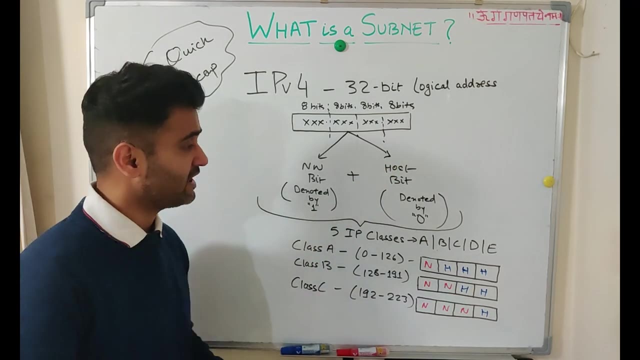 host and like that. so always remember that your network bits are always denoted by 1 and your host bits are always denoted by 0 when you are doing subnetting. you will come to know about this when we will go into more detail again. your ip address is categorized into five different classes. class a: 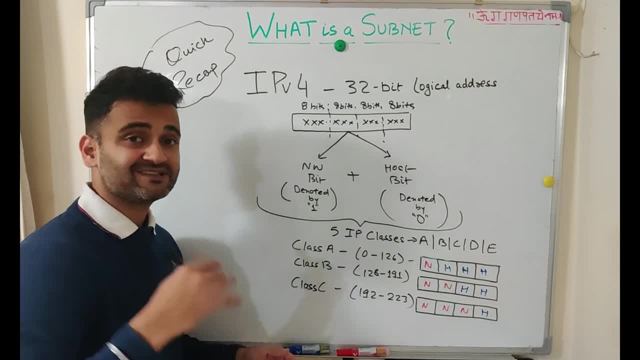 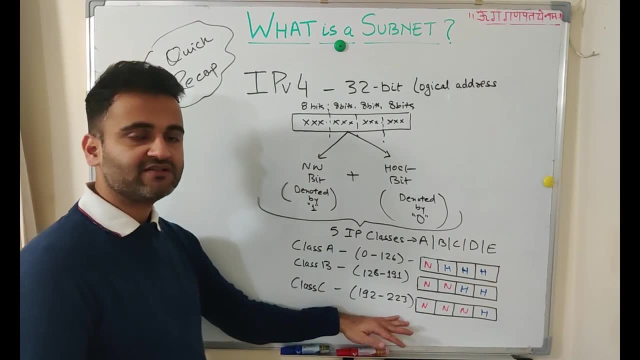 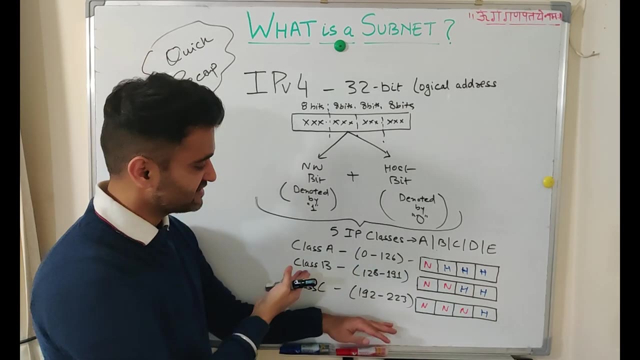 b, class c, class d and class e, and we are not discussing class d and e. if you want to know more, you can watch that video. but for now these are the three primary uh ip address classes which are used uh today and these are the ranges for the same. so class a ranges from 0 to 126. class b is from 128 to 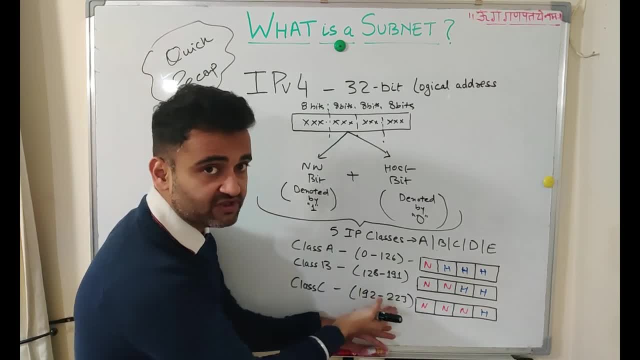 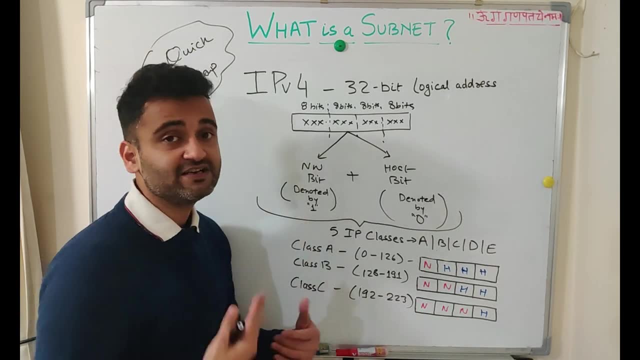 191 and class c is from 192 to 223. so just by looking the ip address of any kind, you can identify that which particular ip address you are using and you can identify that which particular class it belongs to. so, based on your ip address classes, you identify that how much bits are given. 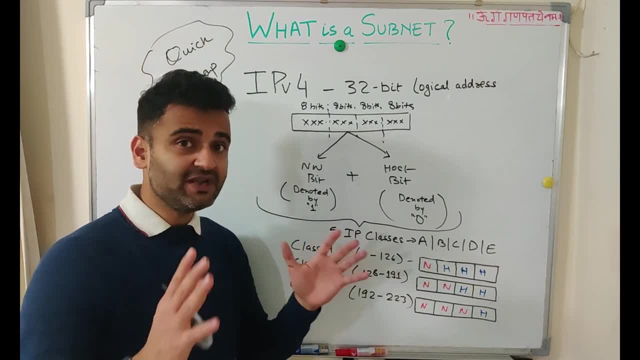 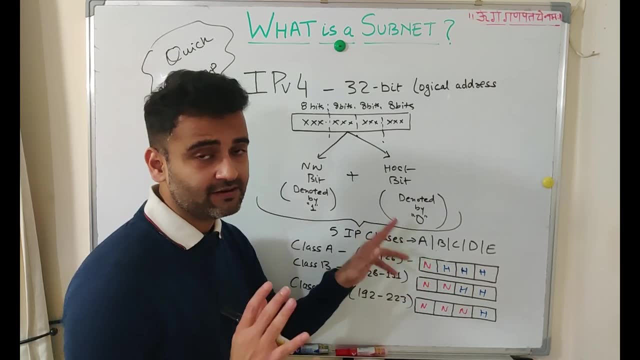 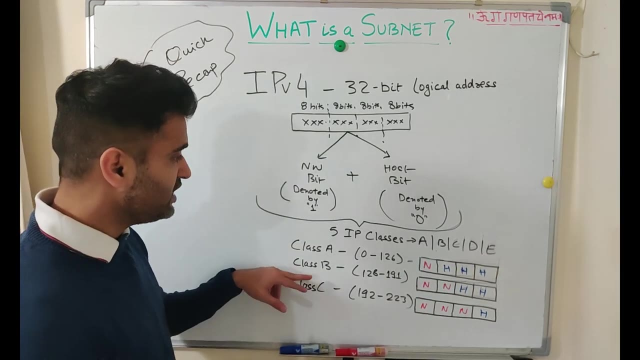 to the network and how many bits are given to the host. it is predefined. so for a class a it is mandatory to give the first octet or your first eight bits to the network and rest are for the host. so eight, eight, eight. these three are given to the host. and in class b we have first two octets. 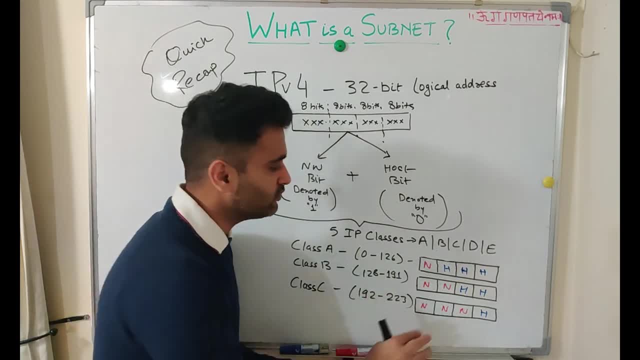 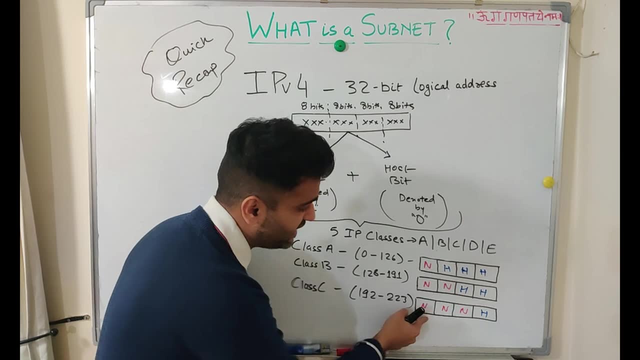 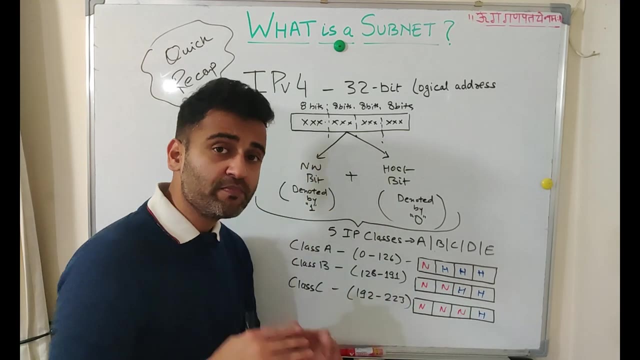 one octet is eight bits, so eight and eight, sixteen for the network, sixteen for the host in class c you have, uh, you have first three octets which are eight, eight, eight, twenty four bits given to the network and only one particular octet or eight bits given to the host. so, based on your need, you, 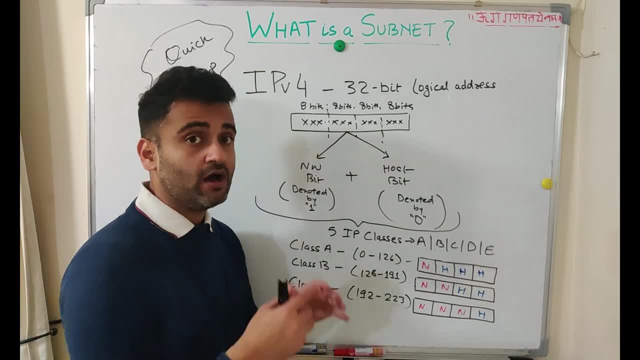 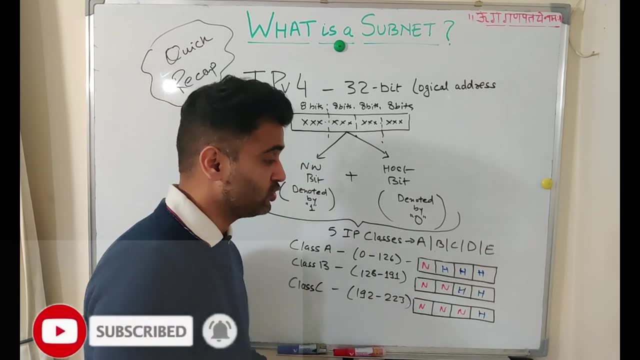 decide whether you need a class a, class b or class c. uh ip address range again. uh, we have gone into more detail in our last video, so go check that out if you want to know more, but this is good enough to uh have a basic understanding of how you know these ip address. 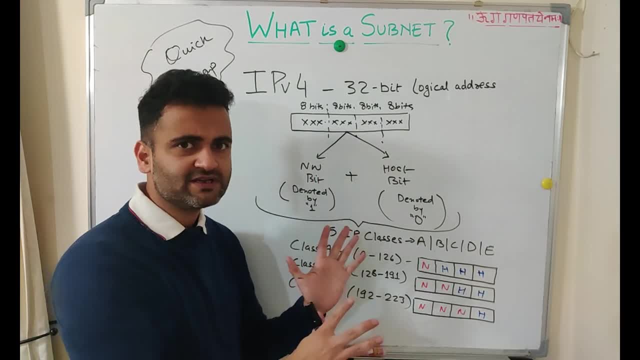 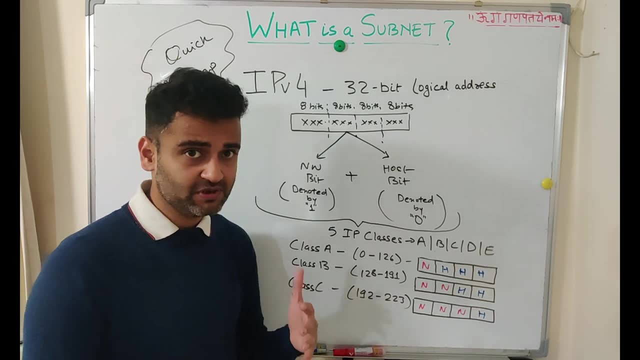 classes are defined. now we- this is, this is pretty much about ipv4. now we will go to subnetting and we will try to understand it from a layman perspective, taking a real life example, and then we will touch base upon some of these concepts when we will go into the core of 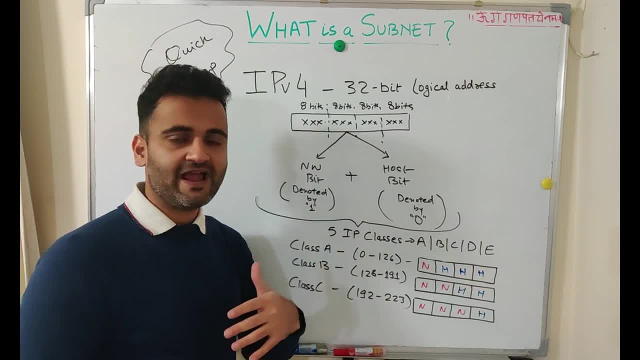 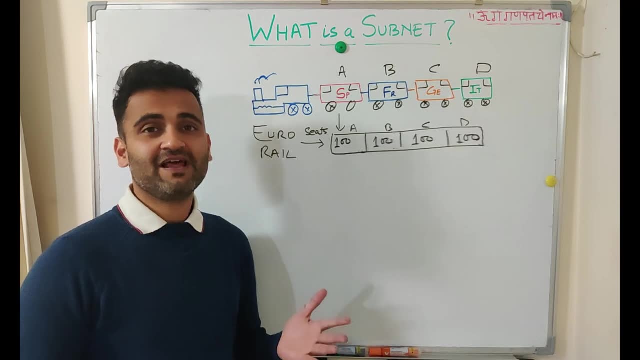 networking fundamentals. so let's let's take an interesting example. so let's start by an interesting real life example. so let's take an example of this euro rail. euro rail is a famous railway service in europe which helps passengers travel europe going across country. so suppose this: 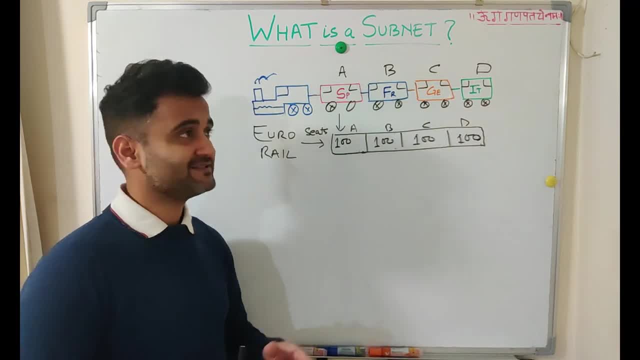 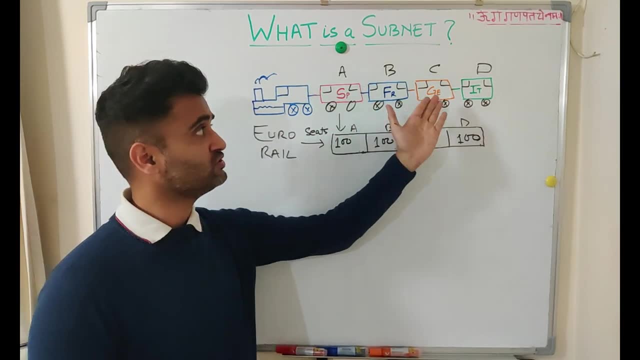 is one of those trains where we have four different coaches and every particular coach is reserved for a specific country. so coach a is for spain, coach b is for france, code c is for germany and coach d is for italy and by default we have 100 seats built into. 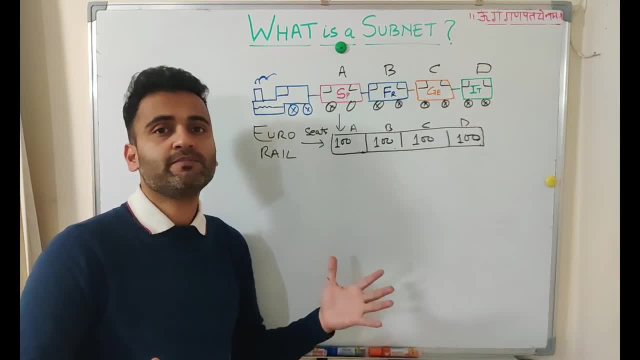 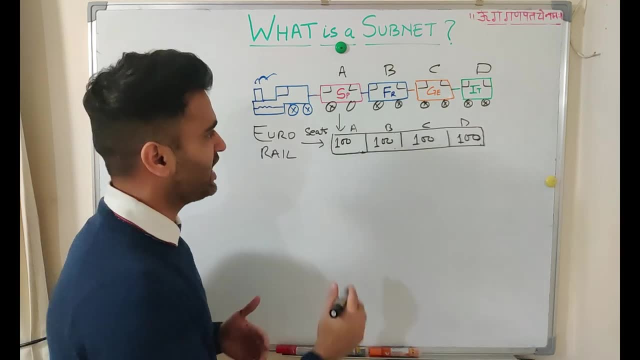 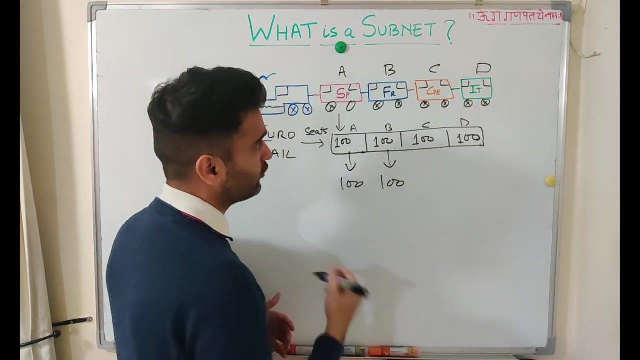 these coaches and you cannot have more than 100 passengers, obviously because you have only 100 seats available. but just suppose, just before the journey the bookings opens and a booking for spain goes 100 full and for france also it goes full. for germany it gets overbooked, so it goes to. 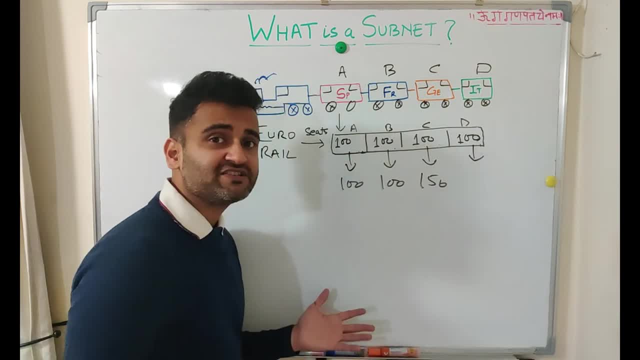 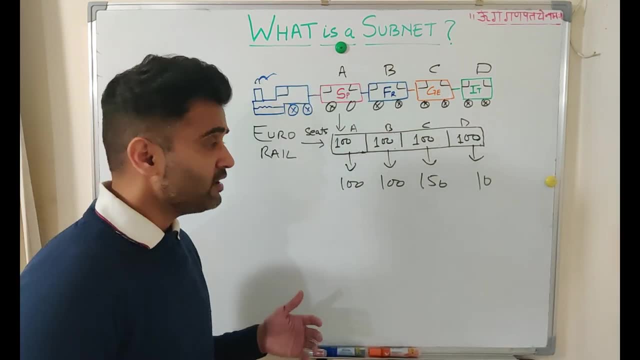 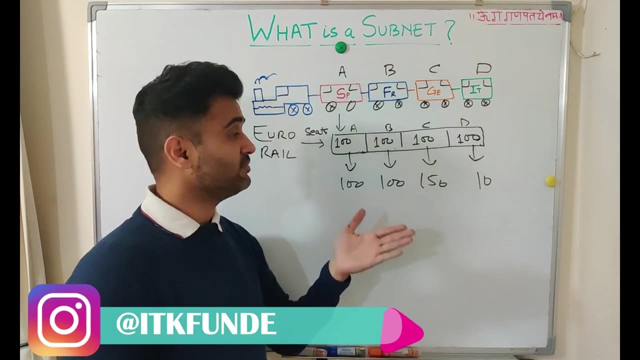 150, and for italy it is only partially utilized and it goes to take, for example, 10.. okay, so now there is a problem because we have more passengers going in germany. okay, but they cannot accommodate that, because germany has only 100 seats available and those 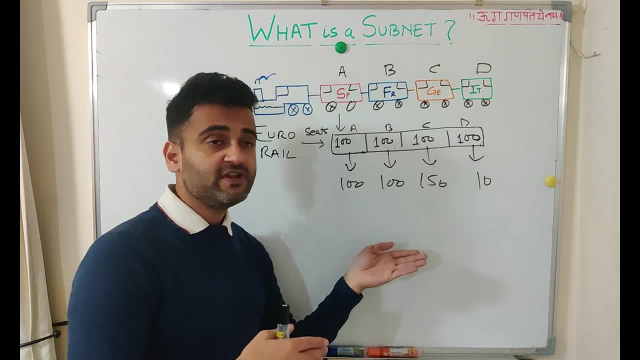 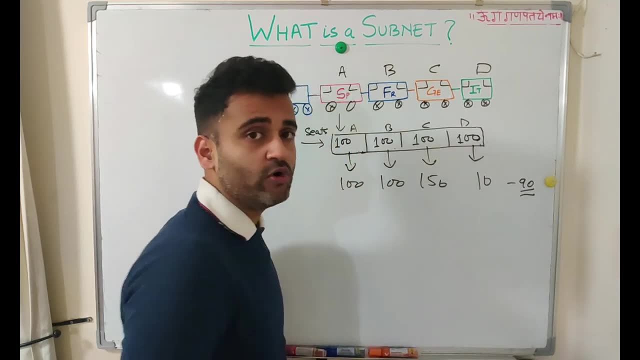 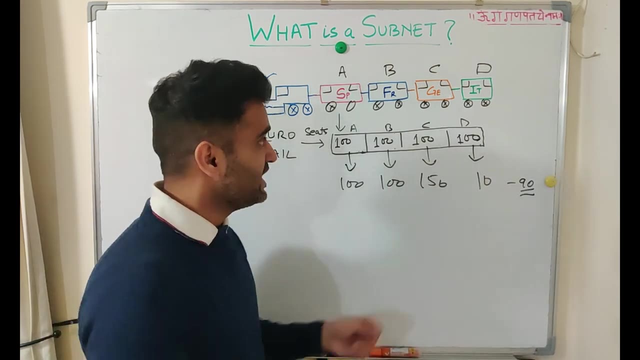 all are filled, but then the service would lose on to those 50 passengers wherein, in italy, we are losing anyways, because out of 190 seats are anyways uh going as vacant. okay, so a general uh phenomena. what we see is that these 50 passengers can be accompanied. 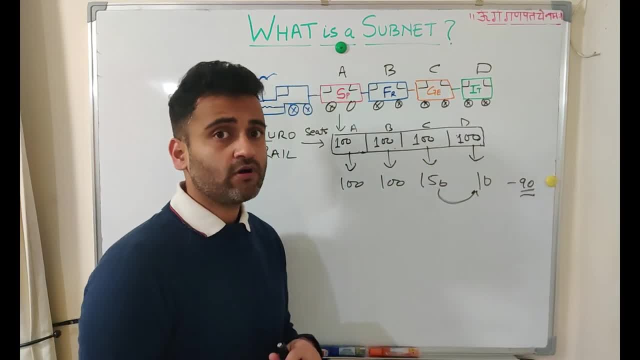 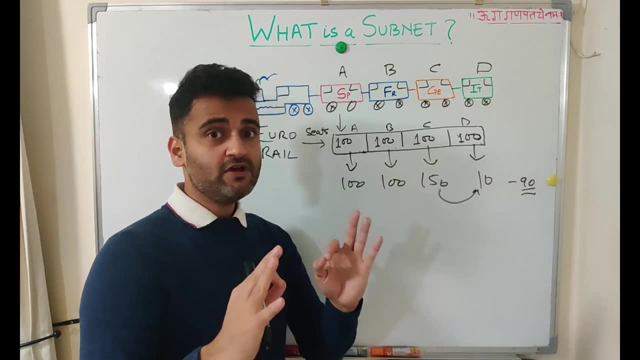 by one of our coaches for 40 minutes, which is the only way for the coach to get into his seat. but in fact the coach can go in and get to the seat three minutes earlier and in that place the coach will be able to carry all the passengers. most of the passengers will be being taken away. 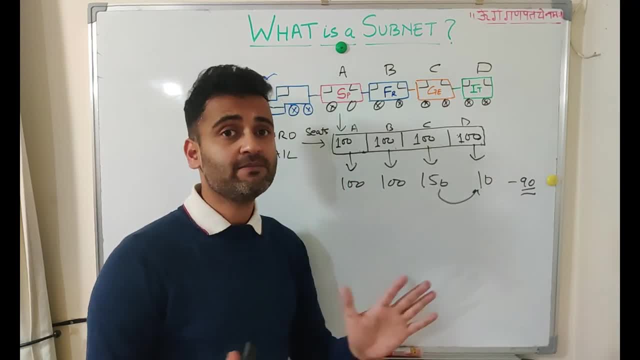 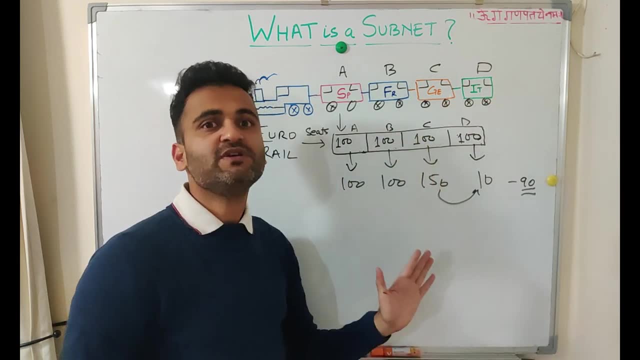 so in the case of this coach as well, he's only performing two shifts and down. all the passengers would be cast aside, or he is not enough for the행t and he would be 91.. the coach may not be able to carry more passengers, but the coach will be. 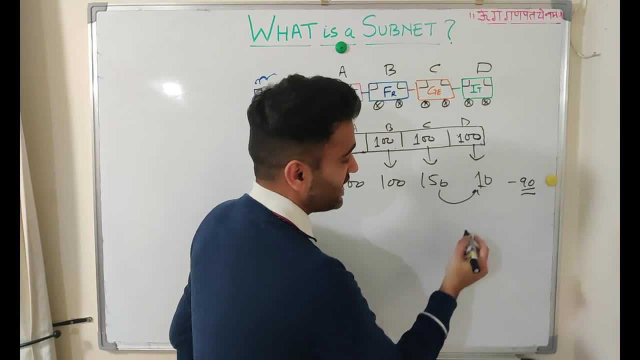 able to carry a lot of passengers, so one of those passengers would be cast aside, and if he is not available in a couple of minutes he may get stranded somewhere else, and so on. so that is how the issue is. even if we add 10 more, it goes to your 20 reserve quota, so we still have 10 more seats. 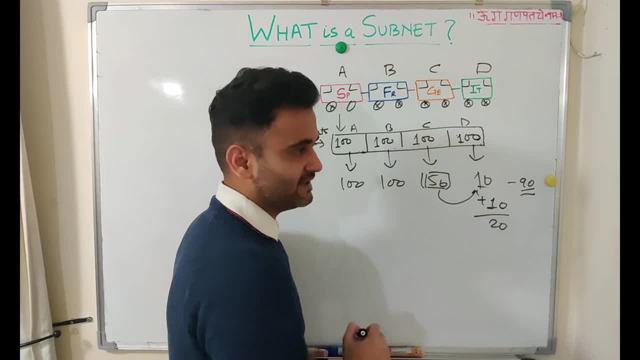 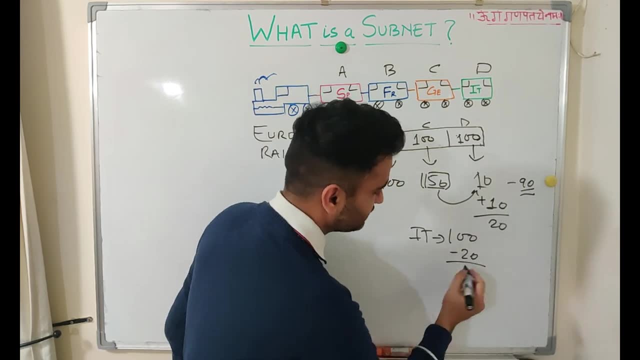 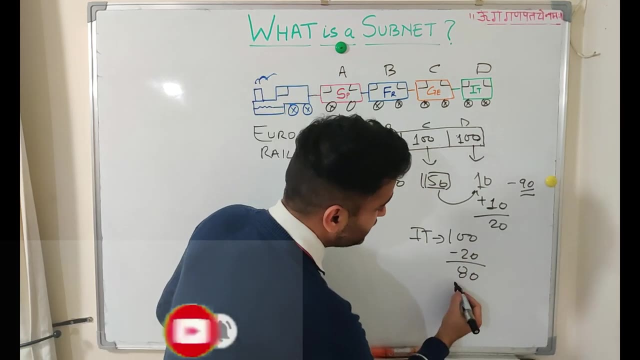 available here and here we only need 50 to be adjusted. so even if we, if we take 100 for Italy, okay, and up in that, we minus the 20 reserved seats, so we are left with 80, 80 seats are still available. so what will be done? these 50 passengers will be adjusted into this and 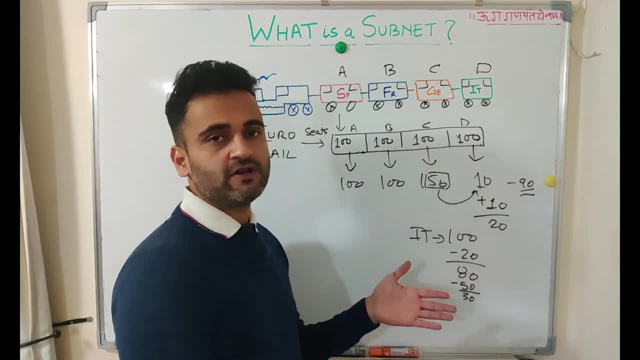 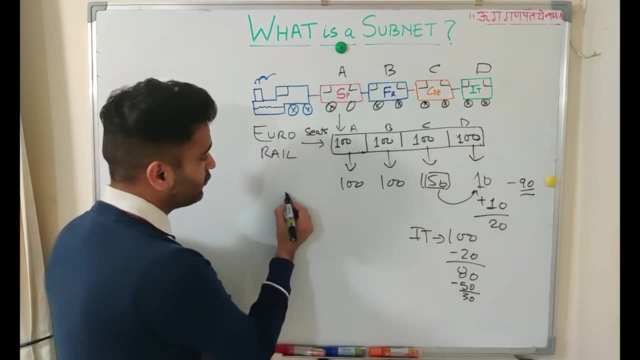 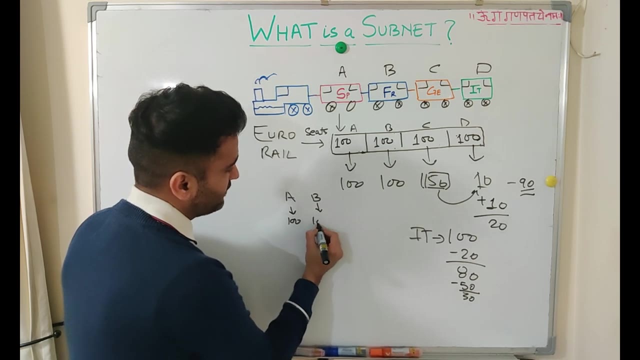 still, it will have 30 seats left, which is fine, because now everyone has been adjusted. so what would be the new setup? new setup would be that, obviously, for Spain, compartment A, we have 100, which is not a problem. for compartment B, France, we have 100, that's not a problem. 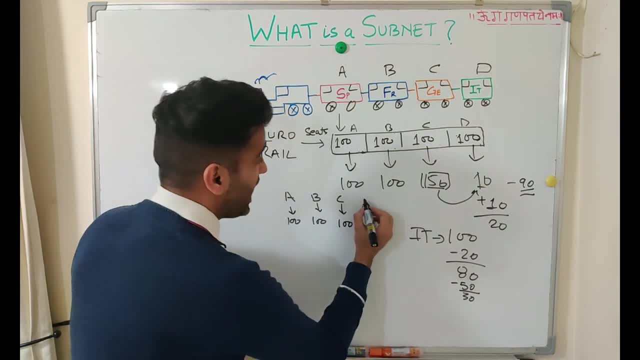 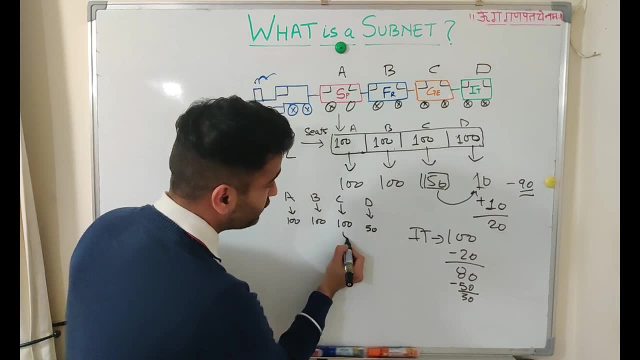 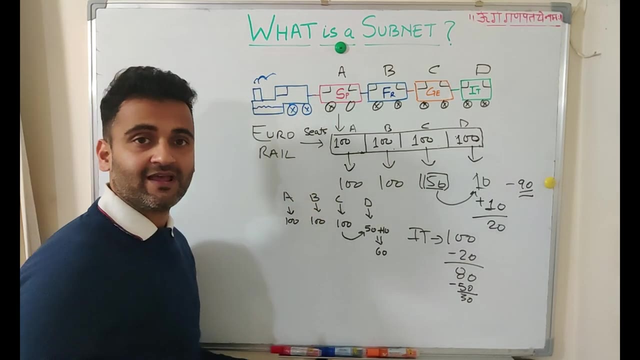 for compartment C also now we have for Germany, we have 100, and for compartment D: now we will have 50, which were moved from here to here Here plus the existing 10, so it will go to 60. you are understanding my point right, so 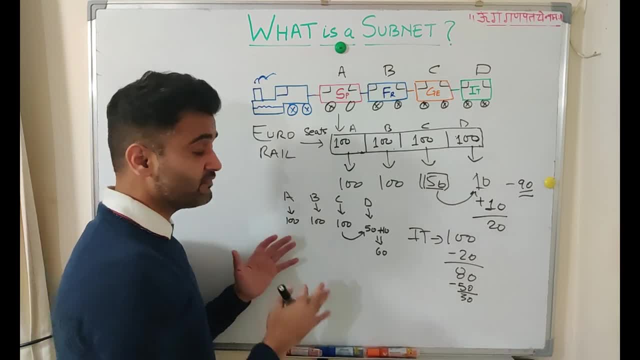 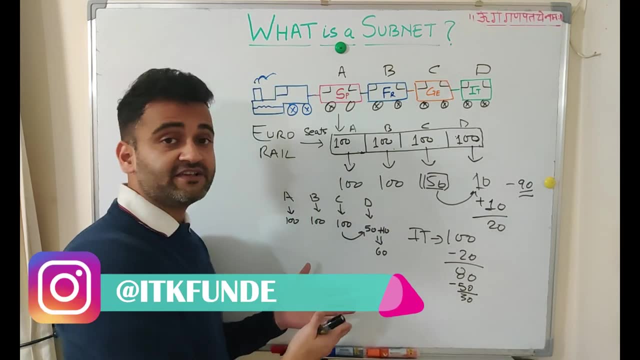 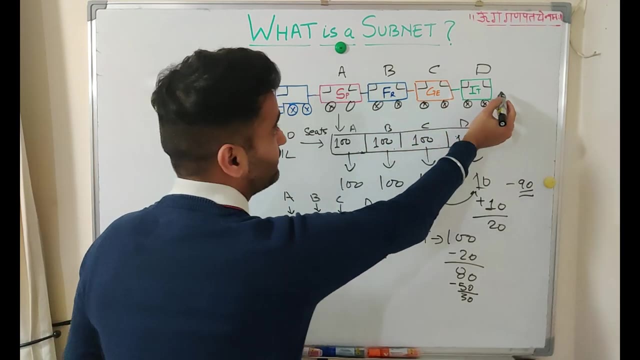 what it did it what what the railway service did. railway service adjusted some of the passengers from this particular compartment to this compartment to allow more utilization of seats and reduce the wastage of resources because unnecessarily, you know, Italy coach was anyways going most mostly empty. This is the example. 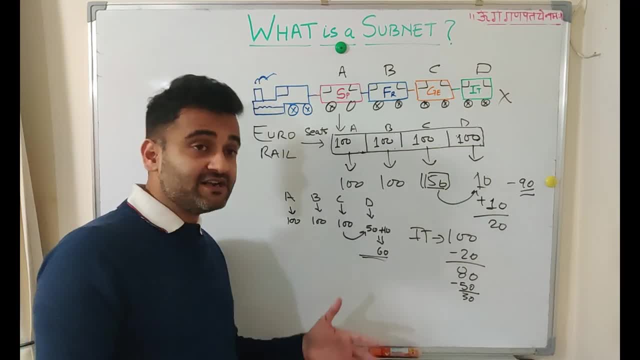 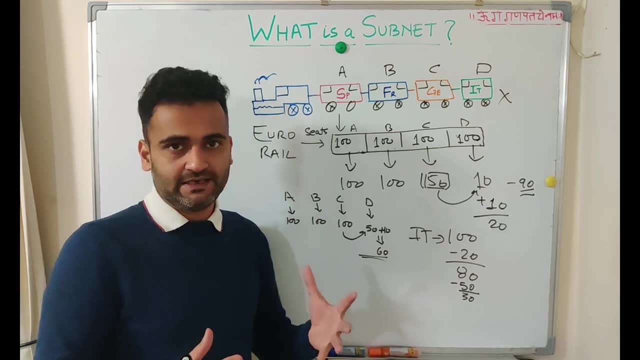 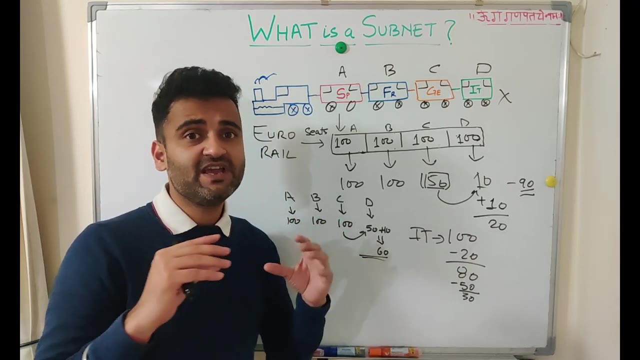 This is the exact way subnetting works. so now, subnetting what exactly does? which, which we will understand, is it helps you utilize your network network bandwidth more intelligently. so, as we just now saw, that we have already predefined network and host bits for your class A, class B and class C, but suppose you have a requirement wherein you do not require? 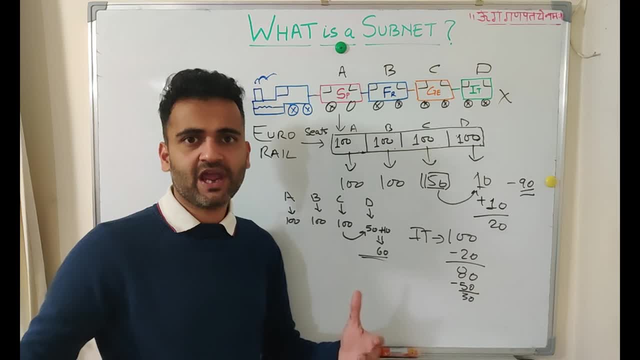 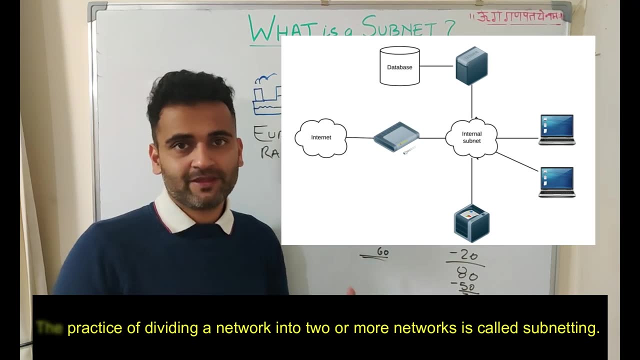 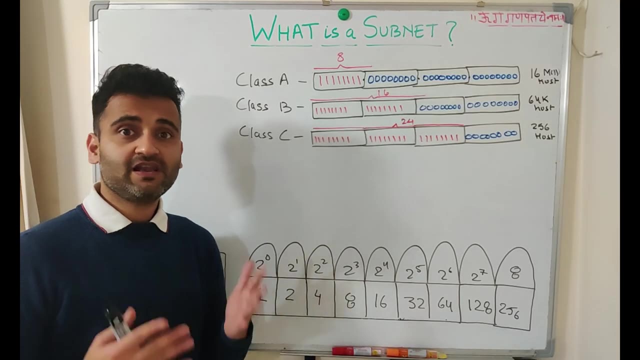 so many networks to go waste or so many hosts to go waste. okay, in that case, you divide one particular network into multiple sub networks based on your usage, and that is precisely what is a subnetting. so, friends, in a typical class A, class B and class C IP address ranges, we already have predefined. 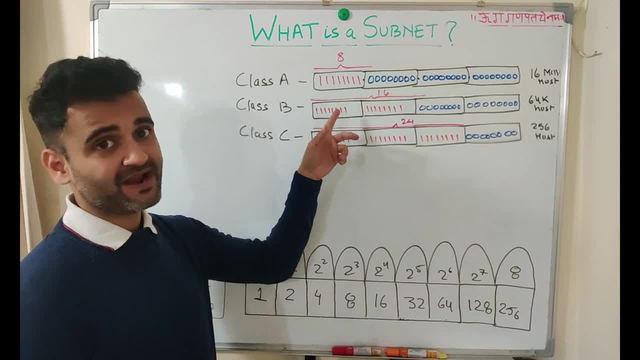 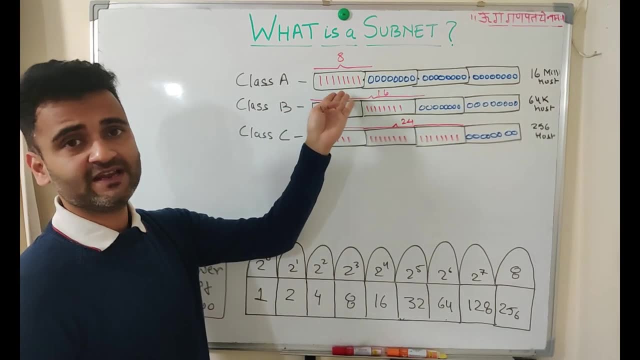 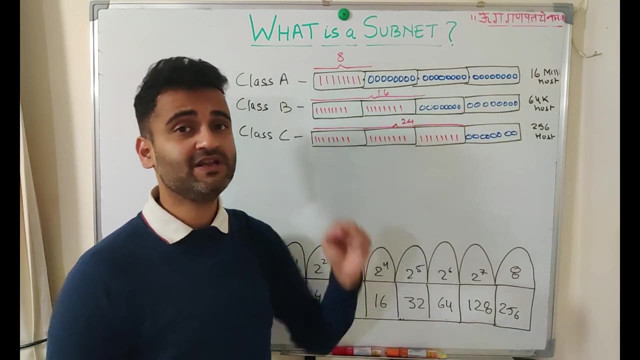 number of bits dedicated to network, which you see in red and rest are, you can see in blue, are for the host. so, as you can see, for class A we have eight bits dedicated to the network and rest 24 are dedicated to host, which results in around 16 million hosts in. 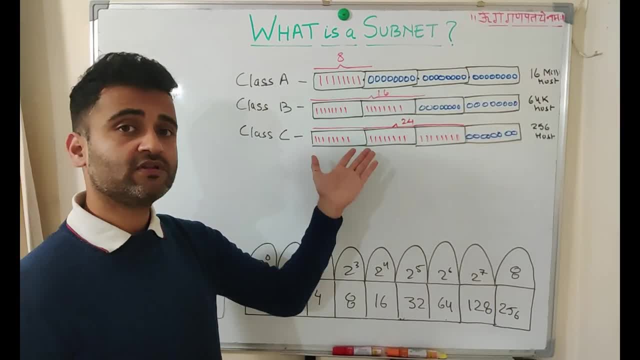 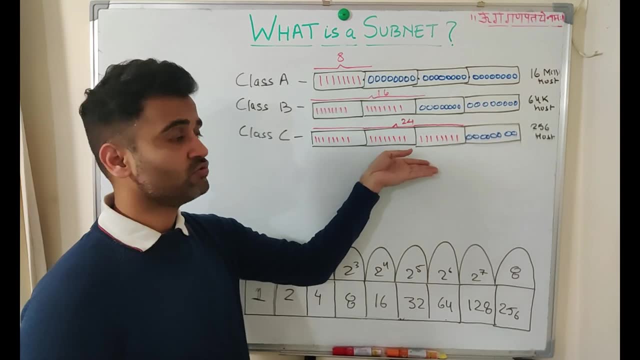 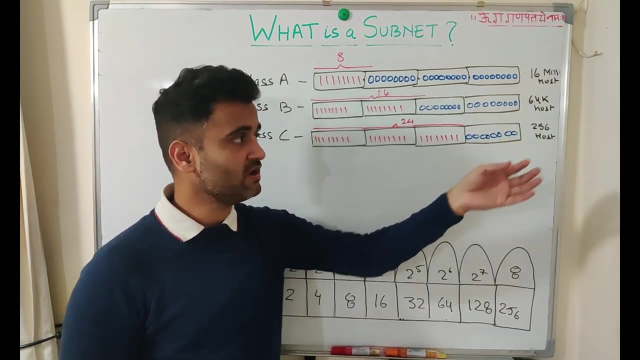 class B, we have 16 for you know, for the, your network, and 16 for your host, which results in 64,000 hosts. and for class C, we have 24 dedicated to network and only eight bits given to the host, and that results into 256 hosts. okay, now you might be wondering how I'm coming. 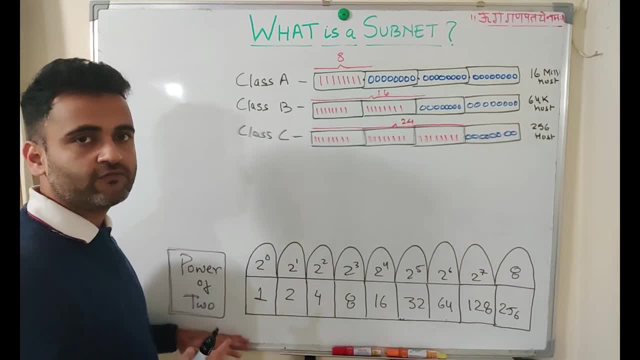 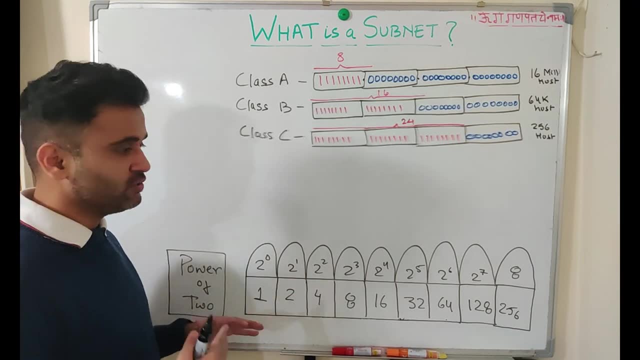 to this calculation. So, friends, I always remember this power of two in decimal and while working with IP addresses or overall networking, you it will, for you will find it very handy. So whenever you want to calculate any, you know, any decimal number based on your binary. 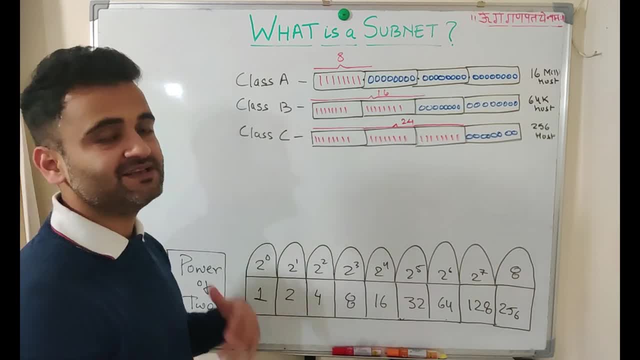 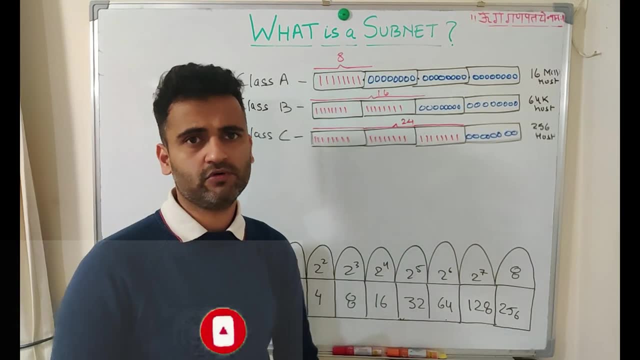 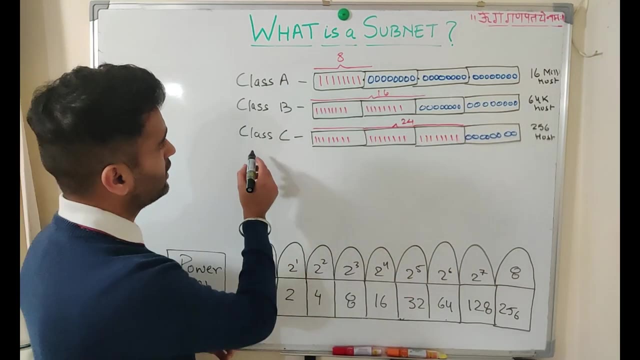 number, then you can use this power of two. we will see this, how okay. So just understand that if, if you get any requirement for around 500 computers, suppose you have to put 500 computers in your office into your particular network address- Now, obviously class C you will first go for, but in class C you have only 256, you know. 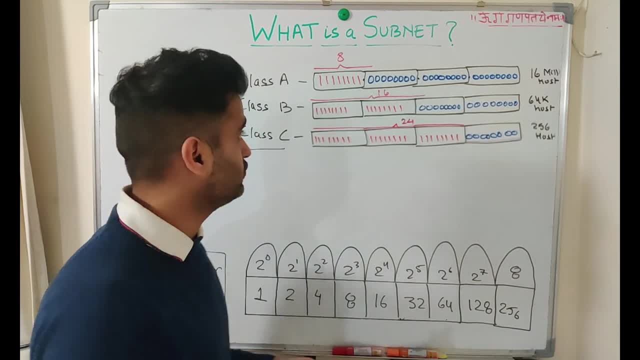 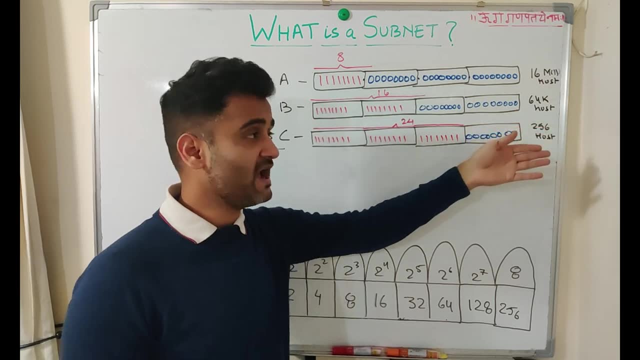 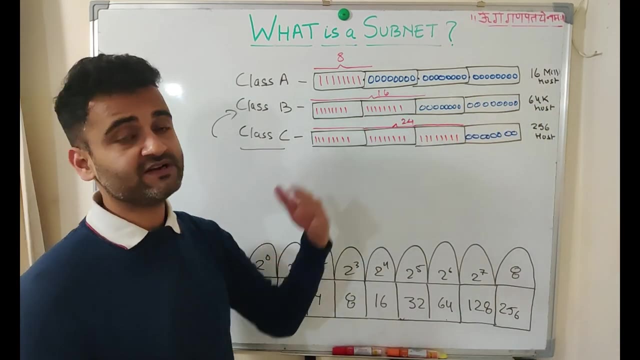 hosts available. So the only option which is left for you is to switch to class B. but then the range is so high- you know there are 64,000 hosts there and you just need 250 more odd host to be adjusted and for that you will waste so many. you know host bits or the. you know host IDs. 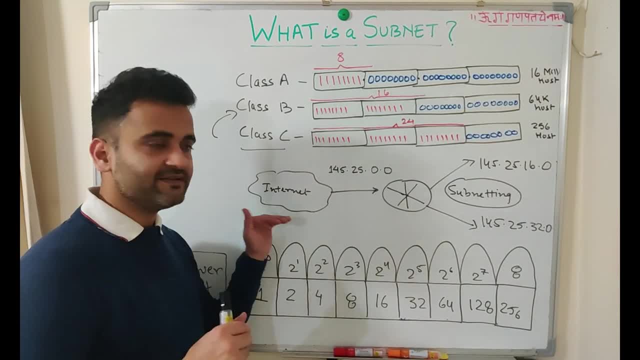 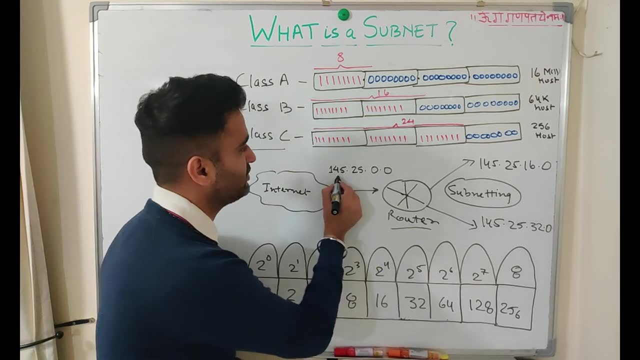 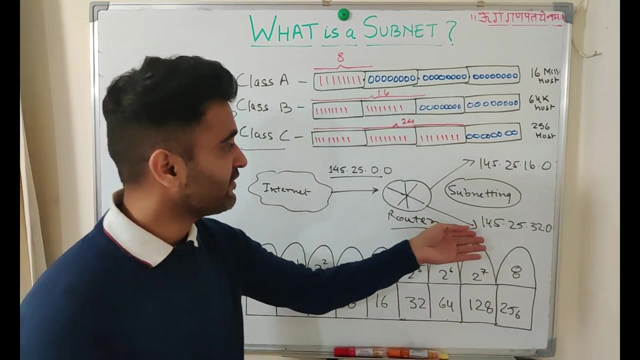 which can be utilized more efficiently. Okay, So there is a network connection coming from internet and going to your router. Okay, And this router has this particular IP address which is coming in and now it has to, you know, it has to distribute it into multiple subnets, so it can divide that using subnetting. 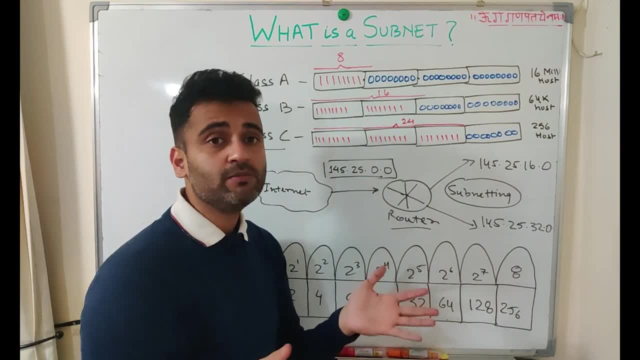 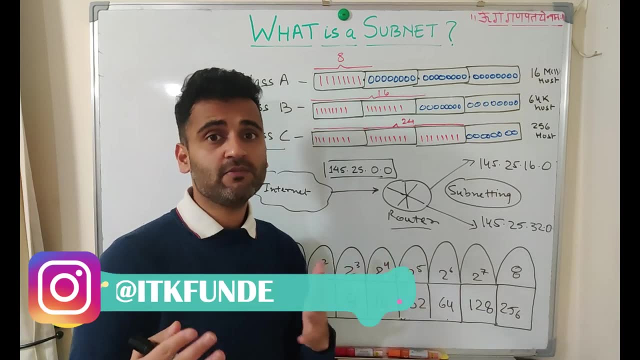 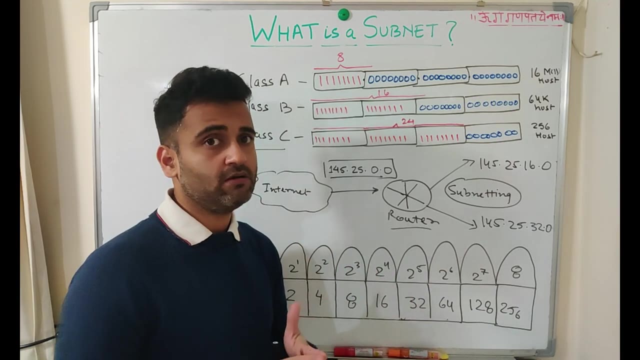 Okay, else you know this whole network. this whole network will might not be utilized fully, so you can divide it into five different subnets. Just remember, like in our one of our very famous videos on networking we took example of a school, So in a school we can have one particular- maybe you know- network coming in. 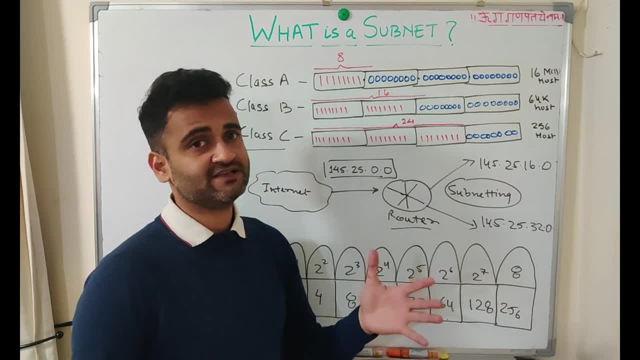 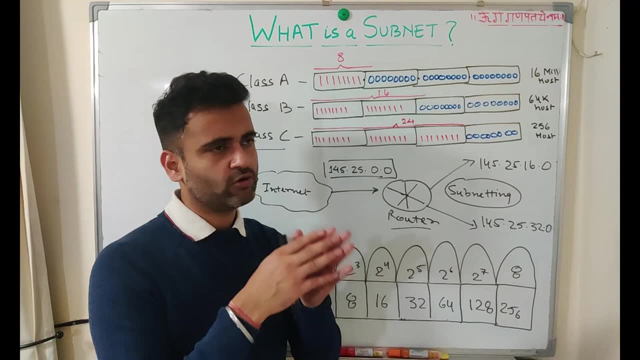 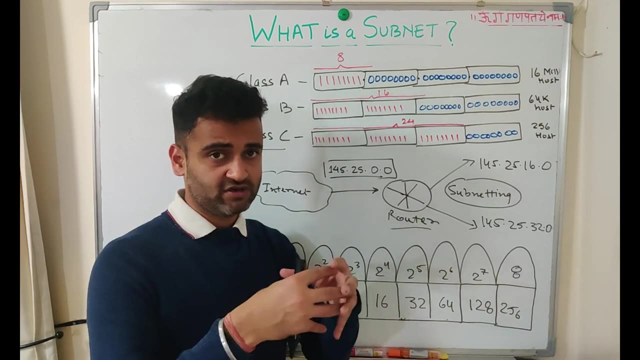 Okay, and then it could be divided into five different classes. Okay, so based on that, based on your utilization, you can have one network coming from your internet or any any other outside network to your router, and then your router, based on your subnetting- what subnetting you have done, will distribute it internally. so far, 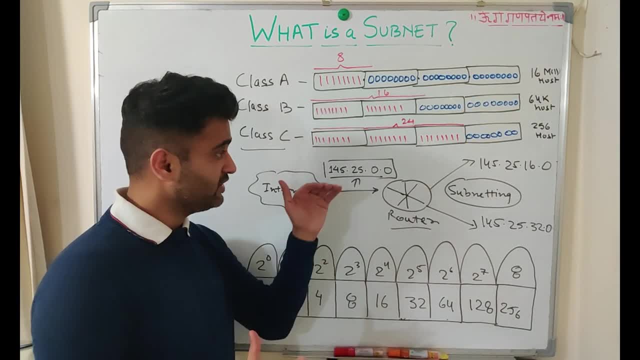 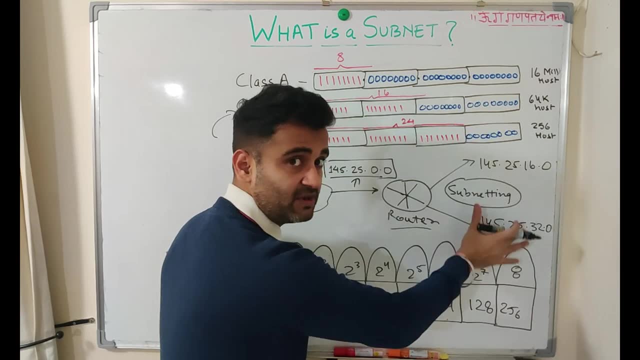 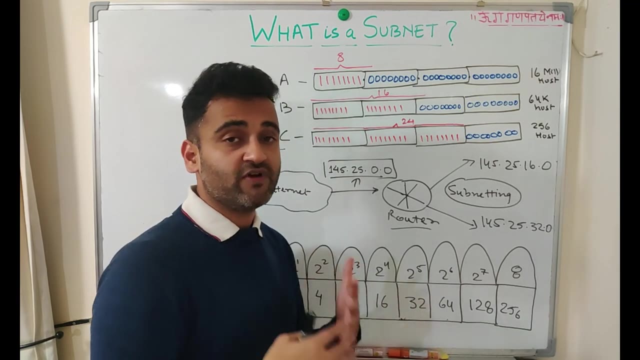 outside world It is still- Uh, It is still the IP address to go into. but internally, this particular IP address has been- you know, has been- facilitating so many different multiple subnets, so that in that way you utilize your network bandwidth very intelligently, and that's why submitting becomes. 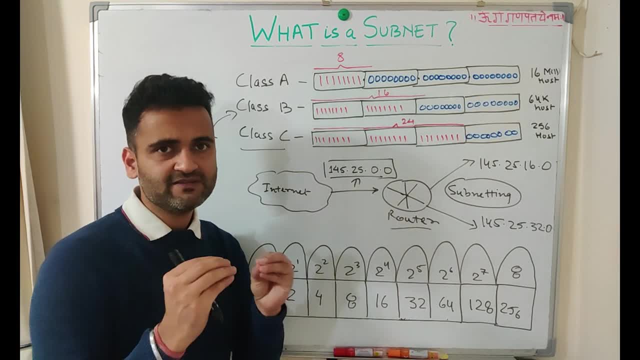 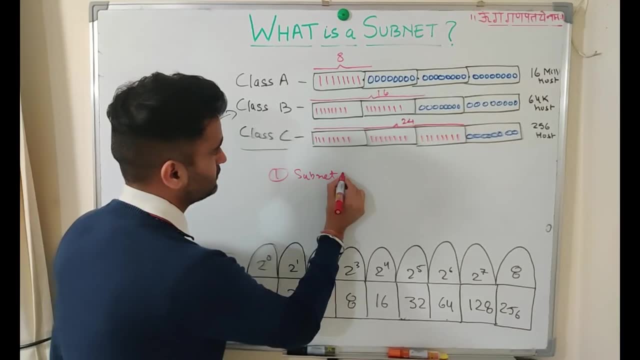 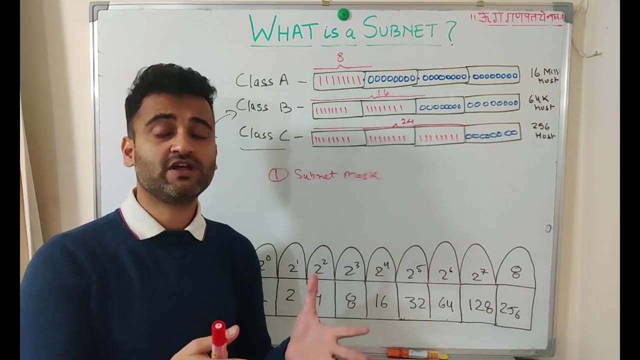 so very important. So now let's understand some basic terminologies which we use and what does exactly it exactly means in the world of submitting, Okay, Okay. So subnet mask is nothing it has. no, it is not an entity to be recognized on the network. 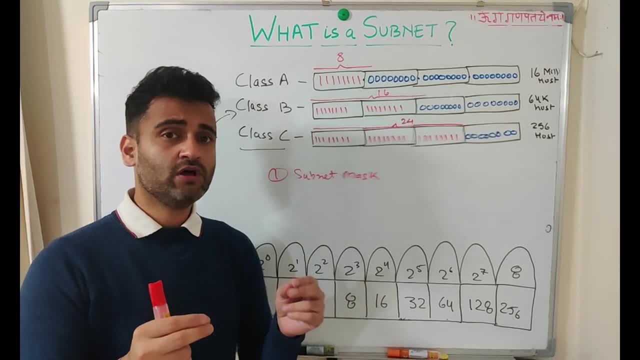 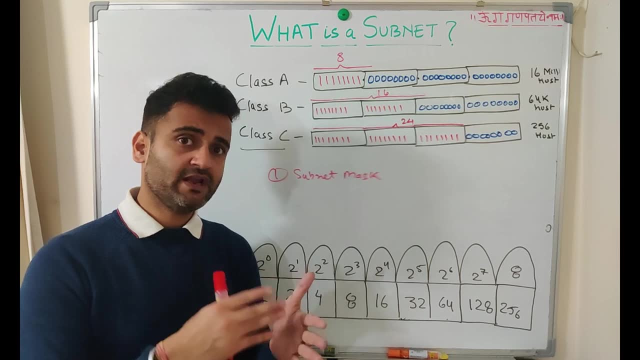 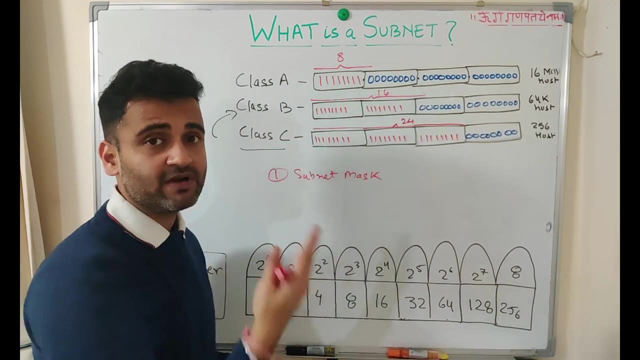 It is a term which is used to denote or to specify in an, in an IP address, how many bits are given to the network and how many are given to the host. So take, for example, your class a IP address. Okay, So what would be the subnet mask for this? 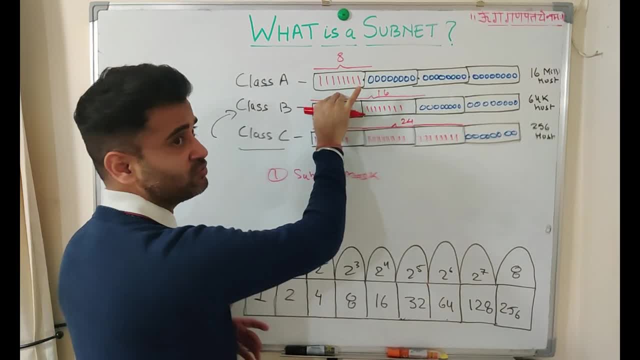 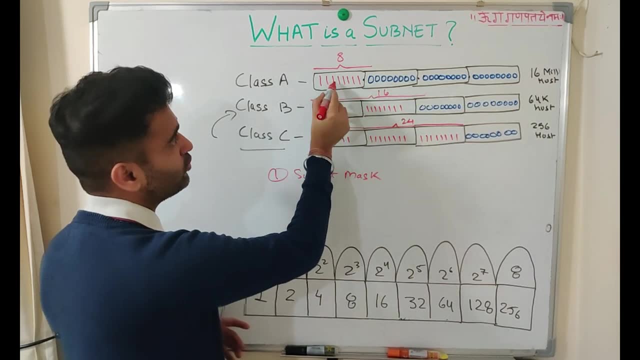 So you have to simply see, you know, the number of bits given to the network. Okay, So how many bits are given to the network? All the eight bits, Okay. All the eight bits means if you add all these eight bits, Okay. 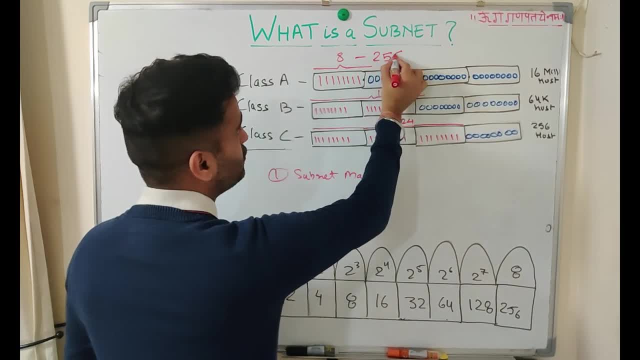 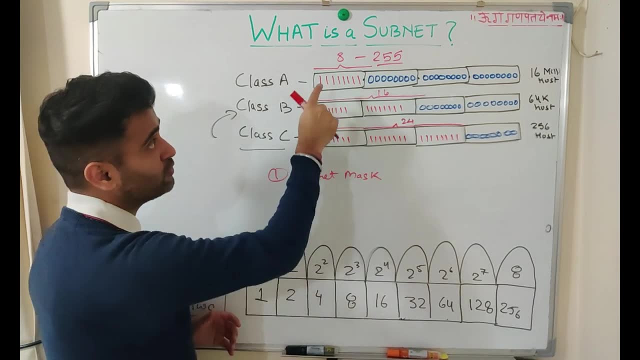 Based on the power of two table, it will come on to 255.. So any octet will not have a maximum value more than 255.. Okay, I've told that in the previous video also. So what would be the subnet mask for this particular IP address? 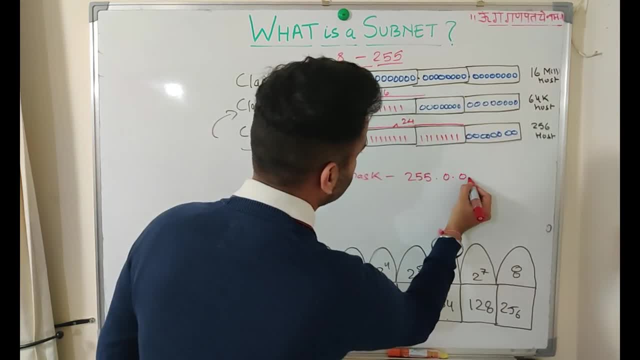 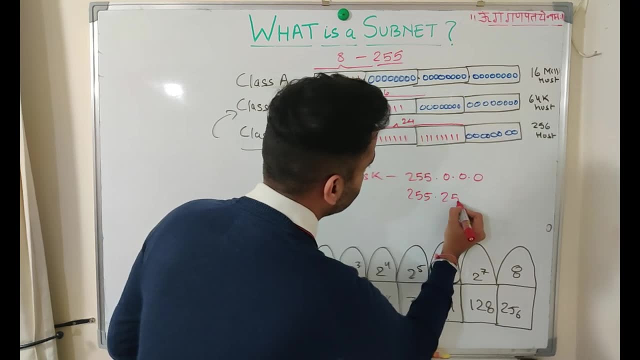 It would be 255.0.0.0.. Okay, Similarly for class B, Okay, Okay, Okay, Similarly for class B, it would be 255.255.0.0 and for class C, it will be 255.255.255.0.. 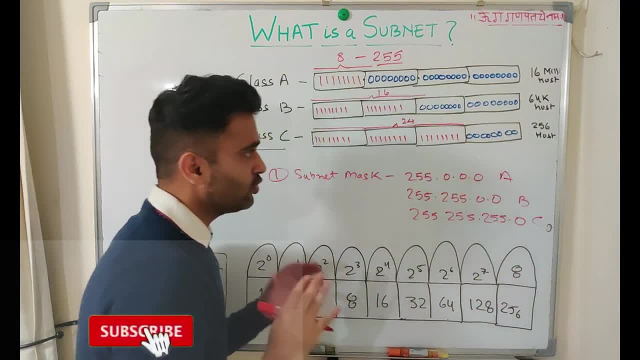 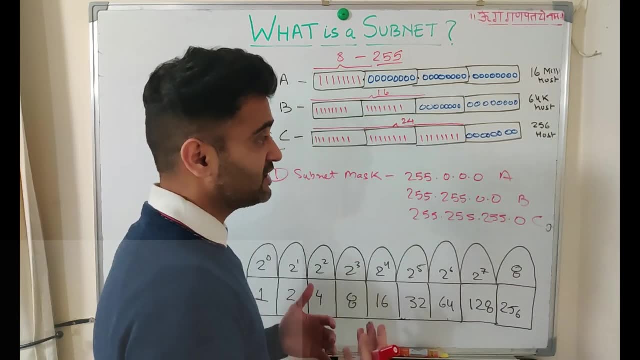 Okay, So it is class A, B and C. So just by looking at your IP address and your subnet mask, you can very clearly identify that which particular bits are given to the network And which are given to the host. So now what we learned about subnetting. 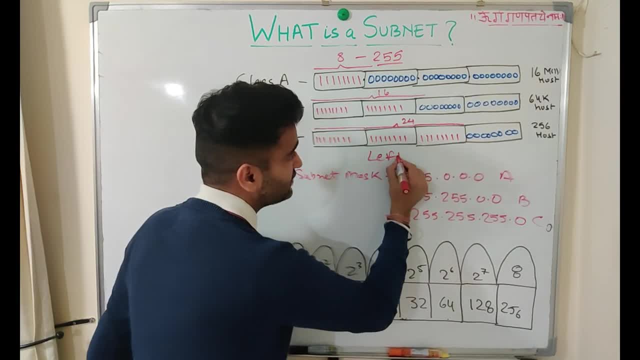 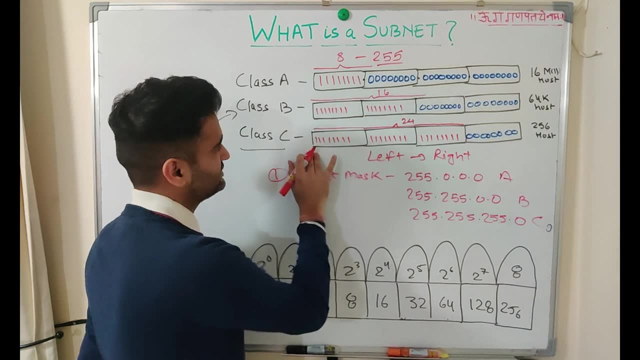 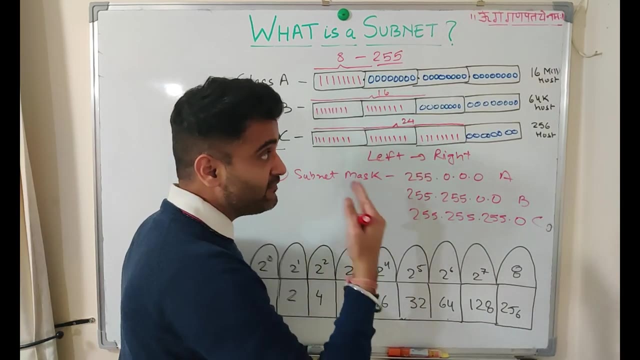 Subnetting is always done from left to right. Okay, So what your network admin will do, suppose? take, for example, this class C IP address: Okay, Now it already has 24 bits given to the network, But when we will do subnetting we will creep into the host bits. 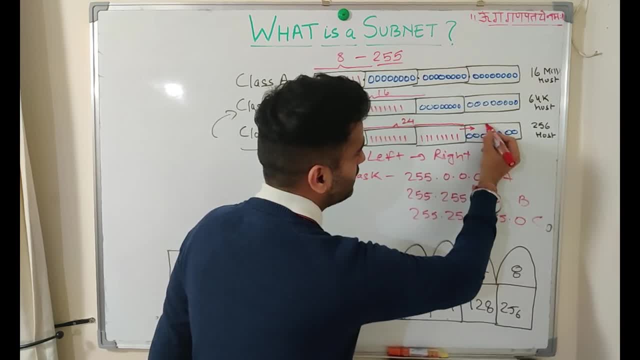 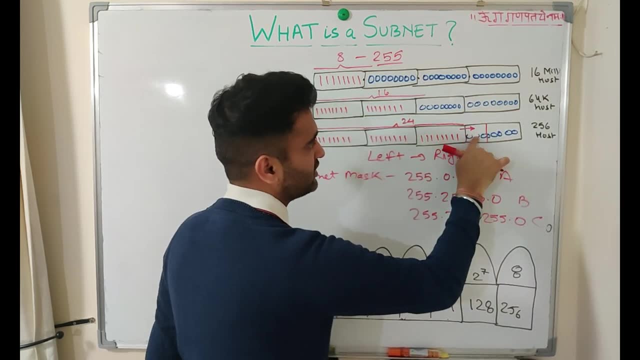 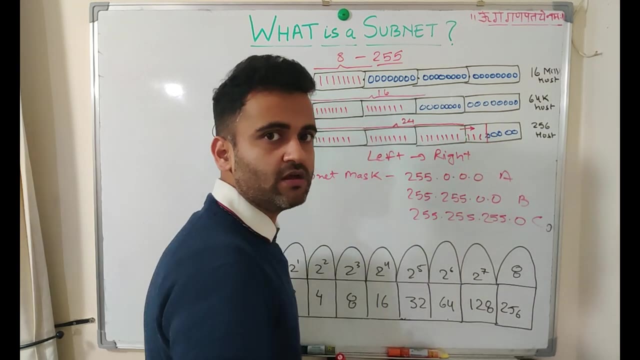 Okay, We will creep into the host bit And maybe take, You know, maybe these many bits. Okay, I am just doing it like this just to make you understand. Okay, So now what has happened? All these will become one, Okay. 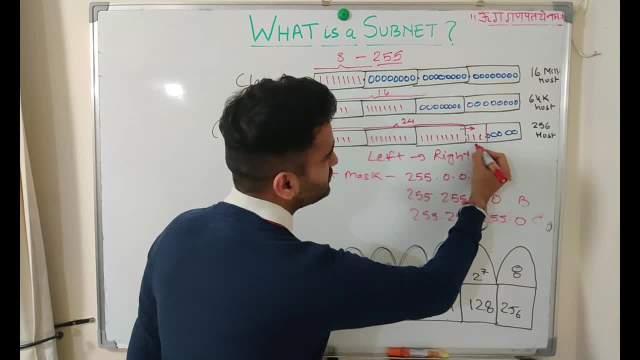 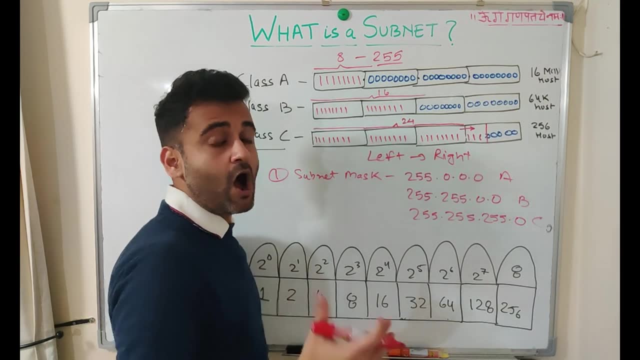 All these will become one. So we already had 24 and we took three bits, Three bits from this particular octet. and how you will take it, It will be based on your subnetting needs, How many subnets you want to create, which we will see with an example. 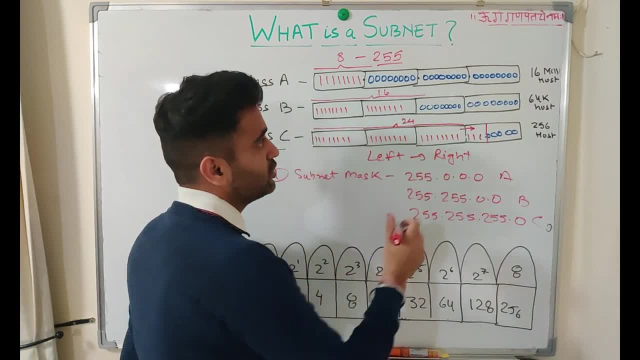 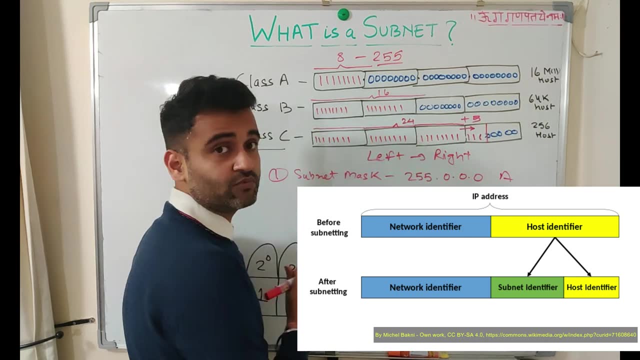 But just understand that. suppose you took three bits from this. So now what happens? 24 plus 3.. So you have now 27 bits, 27 bits given to the network. Okay, So in that case? now what will be your subnet mask? 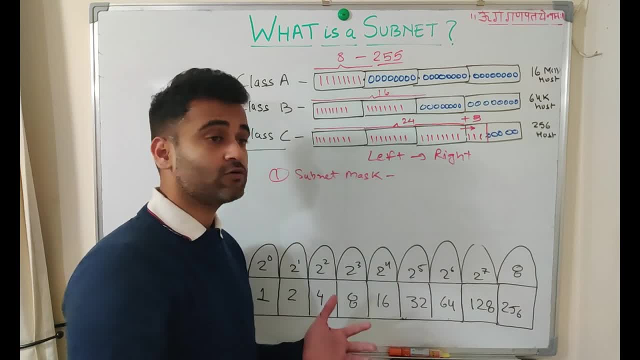 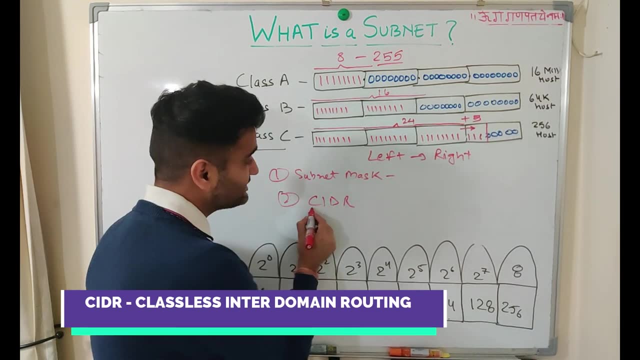 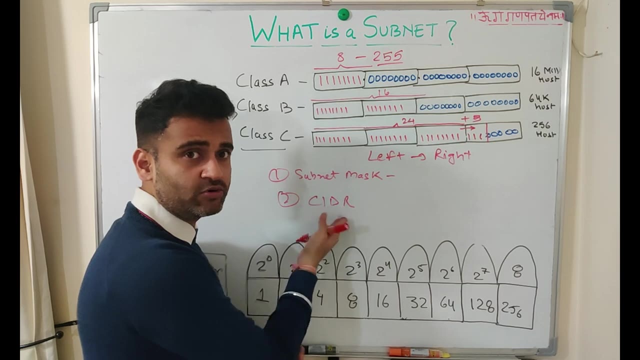 So now, with this concept coming in, another concept comes into picture, which is CIDR range. Okay, What is a CIDR range? CIDR range is classless inter domain routing. That means that, regardless of any class, simply by looking at your CIDR notation you can. 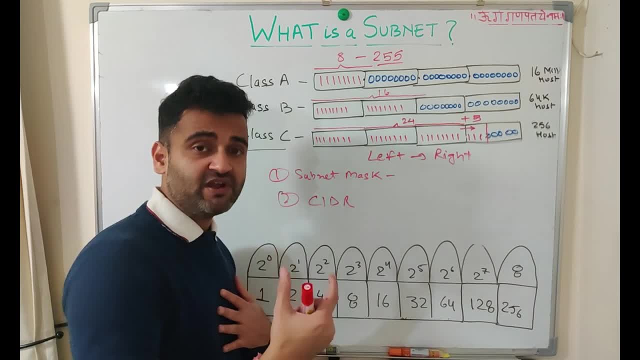 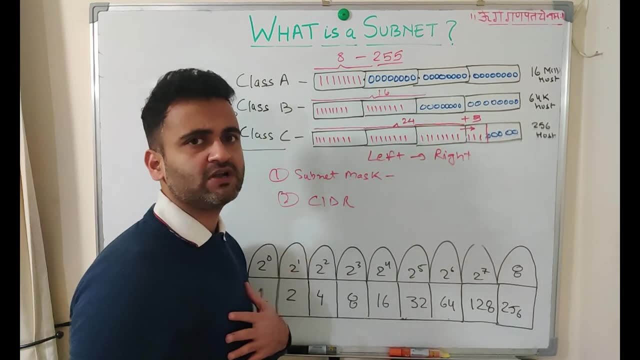 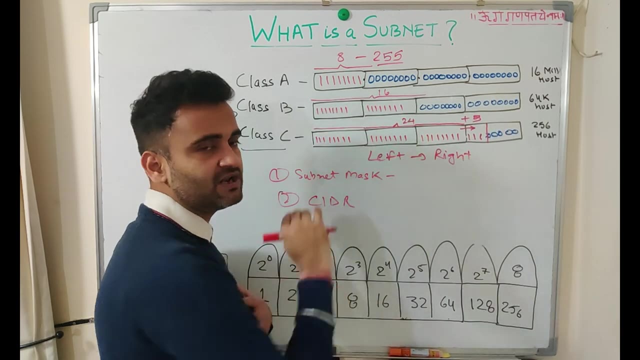 simply identify which bit of your IP address is network and which bit is for host. So suppose in this particular example, Okay, Suppose if we take any particular class C IP address, then it will be denoted by slash notation and then the total number of bits. 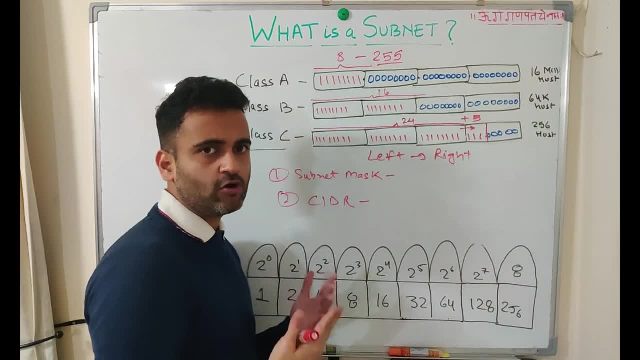 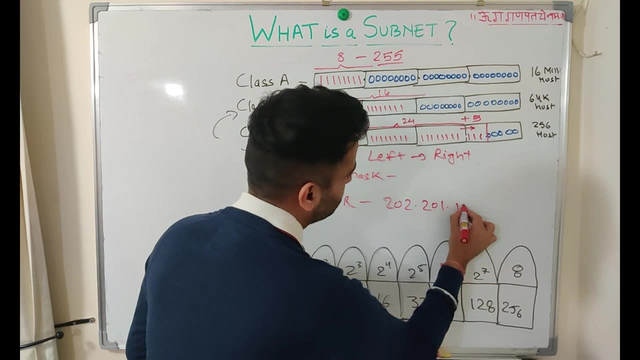 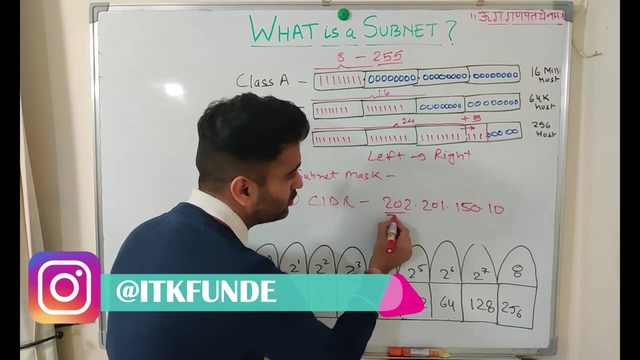 So take, for example, if we take any IP address of class C, So if you take 202.201.150.10.. Okay, So you remember the range Right. So this falls into class C range. In that class C range in the CIDR notation how you will write it. 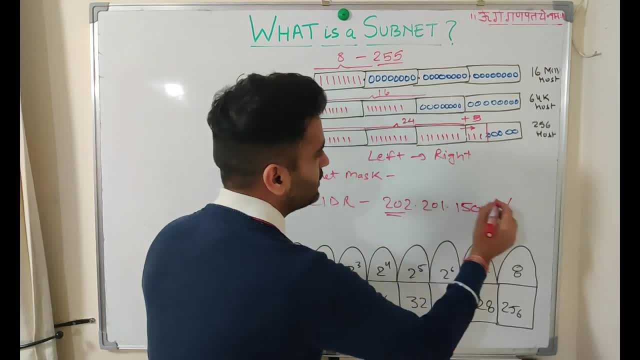 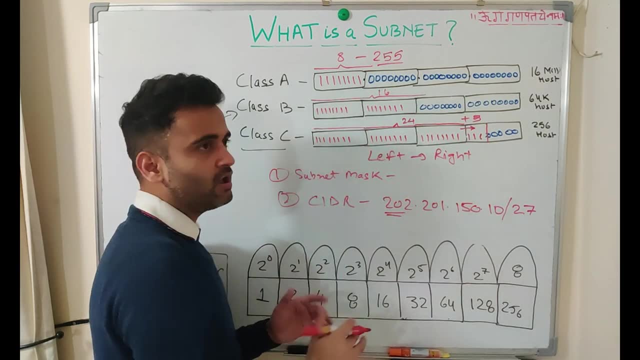 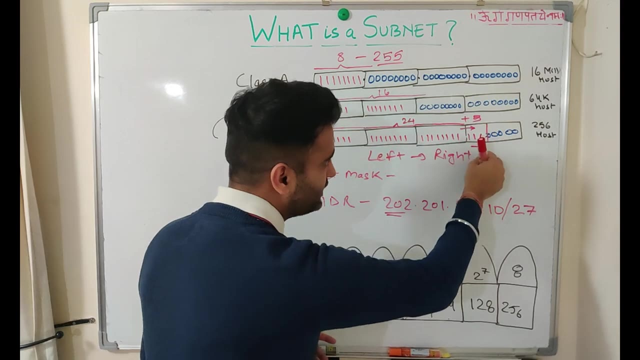 You will simply add a slash and then it will be 27.. You already had 24. by default, class C has 24.. Okay, So you have creeped in. Sorry, I'm using this word, but you are actually taking some bits and doing that utilizing. 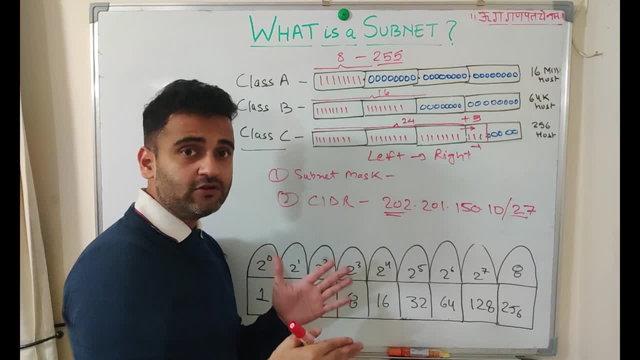 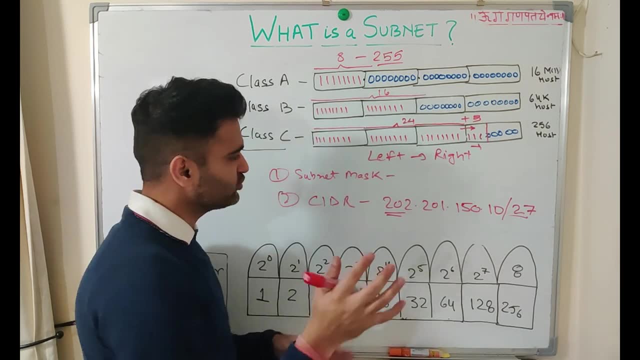 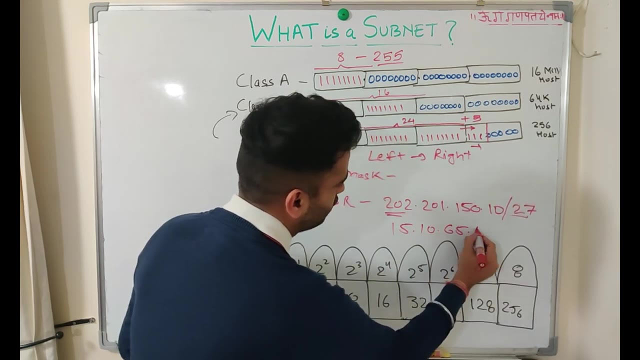 that for the network. So these three bits will get added and then your CIDR notation will be 27.. So, regardless of any class or any IP, Okay, Regardless of any class, suppose if I just take a random IP, Okay, So if I take 15.10.65.40.. 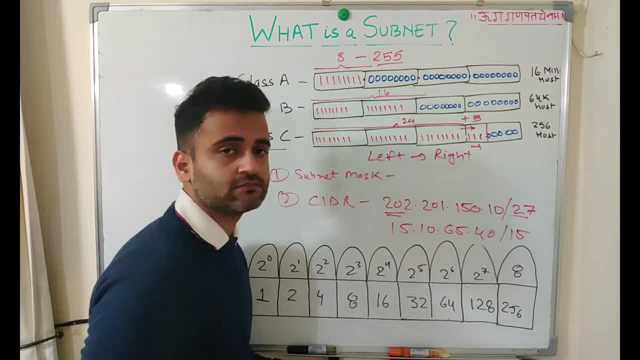 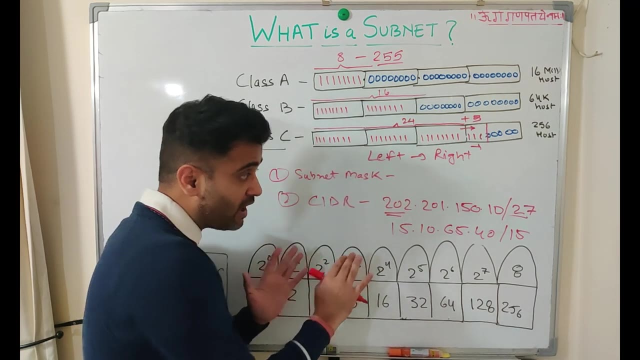 Okay. And if I put slash 15.. Okay, Okay, If I put simply slash 15, that means that for this particular IP address, regardless of its class, 15 bits have been, you know, given to the network. So now I hope you are understanding. and if you now look deep, this is class A IP address. 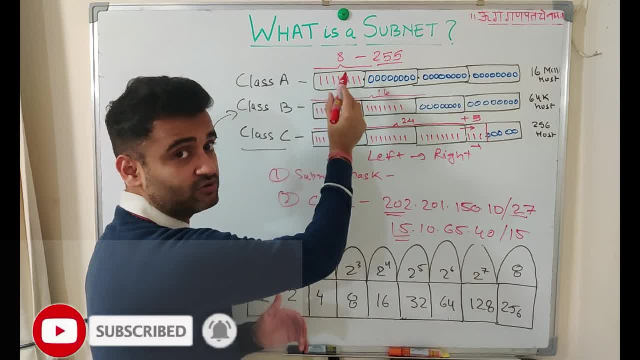 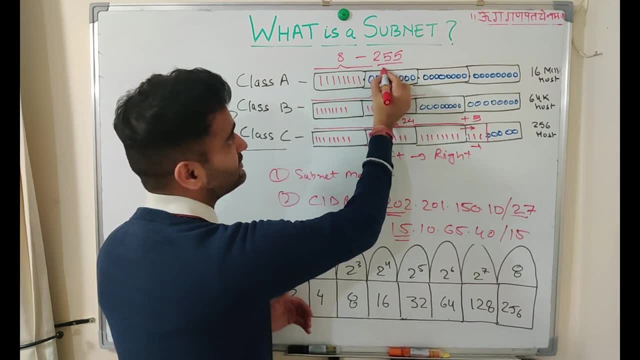 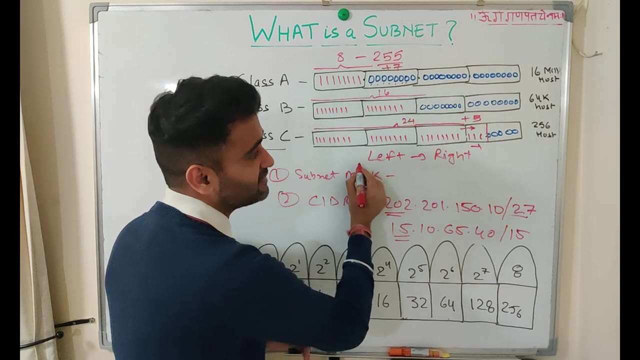 By default, class A has only 8 bits given to the network, but we have given 15 more. That means we have taken 7 bits, 7 bits from here, Okay. So how many? 1, 2, 3, 4, 5, 6, 7- and I always said it is always left to right. 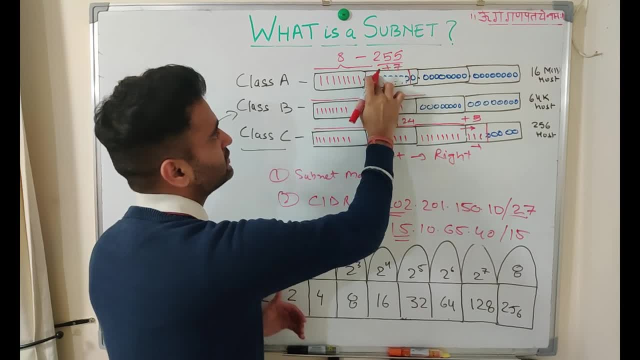 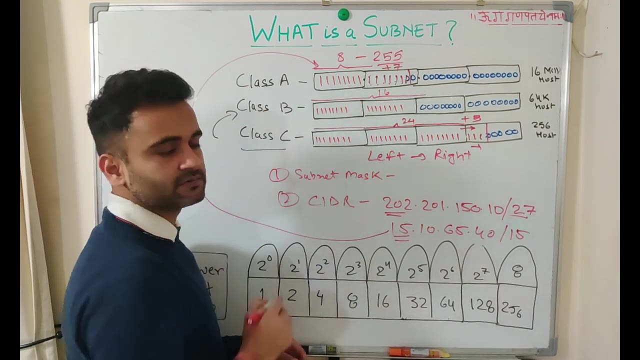 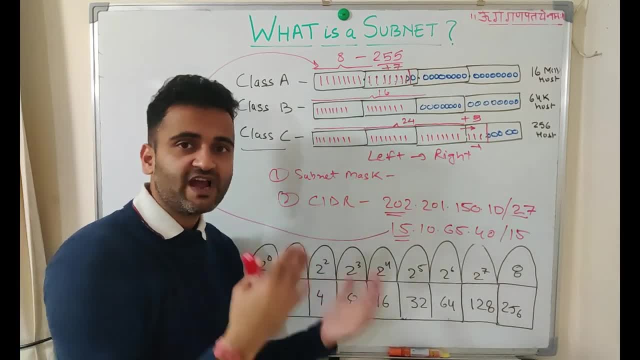 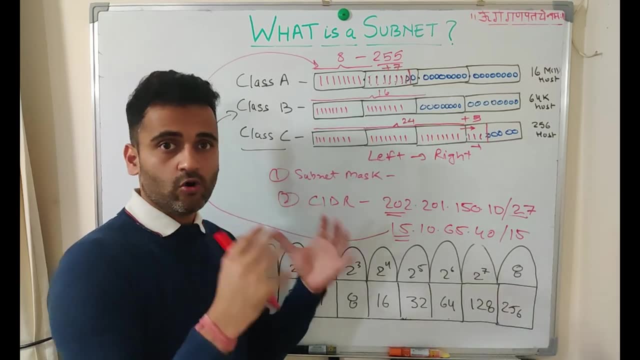 Okay, So this is the way your subnet mask or your CIDR range is helpful to you, Okay, Okay, So your CIDR range is helpful to understand how many bits are given to the network and how many bits are given to the host. 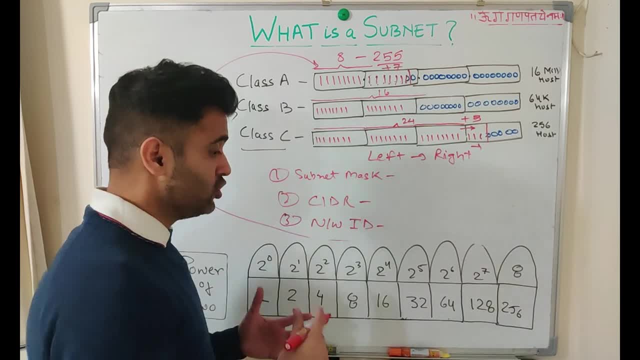 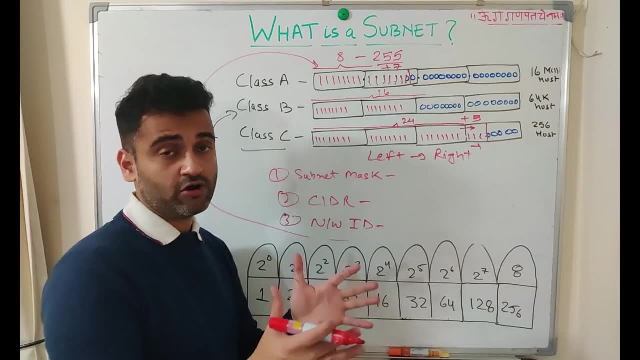 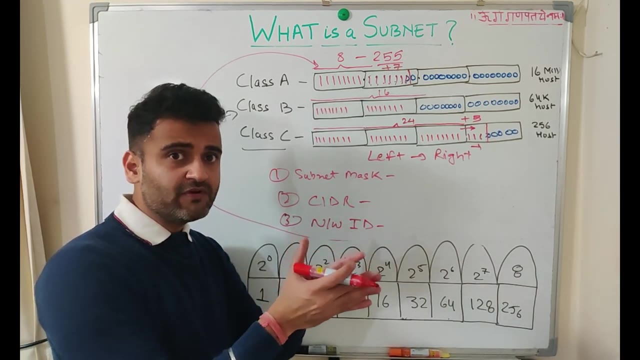 Now the third concept is your network ID. What is a network ID? So every subnet, okay, will always have its first IP, starting IP, as your network IP or network ID. Okay, So suppose, if you divide a network into five different subnetwork, then every subnetwork 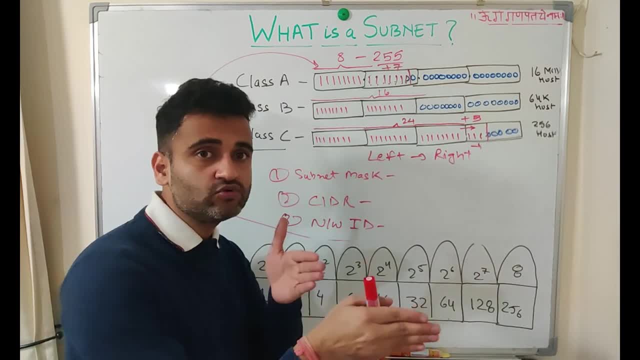 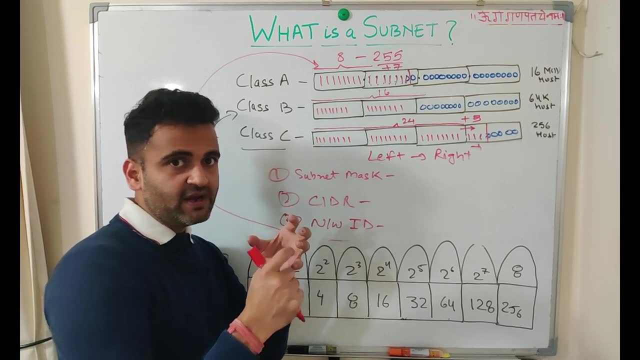 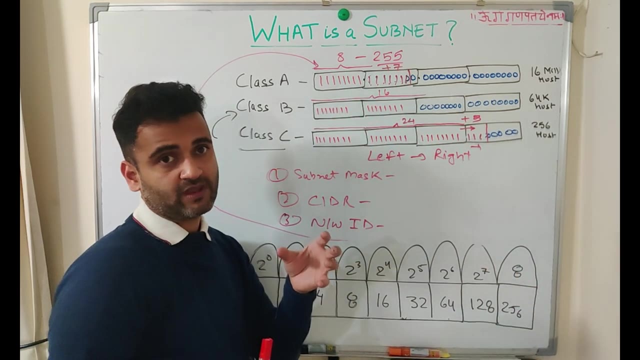 will have a unique network ID with which it will connect to the network. so suppose a router wants to connect to a subnet, then it will remember its network id or it will derive its network id based on the ip address of the device. okay, so that we will see how it. 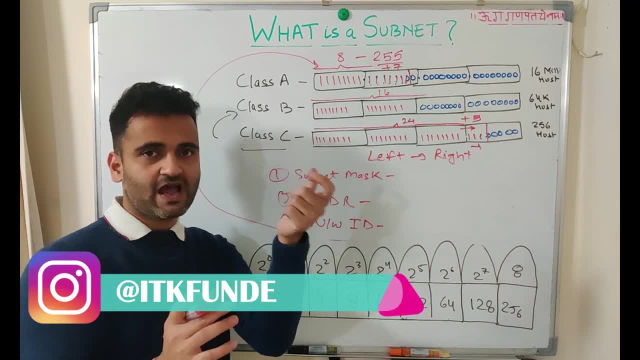 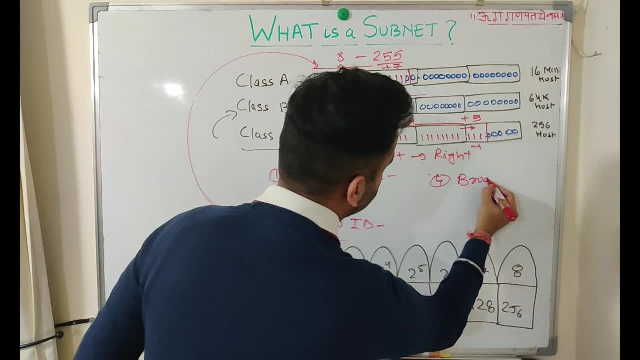 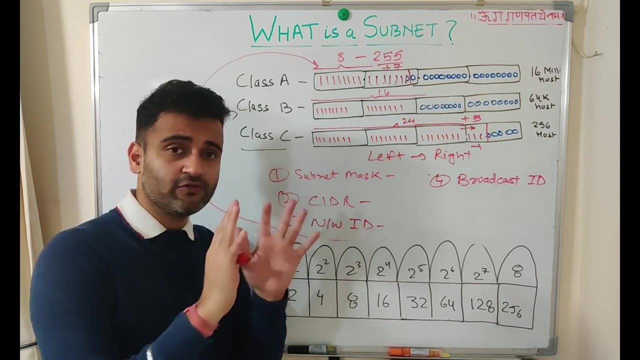 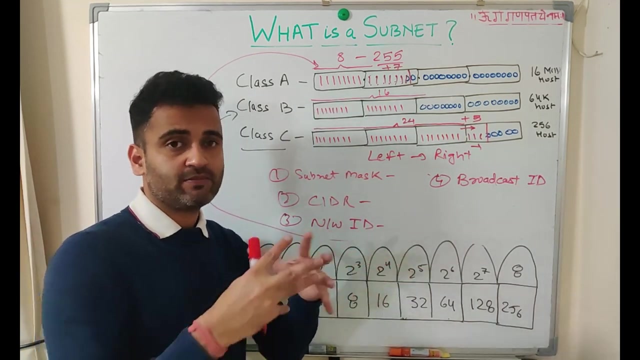 is derived. but just understand that network id is your first id of your subnet range. okay, now the fourth concept is your broadcast id. so your broadcast id is your last id, your last ip address of your subnet range, and this particular broadcast id is utilized to talk to all your hosts within that particular network. okay, so broadcast. 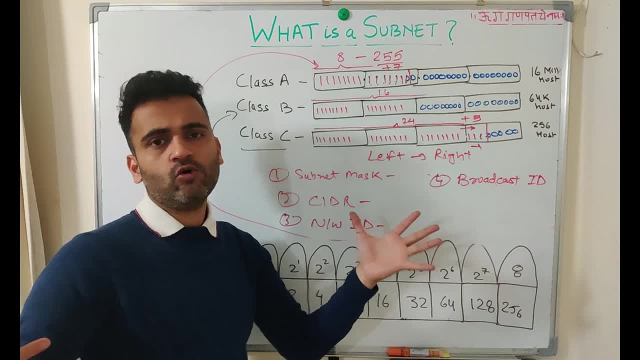 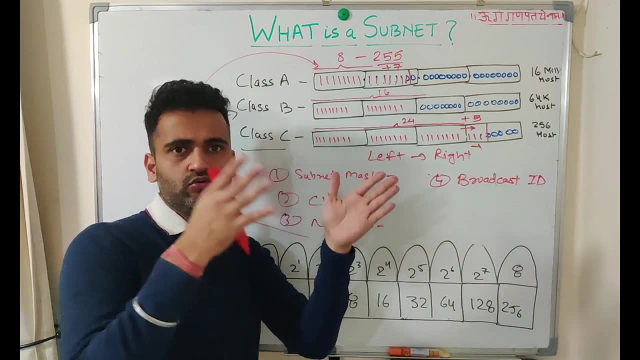 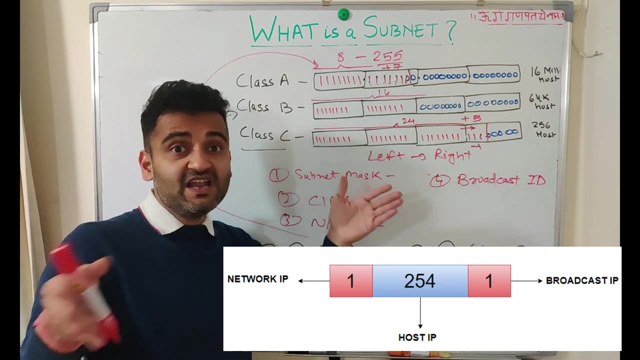 the word broadcast means broadcasting it to an open audience. so suppose, if you have a range from, suppose, just for example, if you have a range of 1 to 10, okay, then 1 would be your network id and 10 would be your broadcast id and in between those 9 would be your actual host. 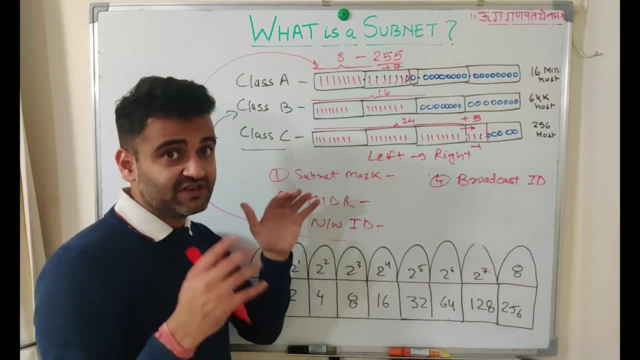 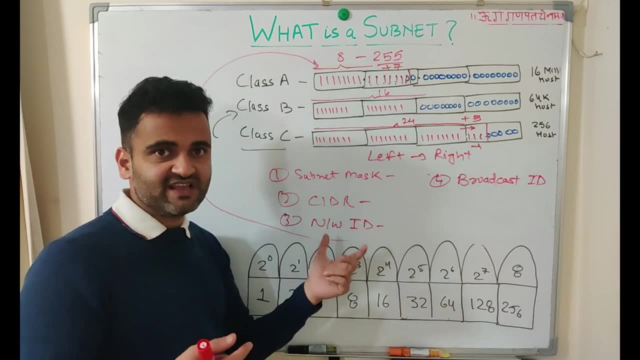 so in this way we have your subnet mask which denotes uh, which particular bits are network and which particular bits are. you know, your uh host cider does the same thing with uh slash notation, which makes it more easy, and then you have your network id and your broadcast. 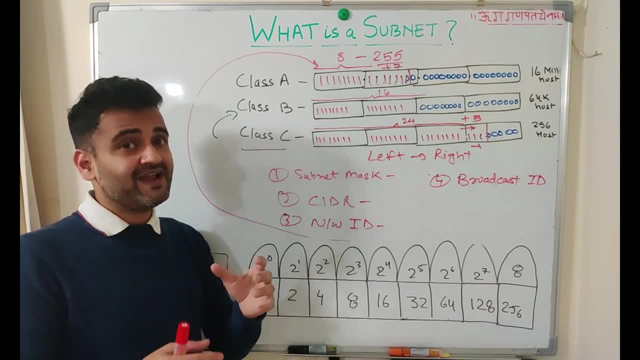 broadcast id. now let's take an example and understand that if we simply have one network id and 10 would be your broadcast id and in between those, 9 would be your actual host. so in this way we have your subnet mask, which denotes which particular bits are network and which particular bits are, you know, your host. cider does the same thing with slash notation, which makes it more easy, and then you have your network id and your broadcast id. now let's take an example and understand that if we simply have one network id and your broadcast id, now let's take an example and understand that if we simply have one, 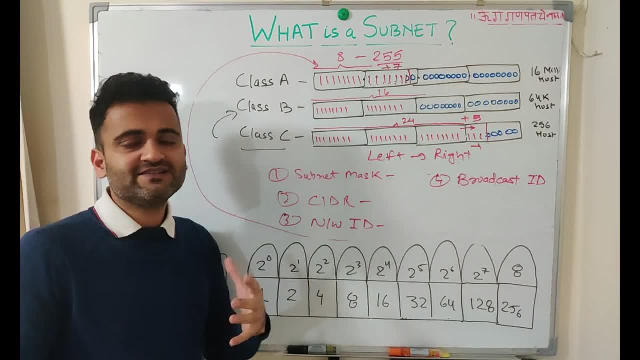 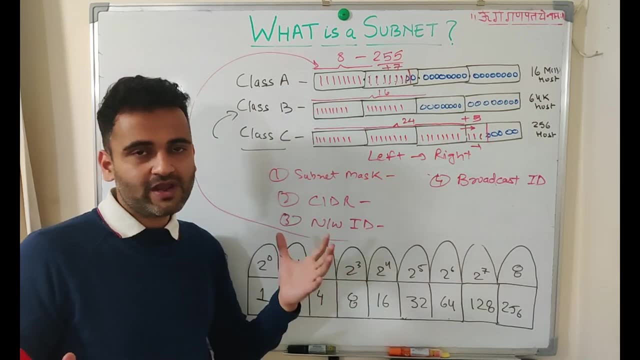 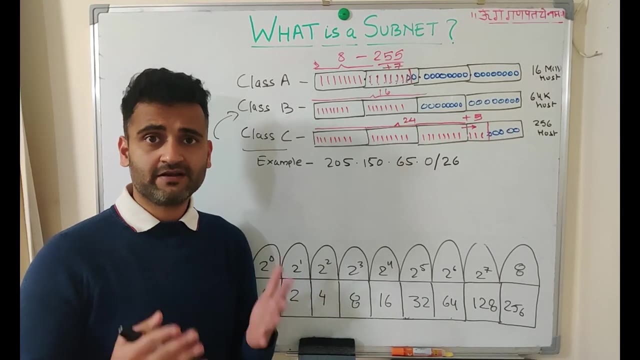 particular ip with a cider range, how we can understand, uh, what is its uh subnet mask, what is its network id, what is its broadcast id? okay, so let's, let's understand that, guys. let's take an example and understand it in more detail. so suppose we have an ip address with 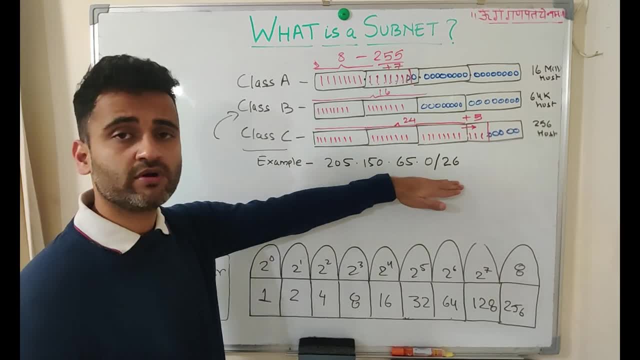 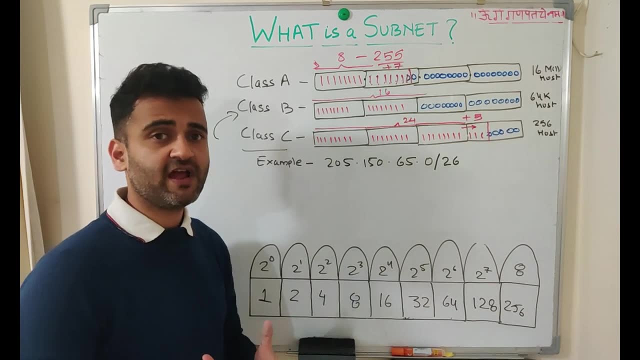 a cider notation: 205.150.65.26. now, this particular: by just by looking at this ip address and this cider notation, we have to identify what will be its subnet mask, what will be its network id, its broadcast id, how many numbers of subnets we can have, how many number of hosts we can. 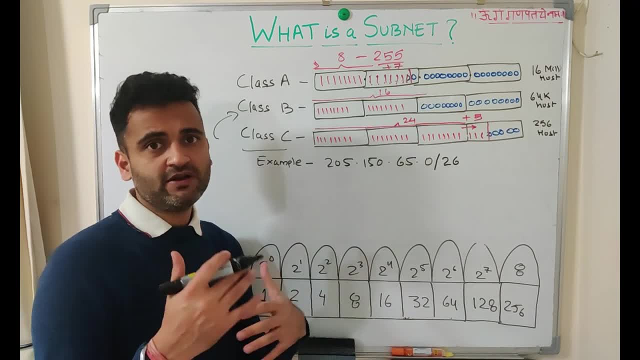 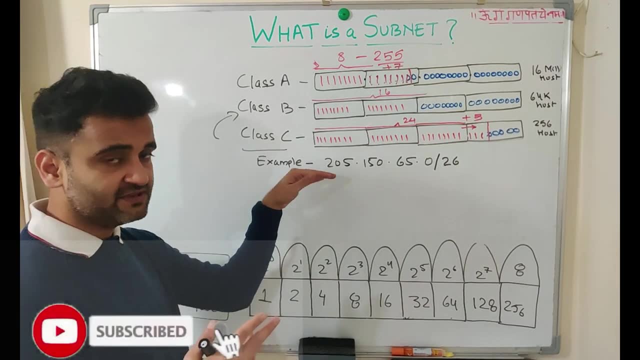 have all these things. so let's take it by example and we'll go step by step, but before that, we have to understand two important formulas, which we will understand with the help of this example. so, first of all, just focus on this whenever you get this kind of a cider notation, just see it is going. 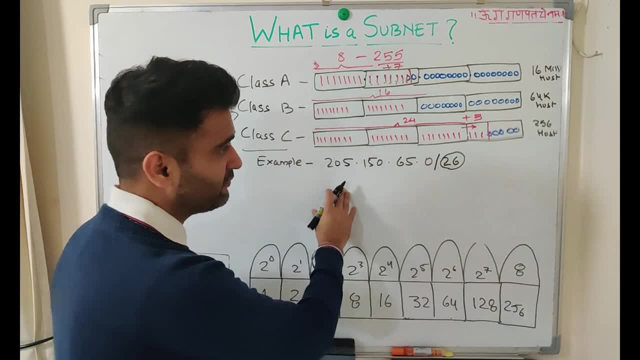 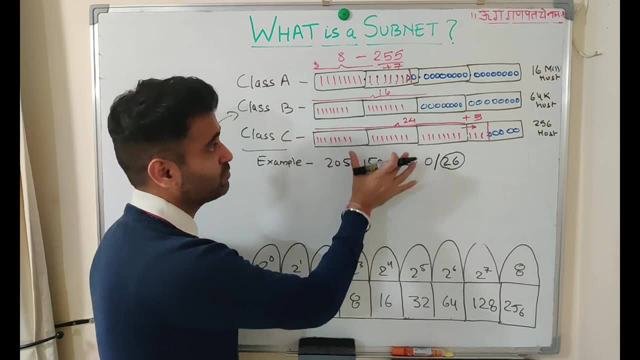 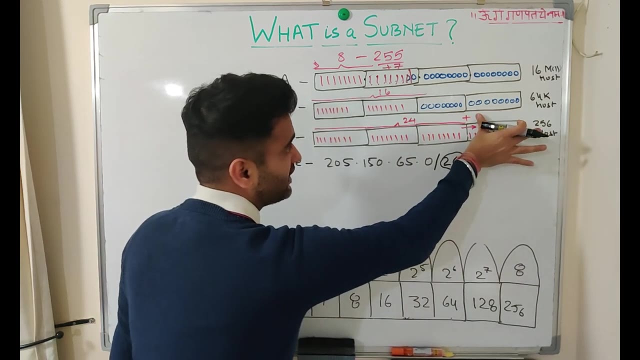 it is 26. so what it is denoting? that by default, you have 32 bits in an IP address. if you see, you know this- this looks like a class C IP address. so by default you have 24 predefined and then after 24 you have two more. so instead of like, just if I have to add it here, so instead, 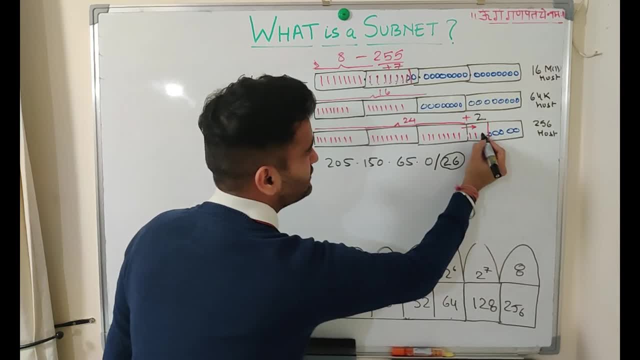 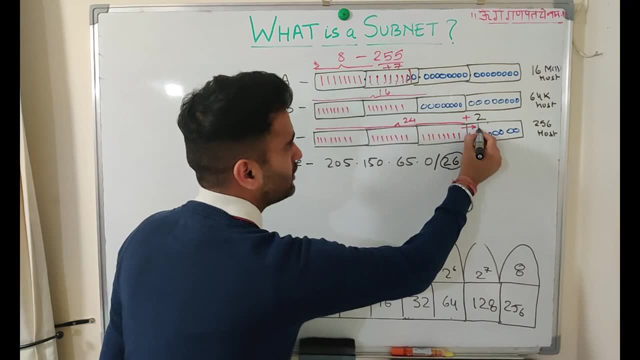 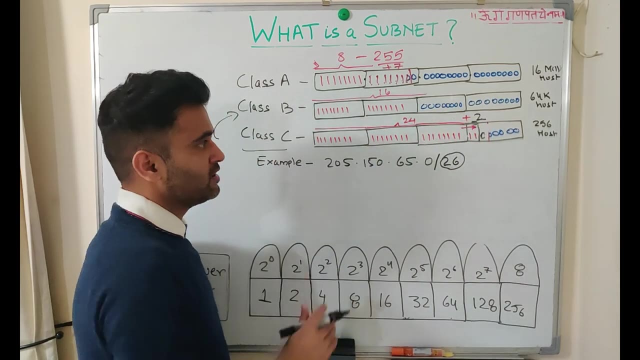 of three, like here, we'll just make it two. okay, and this will become zero. this will be 0, and these two will still be 1. okay, and your network range will be till here. okay. so what you have done? you have increased your network from 24 to 26 bits. now this is this is clear. 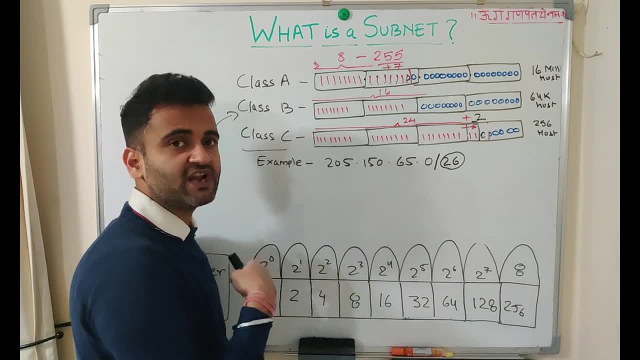 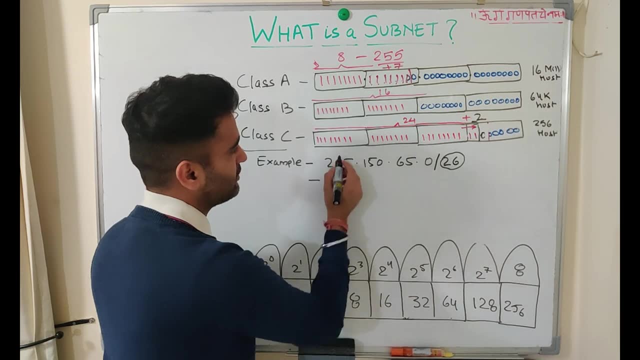 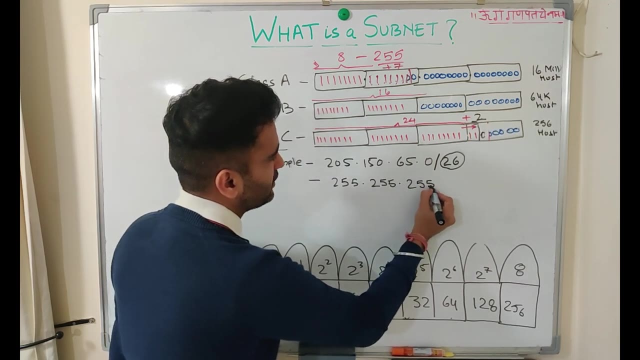 now, based on this, what would be your subnet mask, how you derive your submat mask, so your subnet mask. you already know that by default you have four. Class C: submit mask 255. dot 255. is 15. Now, ideally it is a zero in a normal case, when we have a normal IP range. 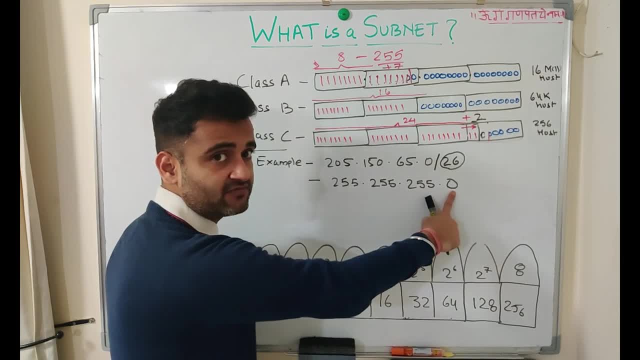 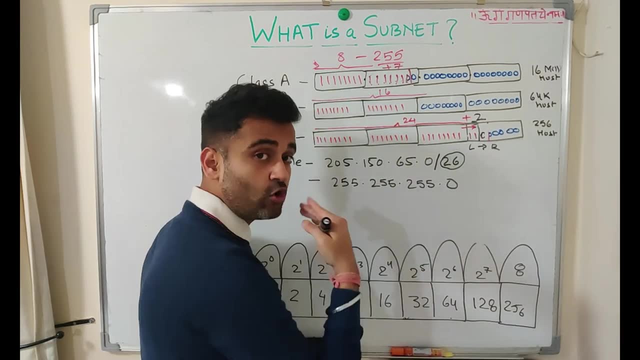 But now we are doing subnetting. So what we are doing, we are borrowing some of the bits from your host octet and giving it to the network. So how many bits we have taken from here? two, So how you will calculate your subnet ID, you have to just add these two bits and see. 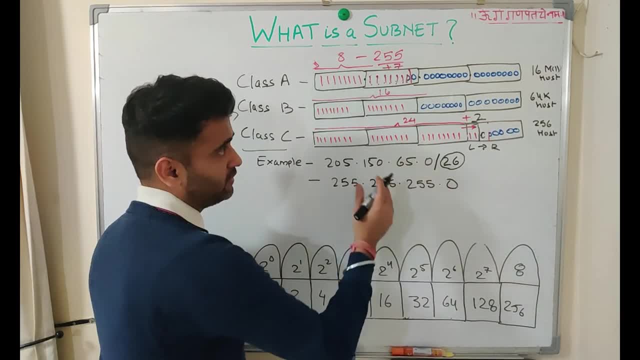 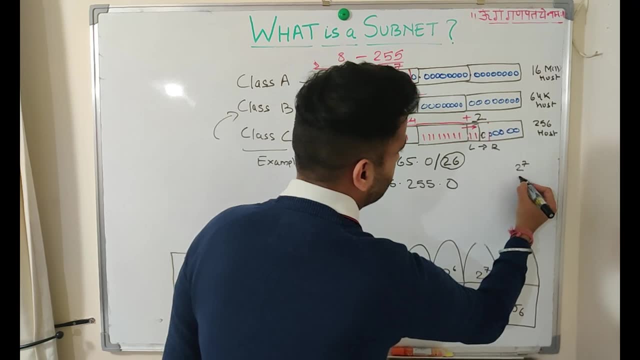 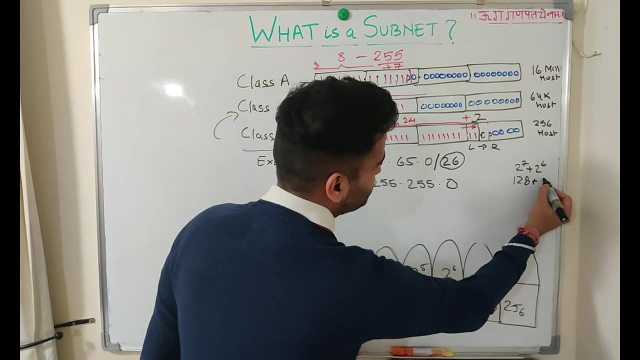 what is the, what is the total? So if you, if you take, you know, the power of two concept into this, then this is two to the power seven and plus the next one is two to the power six, which is 128 plus 64.. 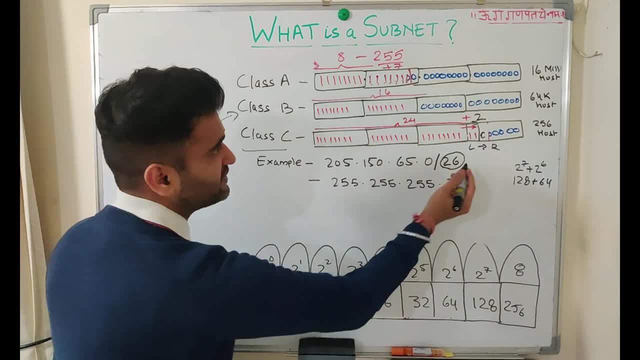 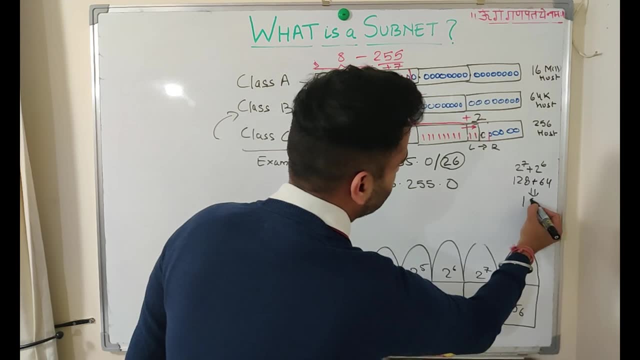 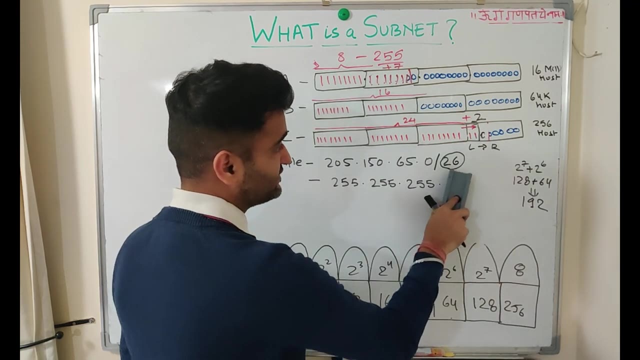 See 128 and 64.. Okay, and always remember it starts with zero: zero one, two, three, four, five, six, seven. So what is the total? Total comes out to be 100.. 192.. So what would be your subnet mask with mine with a slash, 26 sider notation, your subnet. 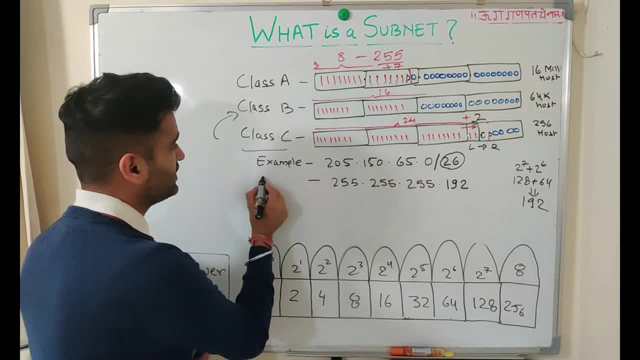 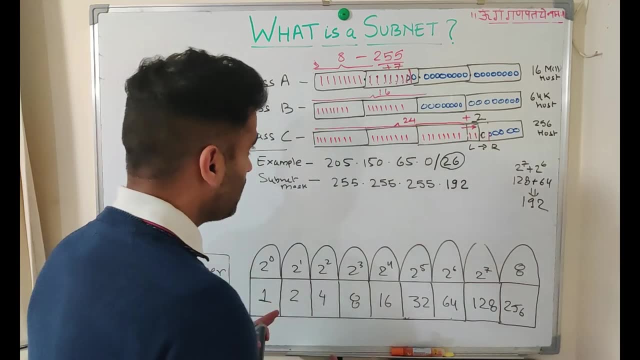 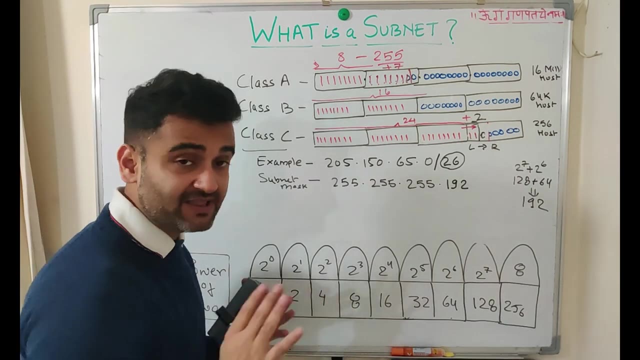 mask will be 192.. This is your subnet mask. Now the next question is: what is your network ID? What is your network ID? Okay, so, for that, there is a binary operation which you have to do, which is called as logical. 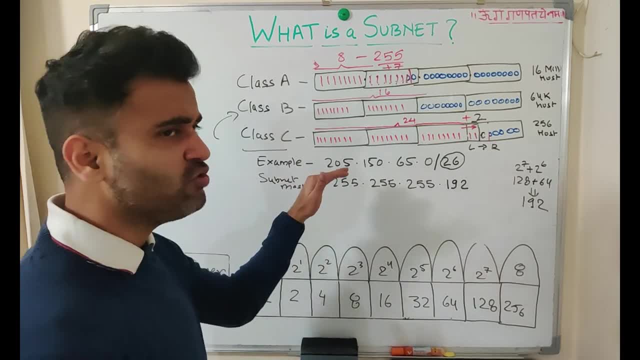 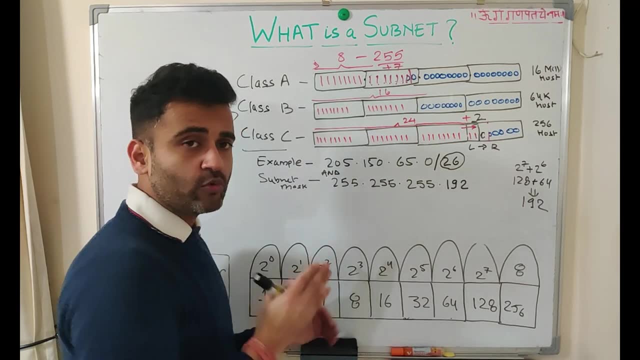 And operation. what is a logical and operation? whenever you have an IP address and when you derive your subnet mask, you have to do an and operation here, So in binary and means. so if you have to take and operation, understand and operation. 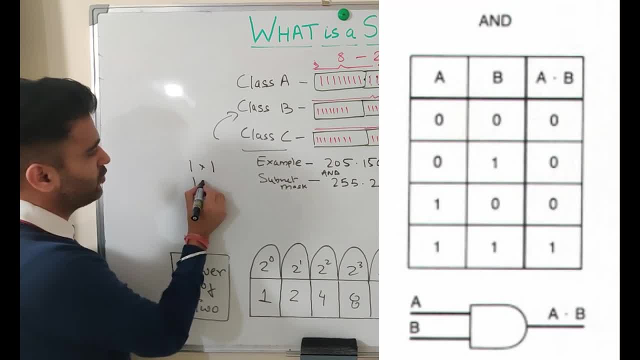 so it is one into one, okay, one into 00 into one, or zero into zero, Okay. these can be the four combinations. So in this case it will be one, Okay, In this case it will be zero. 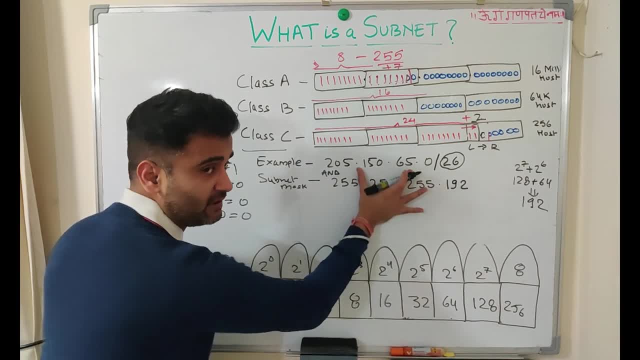 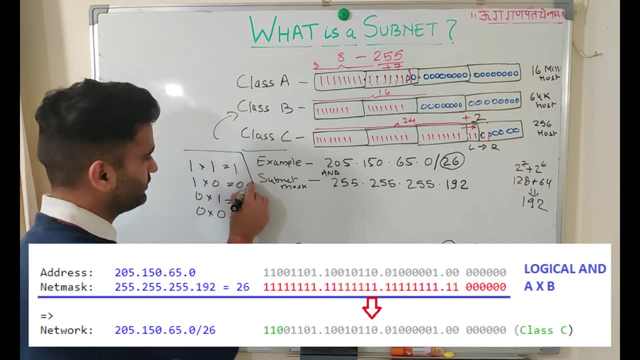 In this case, what you have to do? you have to convert your IP address into binary, And you have to also convert your subnet mask into binary, and then do an and operation Okay, And then, whatever will be the binary output, you will have to calculate it back to decimal. 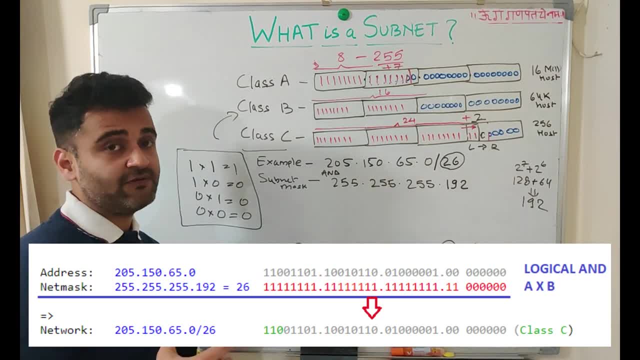 and then that will be your network ID. But it is. it can be very, very difficult task. So a quick, quick thing to do in this case is if you open your Windows laptop, you will have to calculate it back to decimal and then that will be your network ID. 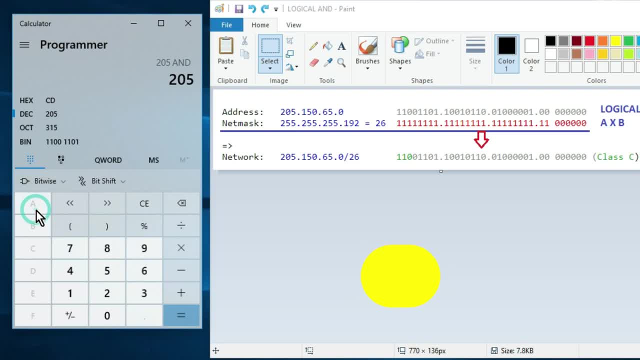 But it is. it can be very, very difficult task. So a quick thing to do in this case is if you open your Windows laptop, you will have to calculate it back to decimal and then that will be your network ID. But it is. it can be very, very difficult task. 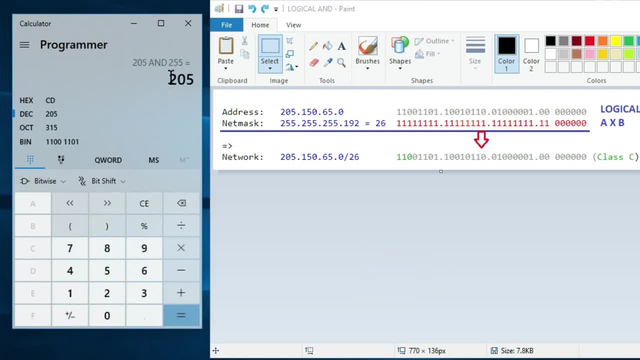 So a quick thing to do in this case is if you open your Windows laptop, you will have to calculate it back to decimal and then that will be your network ID, But it is. it can be very, very difficult task. So a quick thing to do in this case is, if you open your Windows laptop, you will have 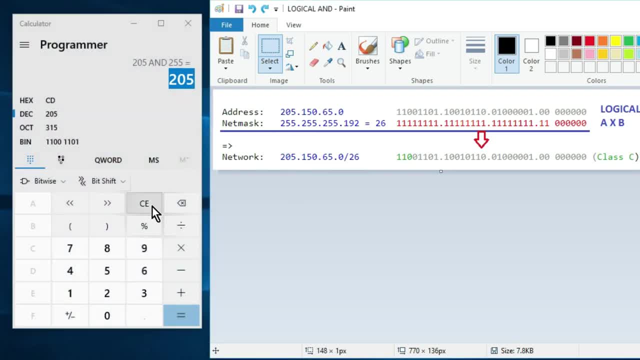 to calculate it back to decimal and then that will be your network ID. But it is. it can be very, very difficult task. So a quick thing to do in this case is, if you open your Windows laptop, you will have to calculate it back to decimal and then that will be your network ID. 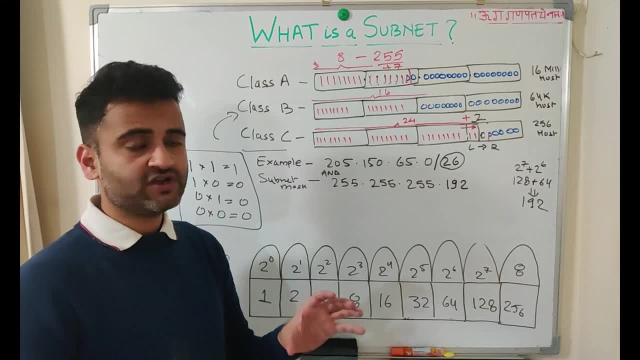 But it is. it can be very, very difficult task. So a quick thing to do in this case is if you open your Windows laptop, you will have to calculate it back to decimal and then that will be your network ID. But it is. it can be very, very difficult task. 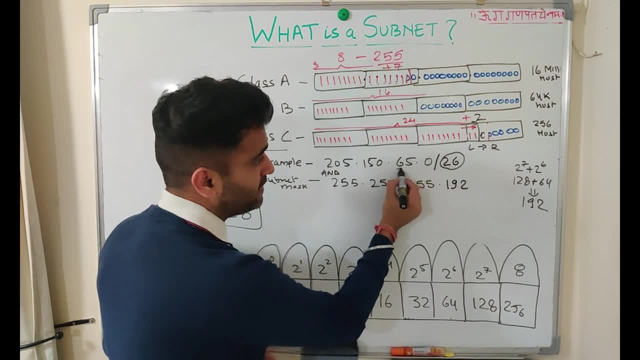 So a quick thing to do in this case is if you open your Windows laptop, you will have to calculate it back to decimal and then that will be your network ID, But it is. it can be very, very difficult task. So a quick thing to do in this case is, if you open your Windows laptop, you will have 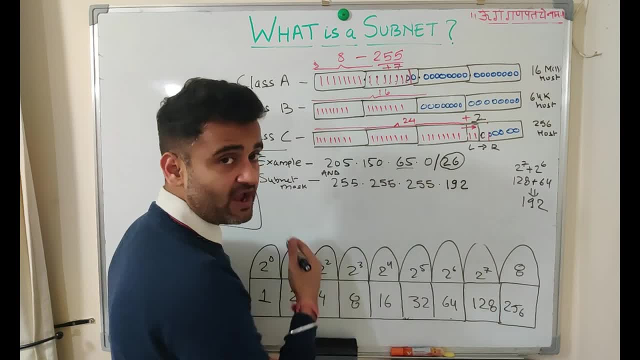 to calculate it back to decimal and then that will be your network ID. But it is. it can be very, very difficult task. So a quick thing to do in this case is, if you open your Windows laptop, you will have to calculate it back to decimal and then that will be your network ID. 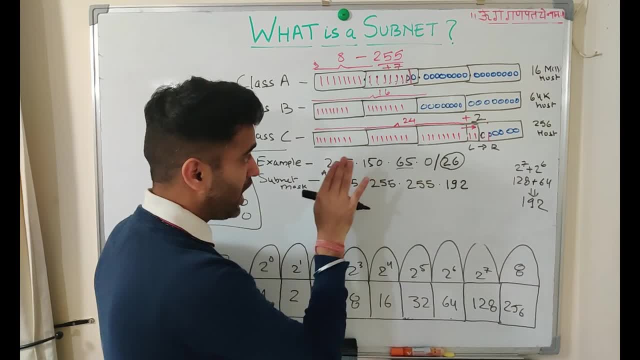 But it is. it can be very, very difficult task. So a quick thing to do in this case is if you open your Windows laptop, you will have to calculate it back to decimal and then that will be your network ID. But it is. it can be very, very difficult task. 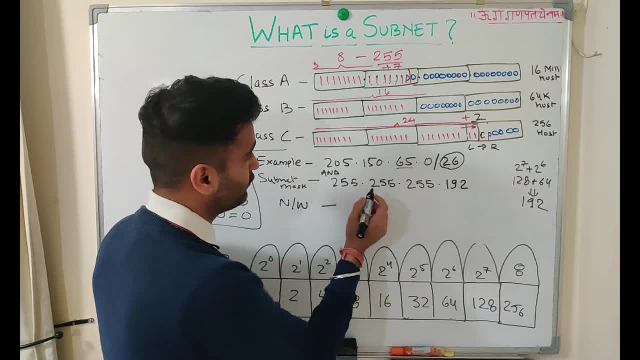 So a quick thing to do in this case is if you open your Windows laptop, you will have to calculate it back to decimal and then that will be your network ID, But it is. it can be very, very difficult task. So a quick thing to do in this case is, if you open your Windows laptop, you will have 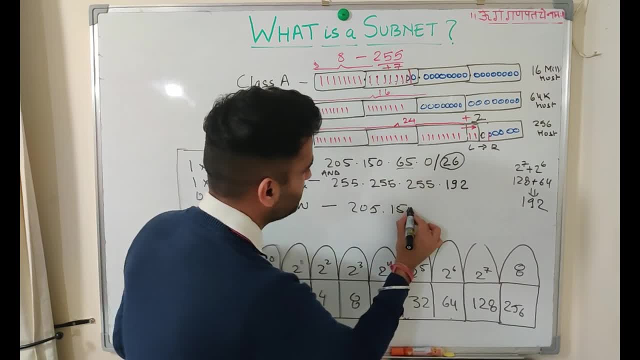 to calculate it back to decimal and then that will be your network ID. But it is. it can be very, very difficult task. So a quick thing to do in this case is, if you open your Windows laptop, you will have to calculate it back to decimal and then that will be your network ID. 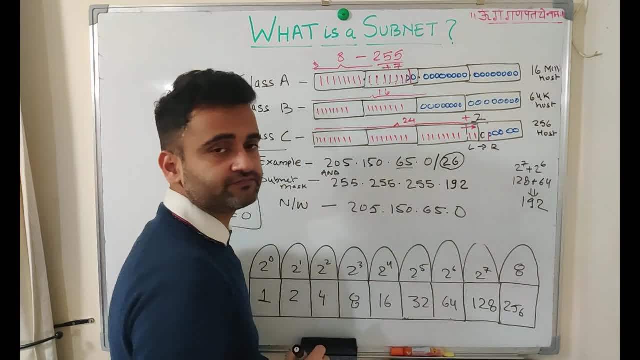 But it is. it can be very, very difficult task. So a quick thing to do in this case is if you open your Windows laptop, you will have to calculate it back to decimal and then that will be your network ID. But it is. it can be very, very difficult task. 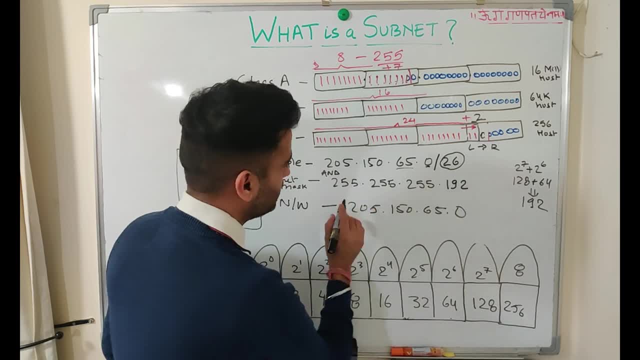 So a quick thing to do in this case is if you open your Windows laptop, you will have to calculate it back to decimal and then that will be your network ID, But it is. it can be very, very difficult task. So a quick thing to do in this case is, if you open your Windows laptop, you will have 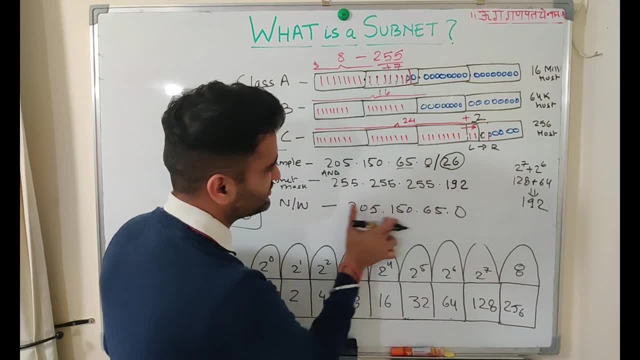 to calculate it back to decimal and then that will be your network ID. But it is. it can be very, very difficult task. So a quick thing to do in this case is, if you open your Windows laptop, you will have to calculate it back to decimal and then that will be your network ID. 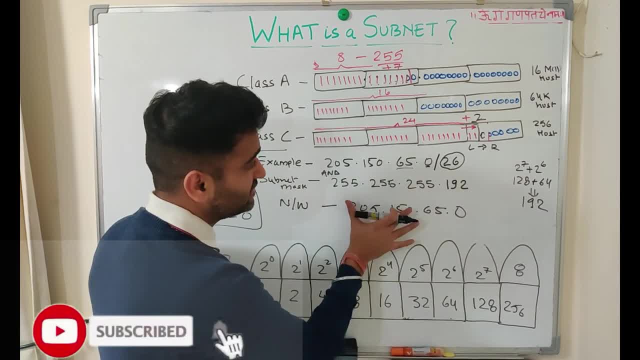 But it is. it can be very, very difficult task. So a quick thing to do in this case is if you open your Windows laptop, you will have to calculate it back to decimal and then that will be your network ID. But it is. it can be very, very difficult task. 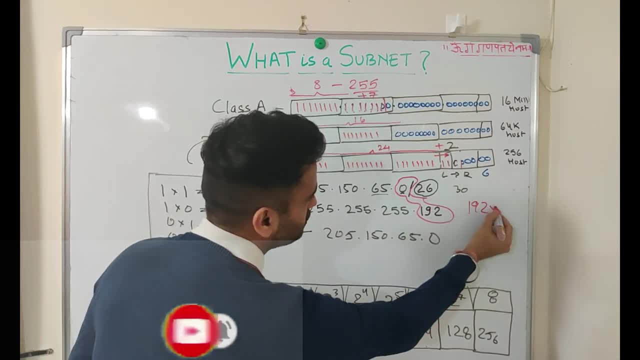 So a quick thing to do in this case is if you open your Windows laptop, you will have to calculate it back to decimal and then that will be your network ID, But it is. it can be very, very difficult task. So a quick thing to do in this case is, if you open your Windows laptop, you will have 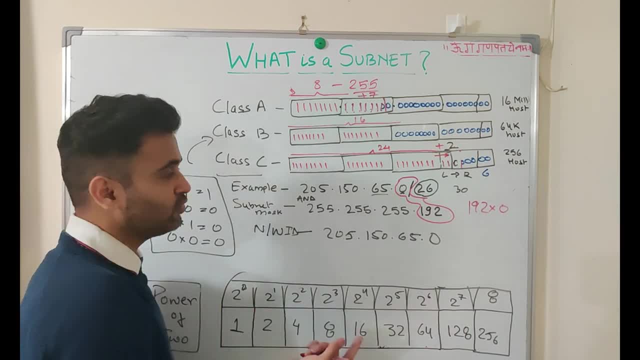 to calculate it back to decimal and then that will be your network ID. But it is. it can be very, very difficult task. So a quick thing to do in this case is, if you open your Windows laptop, you will have to calculate it back to decimal and then that will be your network ID. 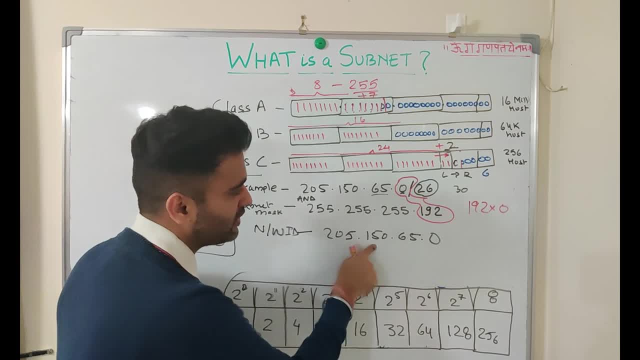 But it is. it can be very, very difficult task. So a quick thing to do in this case is if you open your Windows laptop, you will have to calculate it back to decimal and then that will be your network ID. But it is. it can be very, very difficult task. 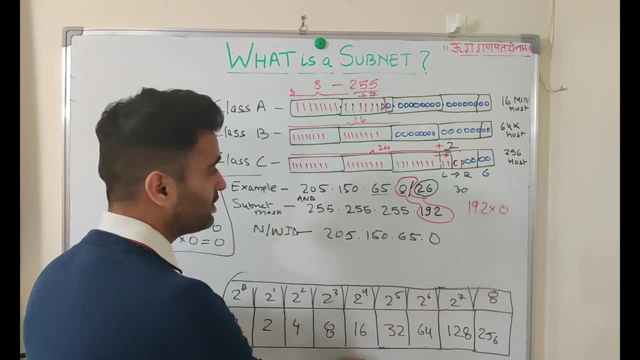 So a quick thing to do in this case is if you open your Windows laptop, you will have to calculate it back to decimal and then that will be your network ID, But it is. it can be very, very difficult task. So a quick thing to do in this case is, if you open your Windows laptop, you will have 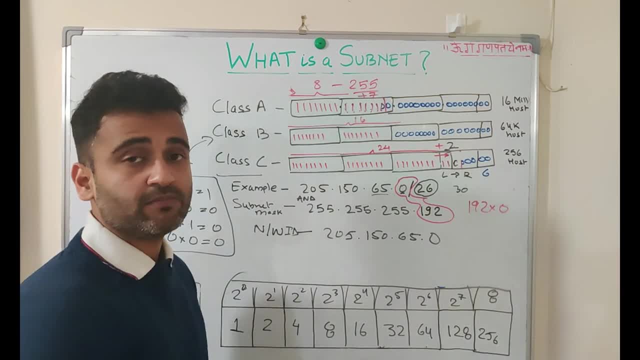 to calculate it back to decimal and then that will be your network ID. But it is. it can be very, very difficult task. So a quick thing to do in this case is, if you open your Windows laptop, you will have to calculate it back to decimal and then that will be your network ID. 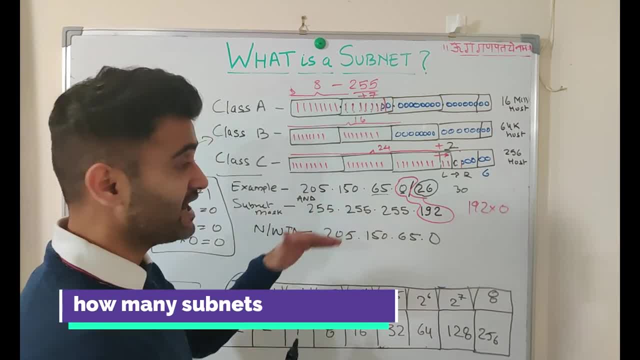 But it is. it can be very, very difficult task. So a quick thing to do in this case is if you open your Windows laptop, you will have to calculate it back to decimal and then that will be your network ID. But it is. it can be very, very difficult task. 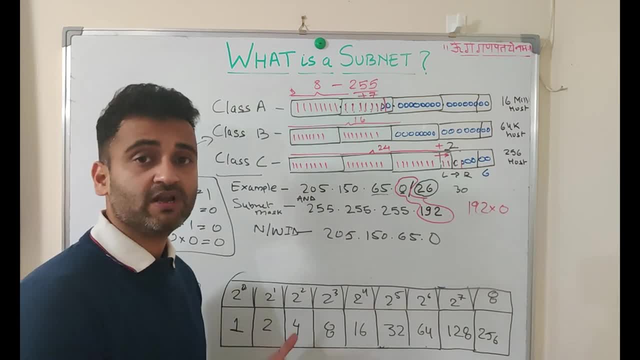 So a quick thing to do in this case is if you open your Windows laptop, you will have to calculate it back to decimal and then that will be your network ID, But it is. it can be very, very difficult task. So a quick thing to do in this case is, if you open your Windows laptop, you will have 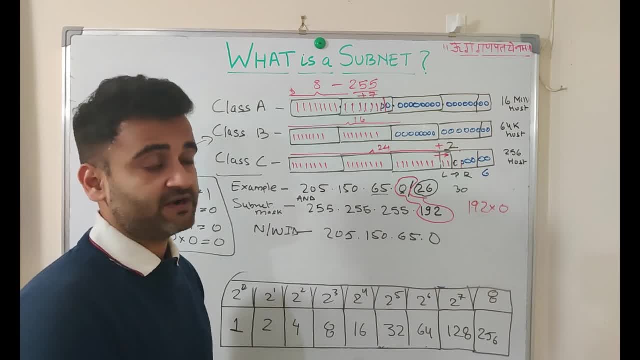 to calculate it back to decimal and then that will be your network ID. But it is. it can be very, very difficult task. So a quick thing to do in this case is, if you open your Windows laptop, you will have to calculate it back to decimal and then that will be your network ID. 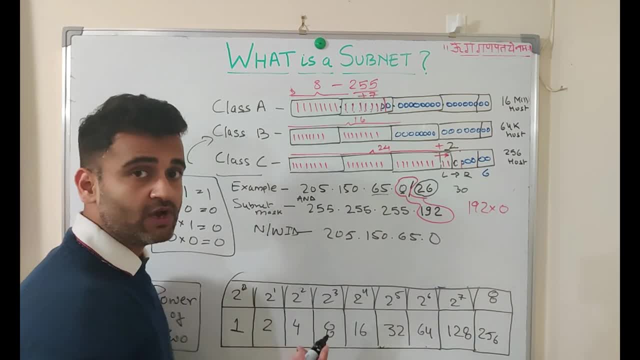 But it is. it can be very, very difficult task. So a quick thing to do in this case is if you open your Windows laptop, you will have to calculate it back to decimal and then that will be your network ID. But it is. it can be very, very difficult task. 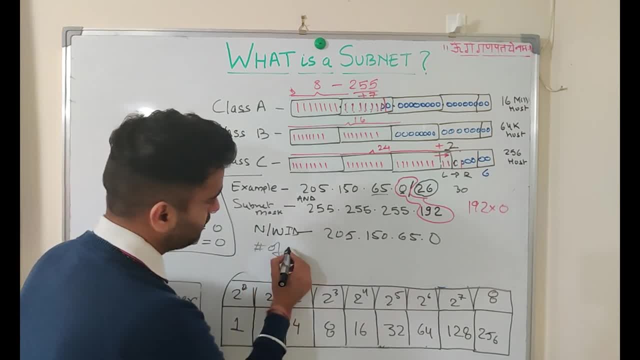 So a quick thing to do in this case is if you open your Windows laptop, you will have to calculate it back to decimal and then that will be your network ID, But it is. it can be very, very difficult task. So a quick thing to do in this case is, if you open your Windows laptop, you will have 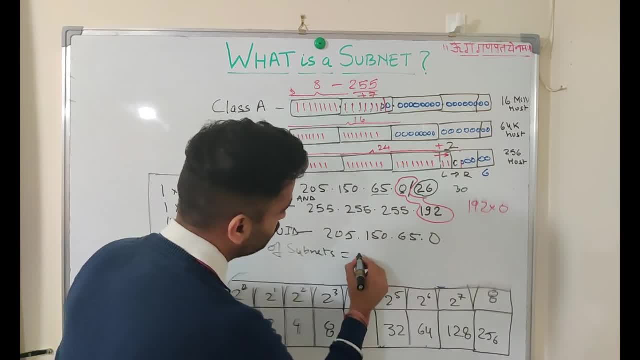 to calculate it back to decimal and then that will be your network ID. But it is. it can be very, very difficult task. So a quick thing to do in this case is, if you open your Windows laptop, you will have to calculate it back to decimal and then that will be your network ID. 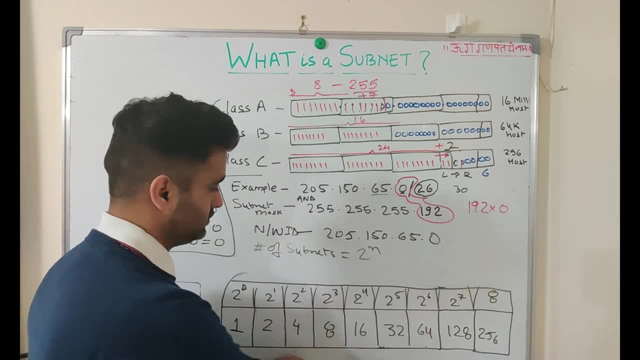 But it is. it can be very, very difficult task. So a quick thing to do in this case is if you open your Windows laptop, you will have to calculate it back to decimal and then that will be your network ID. But it is. it can be very, very difficult task. 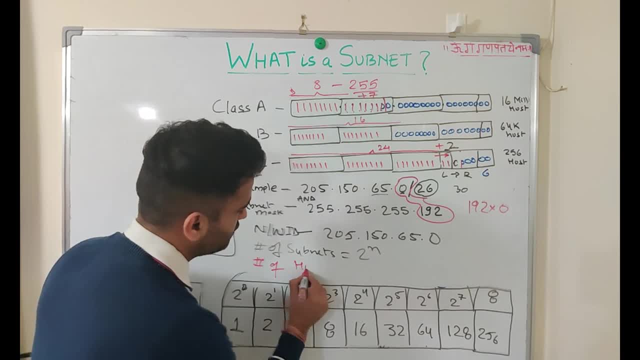 So a quick thing to do in this case is if you open your Windows laptop, you will have to calculate it back to decimal and then that will be your network ID, But it is. it can be very, very difficult task. So a quick thing to do in this case is, if you open your Windows laptop, you will have 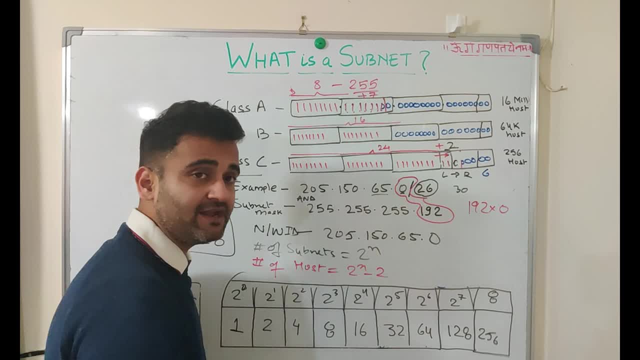 to calculate it back to decimal and then that will be your network ID. But it is. it can be very, very difficult task. So a quick thing to do in this case is, if you open your Windows laptop, you will have to calculate it back to decimal and then that will be your network ID. 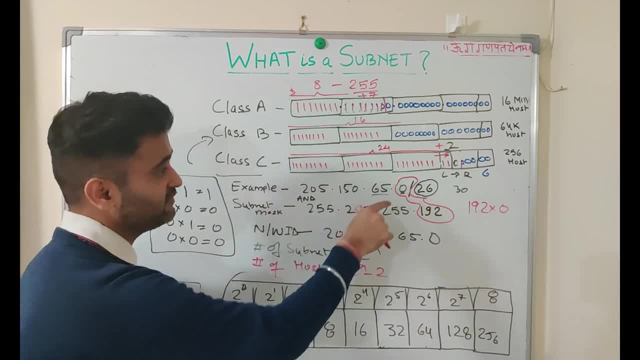 But it is. it can be very, very difficult task. So a quick thing to do in this case is if you open your Windows laptop, you will have to calculate it back to decimal and then that will be your network ID. But it is. it can be very, very difficult task. 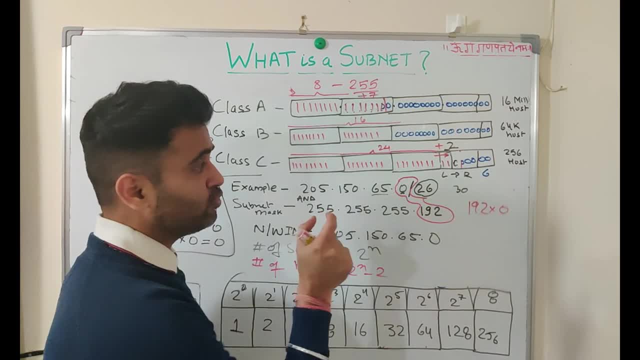 So a quick thing to do in this case is if you open your Windows laptop, you will have to calculate it back to decimal and then that will be your network ID, But it is. it can be very, very difficult task. So a quick thing to do in this case is, if you open your Windows laptop, you will have 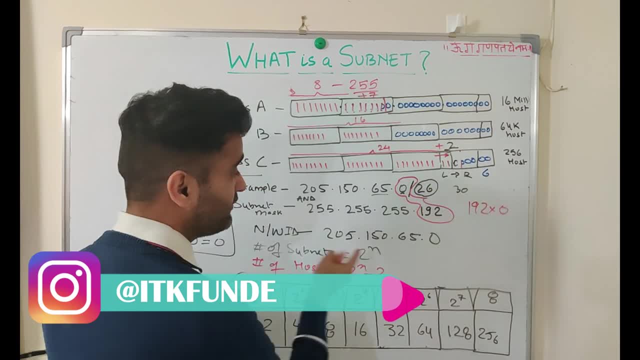 to calculate it back to decimal and then that will be your network ID. But it is. it can be very, very difficult task. So a quick thing to do in this case is, if you open your Windows laptop, you will have to calculate it back to decimal and then that will be your network ID. 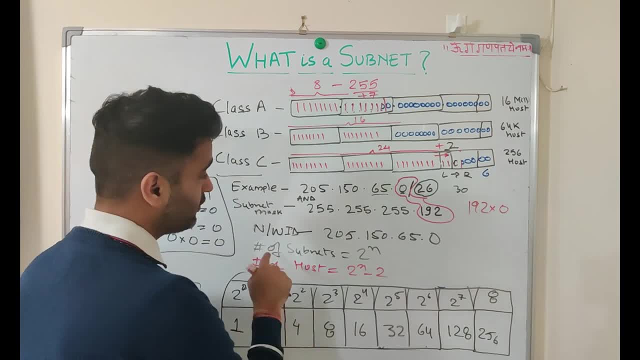 But it is. it can be very, very difficult task. So a quick thing to do in this case is if you open your Windows laptop, you will have to calculate it back to decimal and then that will be your network ID. But it is. it can be very, very difficult task. 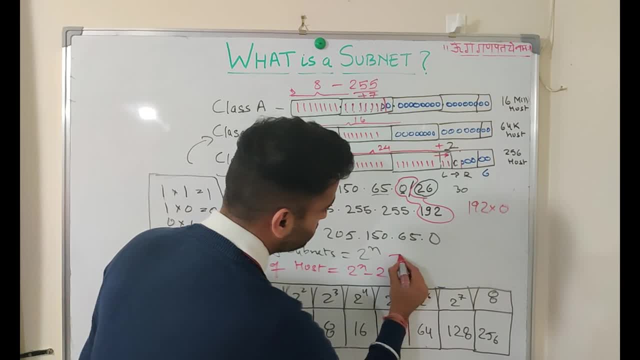 So a quick thing to do in this case is if you open your Windows laptop, you will have to calculate it back to decimal and then that will be your network ID, But it is. it can be very, very difficult task. So a quick thing to do in this case is, if you open your Windows laptop, you will have 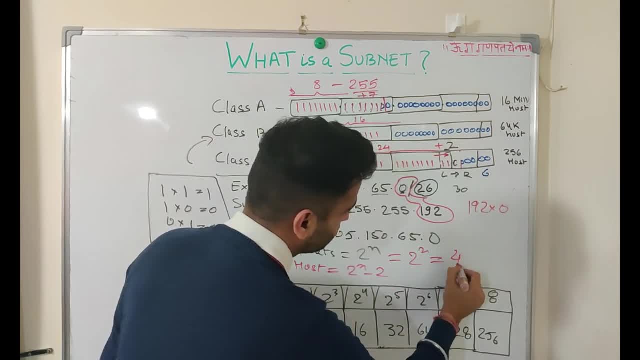 to calculate it back to decimal and then that will be your network ID. But it is. it can be very, very difficult task. So a quick thing to do in this case is, if you open your Windows laptop, you will have to calculate it back to decimal and then that will be your network ID. 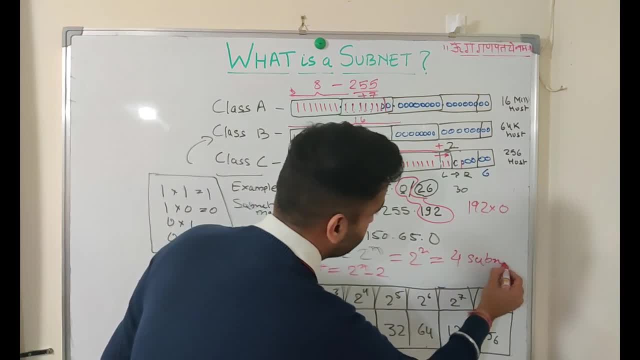 But it is. it can be very, very difficult task. So a quick thing to do in this case is if you open your Windows laptop, you will have to calculate it back to decimal and then that will be your network ID. But it is. it can be very, very difficult task. 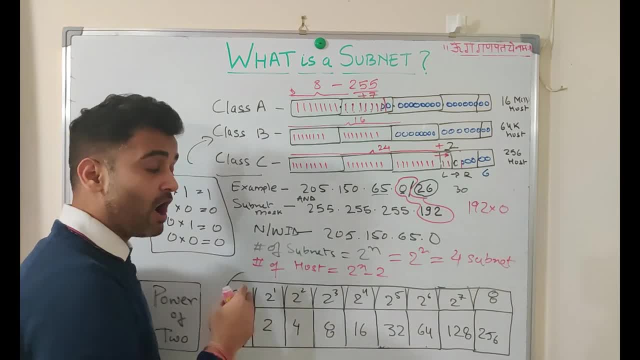 So a quick thing to do in this case is if you open your Windows laptop, you will have to calculate it back to decimal and then that will be your network ID, But it is. it can be very, very difficult task. So a quick thing to do in this case is, if you open your Windows laptop, you will have 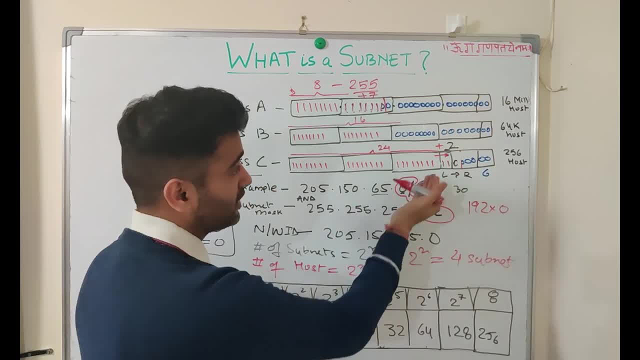 to calculate it back to decimal and then that will be your network ID. But it is. it can be very, very difficult task. So a quick thing to do in this case is, if you open your Windows laptop, you will have to calculate it back to decimal and then that will be your network ID. 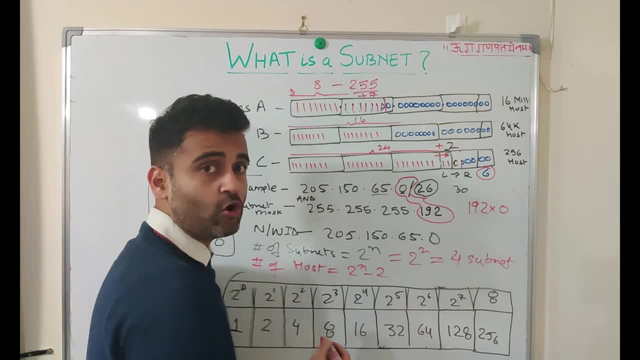 But it is. it can be very, very difficult task. So a quick thing to do in this case is if you open your Windows laptop, you will have to calculate it back to decimal and then that will be your network ID. But it is. it can be very, very difficult task. 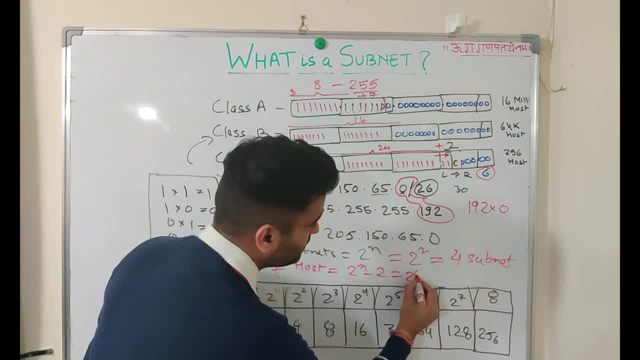 So a quick thing to do in this case is if you open your Windows laptop, you will have to calculate it back to decimal and then that will be your network ID, But it is. it can be very, very difficult task. So a quick thing to do in this case is, if you open your Windows laptop, you will have 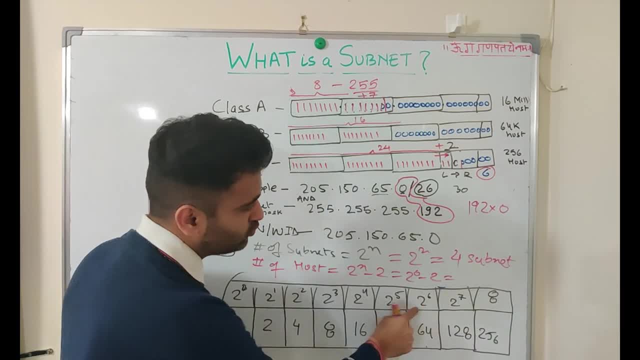 to calculate it back to decimal and then that will be your network ID. But it is. it can be very, very difficult task. So a quick thing to do in this case is, if you open your Windows laptop, you will have to calculate it back to decimal and then that will be your network ID. 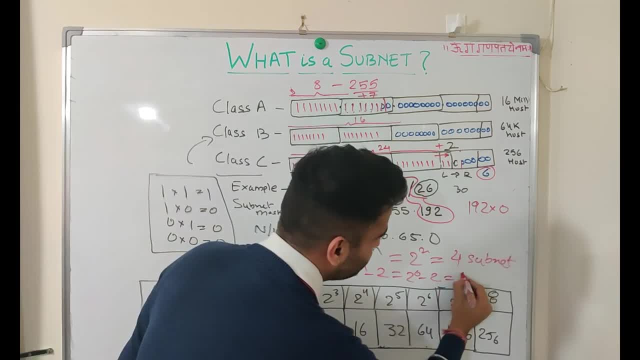 But it is. it can be very, very difficult task. So a quick thing to do in this case is if you open your Windows laptop, you will have to calculate it back to decimal and then that will be your network ID. But it is. it can be very, very difficult task. 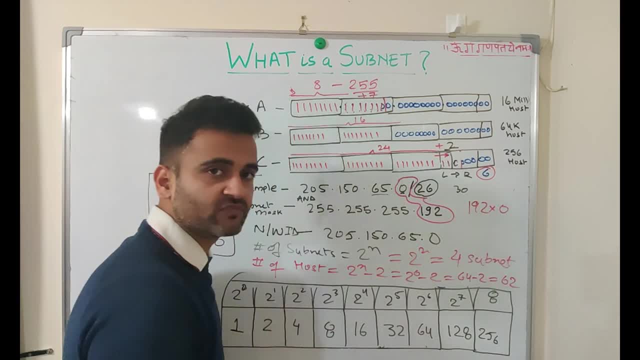 So a quick thing to do in this case is if you open your Windows laptop, you will have to calculate it back to decimal and then that will be your network ID, But it is. it can be very, very difficult task. So a quick thing to do in this case is, if you open your Windows laptop, you will have 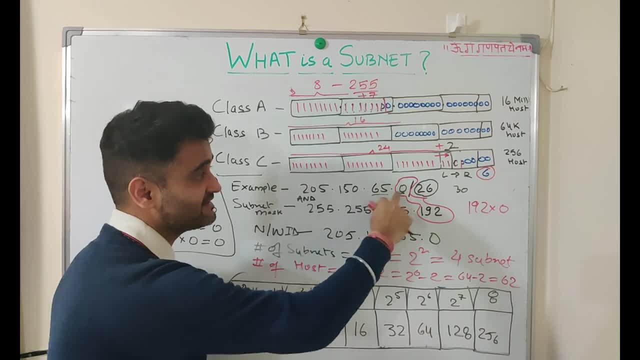 to calculate it back to decimal and then that will be your network ID. But it is. it can be very, very difficult task. So a quick thing to do in this case is, if you open your Windows laptop, you will have to calculate it back to decimal and then that will be your network ID. 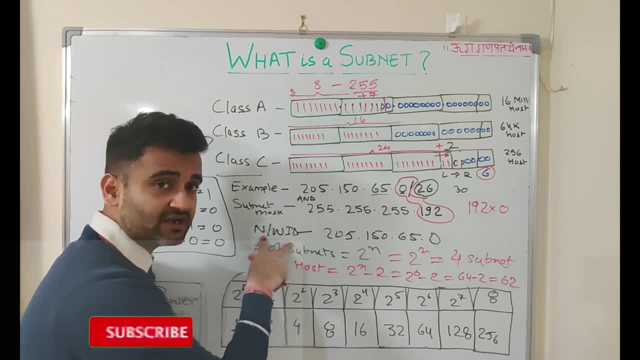 But it is. it can be very, very difficult task. So a quick thing to do in this case is if you open your Windows laptop, you will have to calculate it back to decimal and then that will be your network ID. But it is. it can be very, very difficult task. 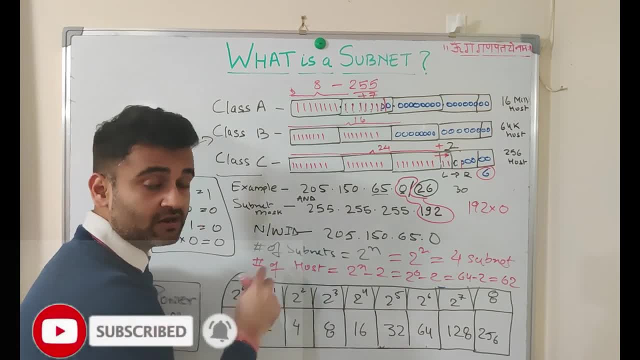 So a quick thing to do in this case is if you open your Windows laptop, you will have to calculate it back to decimal and then that will be your network ID, But it is. it can be very, very difficult task. So a quick thing to do in this case is, if you open your Windows laptop, you will have 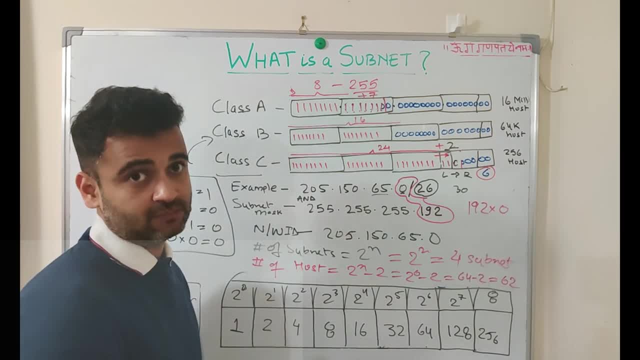 to calculate it back to decimal and then that will be your network ID. But it is. it can be very, very difficult task. So a quick thing to do in this case is, if you open your Windows laptop, you will have to calculate it back to decimal and then that will be your network ID. 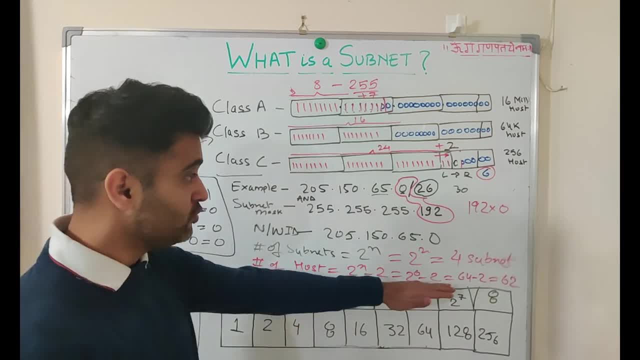 But it is. it can be very, very difficult task. So a quick thing to do in this case is if you open your Windows laptop, you will have to calculate it back to decimal and then that will be your network ID. But it is. it can be very, very difficult task. 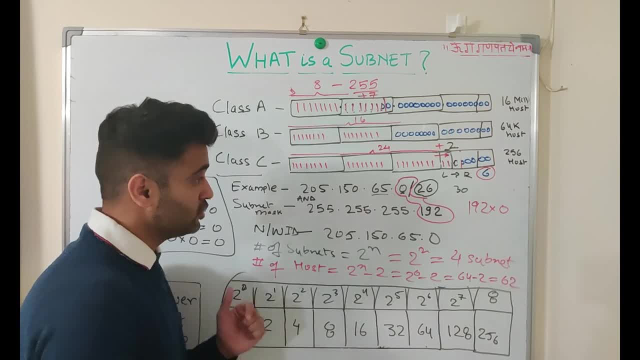 So a quick thing to do in this case is if you open your Windows laptop, you will have to calculate it back to decimal and then that will be your network ID, But it is. it can be very, very difficult task. So a quick thing to do in this case is, if you open your Windows laptop, you will have 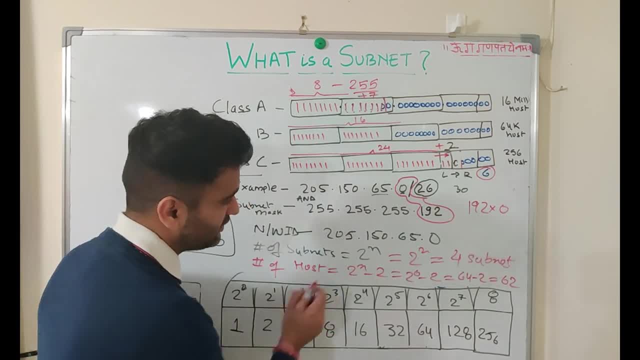 to calculate it back to decimal and then that will be your network ID. But it is. it can be very, very difficult task. So a quick thing to do in this case is, if you open your Windows laptop, you will have to calculate it back to decimal and then that will be your network ID. 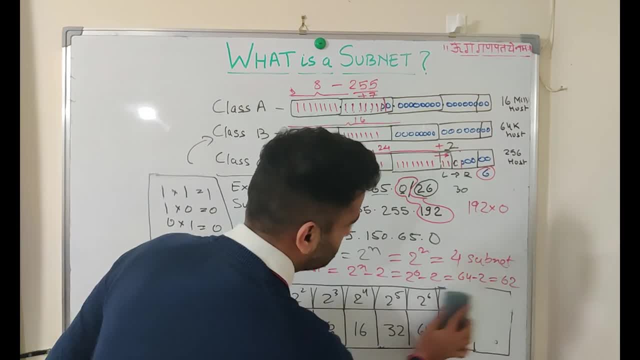 But it is. it can be very, very difficult task. So a quick thing to do in this case is if you open your Windows laptop, you will have to calculate it back to decimal and then that will be your network ID. But it is. it can be very, very difficult task. 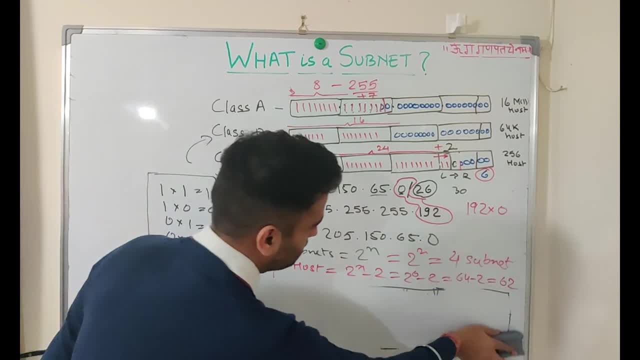 So a quick thing to do in this case is if you open your Windows laptop, you will have to calculate it back to decimal and then that will be your network ID, But it is. it can be very, very difficult task. So a quick thing to do in this case is, if you open your Windows laptop, you will have 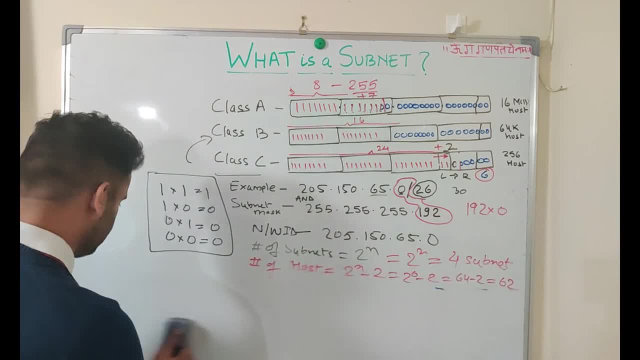 to calculate it back to decimal and then that will be your network ID. But it is. it can be very, very difficult task. So a quick thing to do in this case is, if you open your Windows laptop, you will have to calculate it back to decimal and then that will be your network ID. 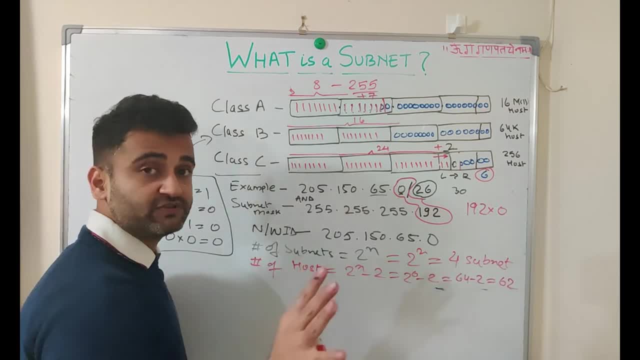 But it is. it can be very, very difficult task. So a quick thing to do in this case is if you open your Windows laptop, you will have to calculate it back to decimal and then that will be your network ID. But it is. it can be very, very difficult task. 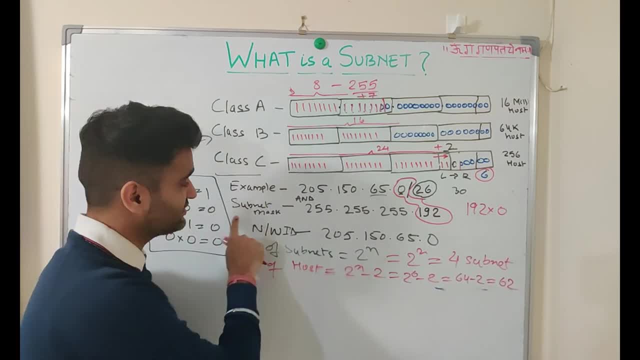 So a quick thing to do in this case is if you open your Windows laptop, you will have to calculate it back to decimal and then that will be your network ID, But it is. it can be very, very difficult task. So a quick thing to do in this case is, if you open your Windows laptop, you will have 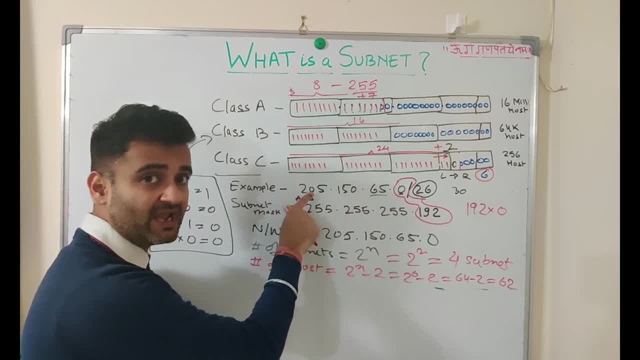 to calculate it back to decimal and then that will be your network ID. But it is. it can be very, very difficult task. So a quick thing to do in this case is, if you open your Windows laptop, you will have to calculate it back to decimal and then that will be your network ID. 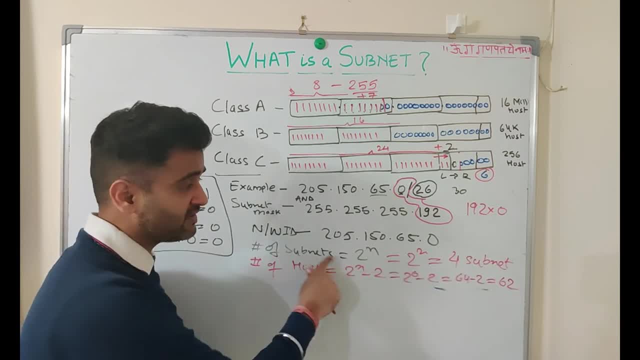 But it is. it can be very, very difficult task. So a quick thing to do in this case is if you open your Windows laptop, you will have to calculate it back to decimal and then that will be your network ID. But it is. it can be very, very difficult task. 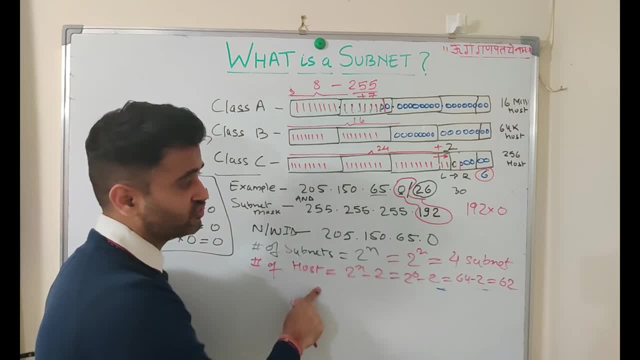 So a quick thing to do in this case is if you open your Windows laptop, you will have to calculate it back to decimal and then that will be your network ID, But it is. it can be very, very difficult task. So a quick thing to do in this case is, if you open your Windows laptop, you will have 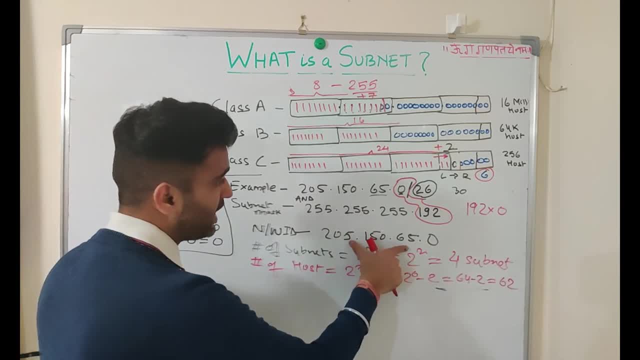 to calculate it back to decimal and then that will be your network ID. But it is. it can be very, very difficult task. So a quick thing to do in this case is, if you open your Windows laptop, you will have to calculate it back to decimal and then that will be your network ID. 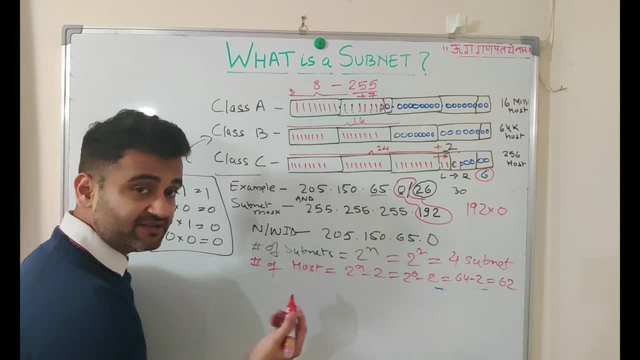 But it is. it can be very, very difficult task. So a quick thing to do in this case is if you open your Windows laptop, you will have to calculate it back to decimal and then that will be your network ID. But it is. it can be very, very difficult task. 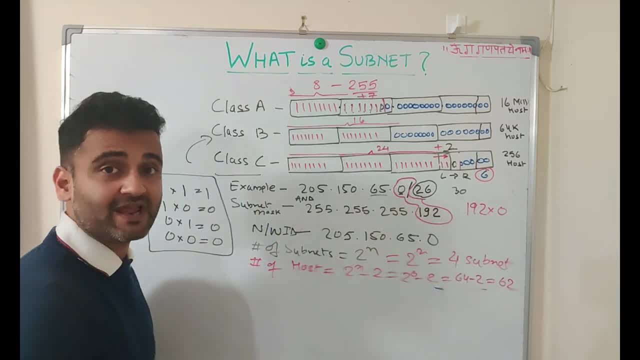 So a quick thing to do in this case is if you open your Windows laptop, you will have to calculate it back to decimal and then that will be your network ID, But it is. it can be very, very difficult task. So a quick thing to do in this case is, if you open your Windows laptop, you will have 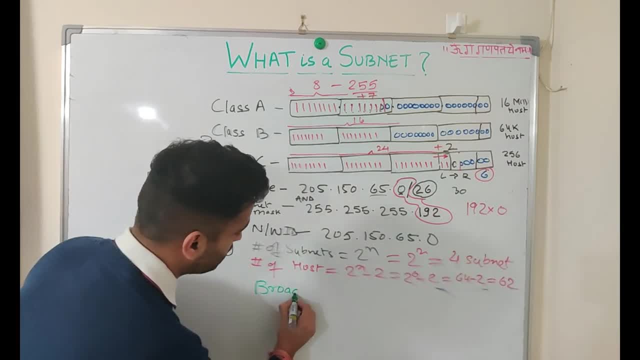 to calculate it back to decimal and then that will be your network ID. But it is. it can be very, very difficult task. So a quick thing to do in this case is, if you open your Windows laptop, you will have to calculate it back to decimal and then that will be your network ID. 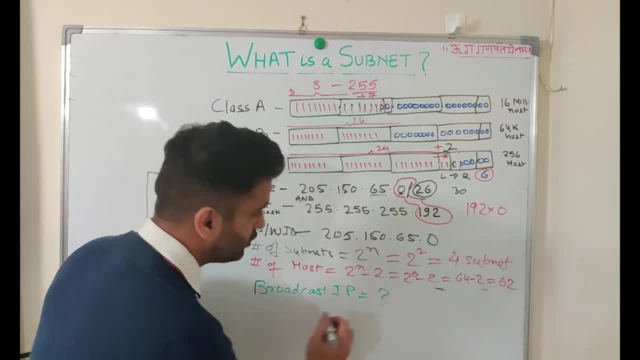 But it is. it can be very, very difficult task. So a quick thing to do in this case is if you open your Windows laptop, you will have to calculate it back to decimal and then that will be your network ID. But it is. it can be very, very difficult task. 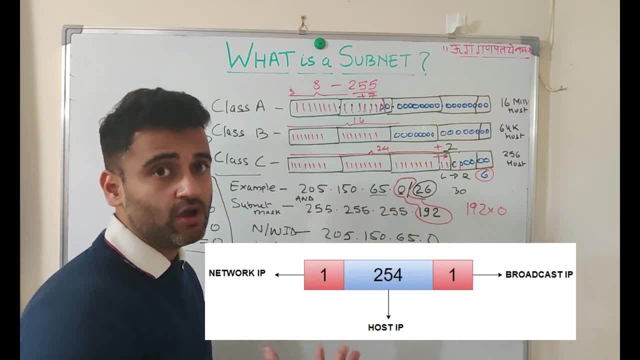 But it is. it can be very, very difficult task, So always remember those middle ones that are for anchors. As I told you, in any subnet, your first ip is your network, the last ip is your broadcast and the middle ones are your host. ok, 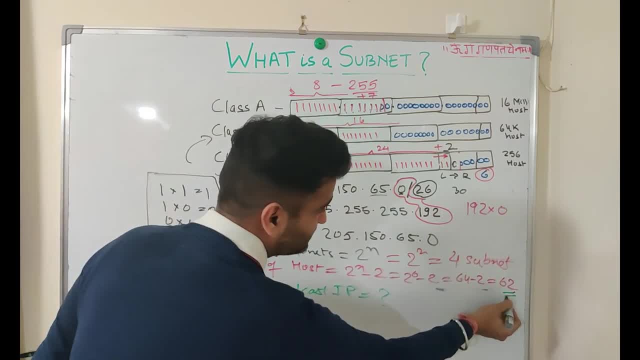 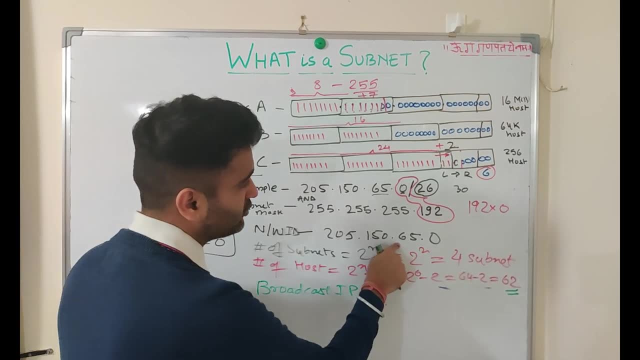 Always remember that. So how many hosts you can accommodate here? 62.. So what would be your broadcast ip? So first, ip started with 205150.65.0. This is your network and you are working here as an authority here Now, if we talk about host networks, 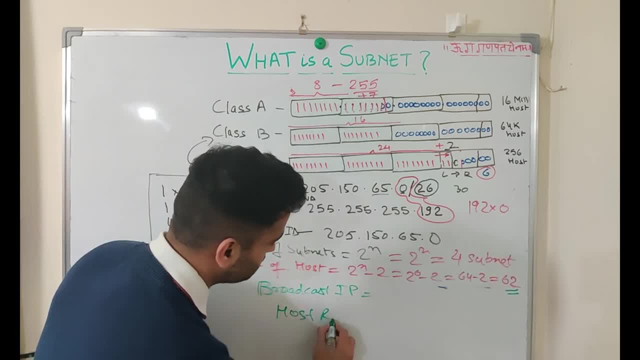 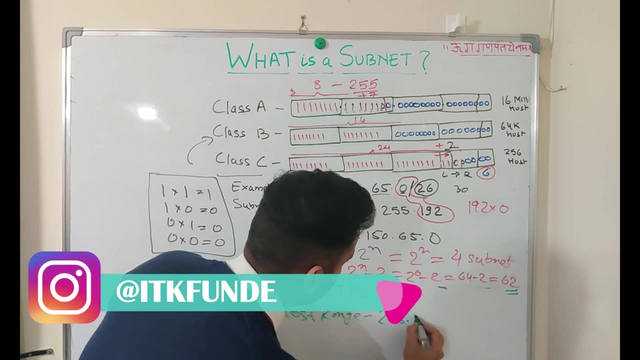 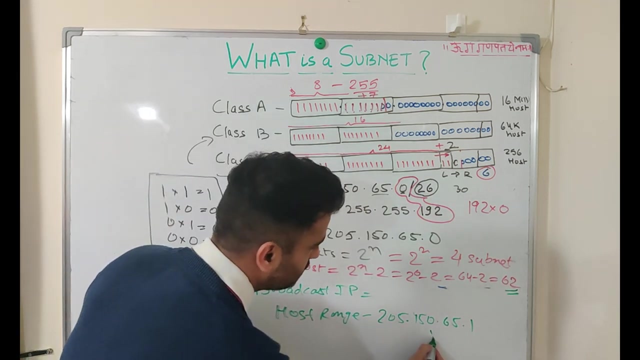 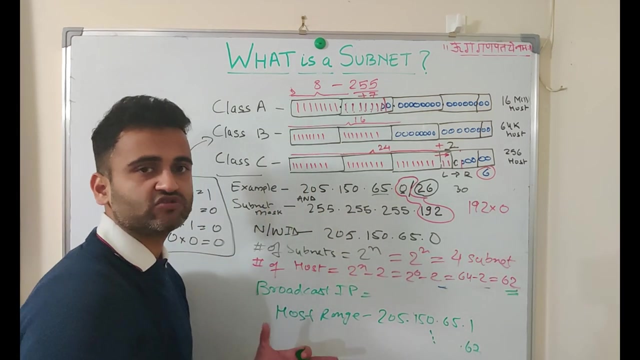 host range. so host range, which a host range? how it will start, just take that example. okay, so host range would be 205.150.65.1. from here it will start and it will go dot, dot, dot and then it will go till dot 62, because you can only have 62 hosts in one particular- uh, you know- subnet. so, guys, by 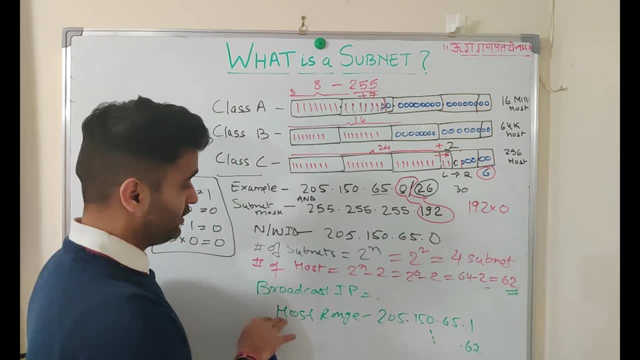 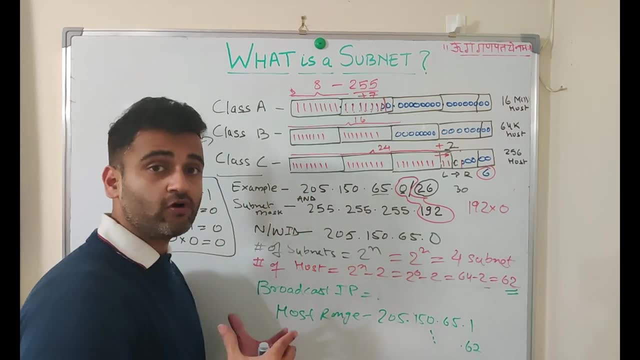 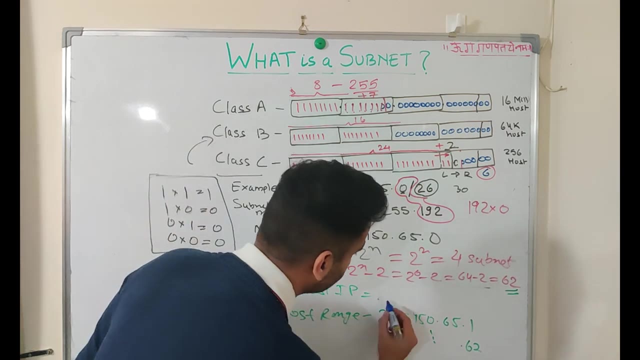 just by looking at your network id, which starts with dot zero, and looking your host range, which starts from one and ends at 62.62, because you can only have 62 hosts by default, it's very, very evident that after all these three, the last ip would be your broadcast ip. so what, what it would? 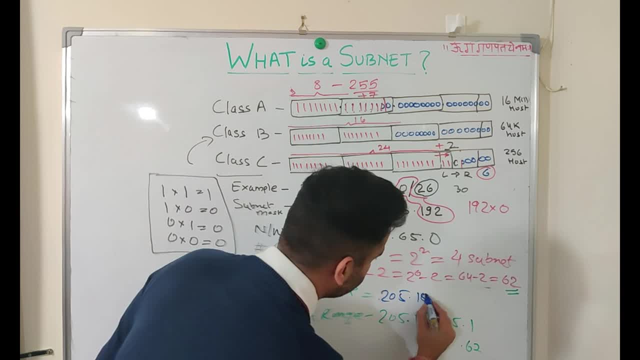 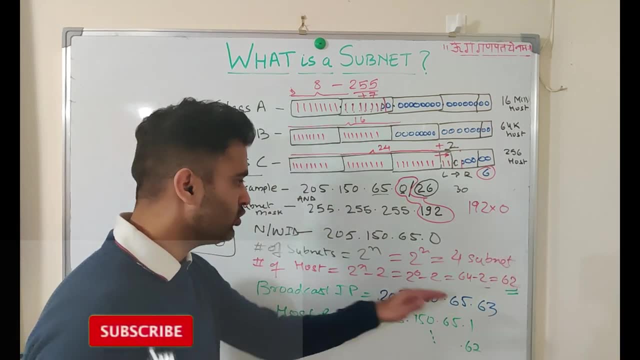 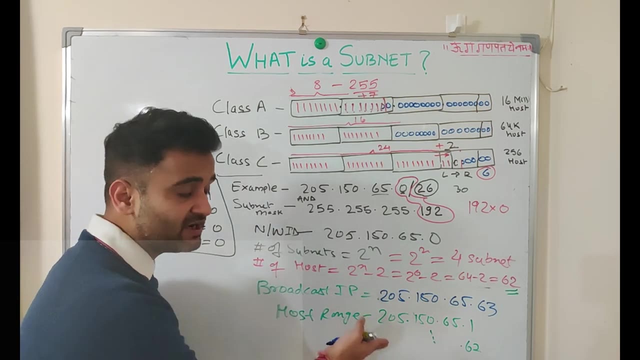 be. it would be 205.150.65.63. so this would be your broadcast ip. after, after you know, after counting your network and your host ips, the last one would be your 63, and then you can continue in this manner and you can create four different- uh, you know- networks from it. so 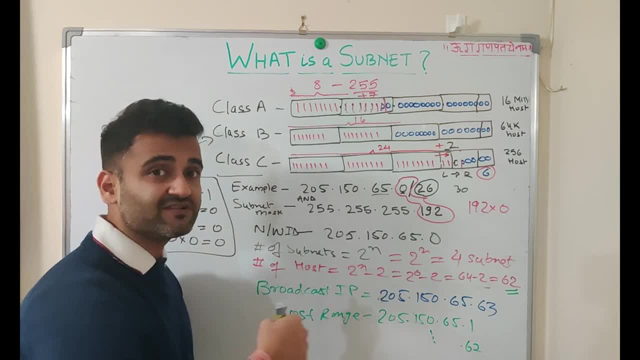 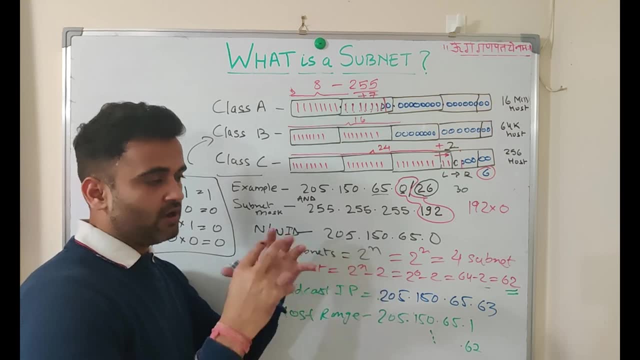 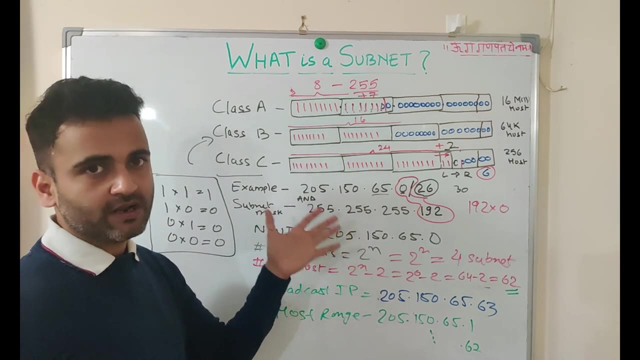 your next uh network address will start from dot 64 and then it can go. so you will have four different blocks of subnets which can be dedicated and which can be uh clearly utilized. okay, now, this is the way. just by looking at the example, an ip address example and a. 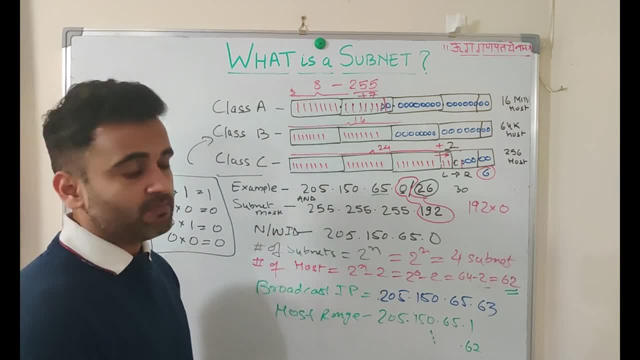 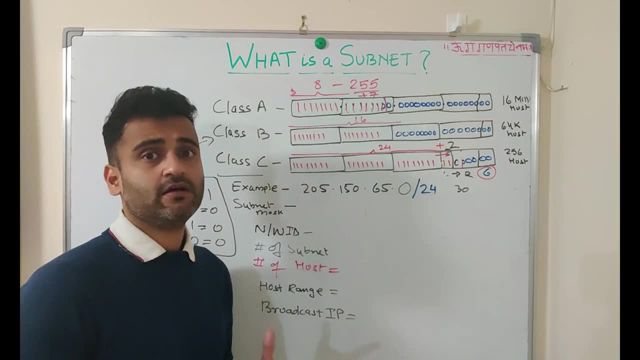 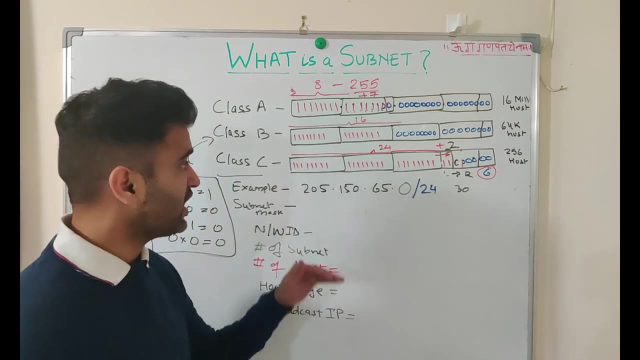 data range you can derive uh, so many details, but there can be another uh question which can be asked. now, friends, let's take another uh, another example to identify that how we can get another kind of queries in subnetting. so suppose i have. i have been given this ip address with slash 24 notation. 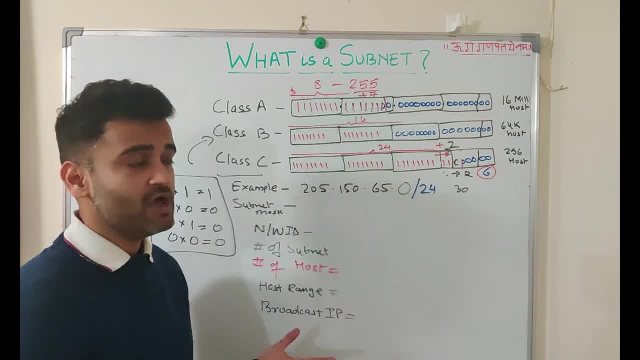 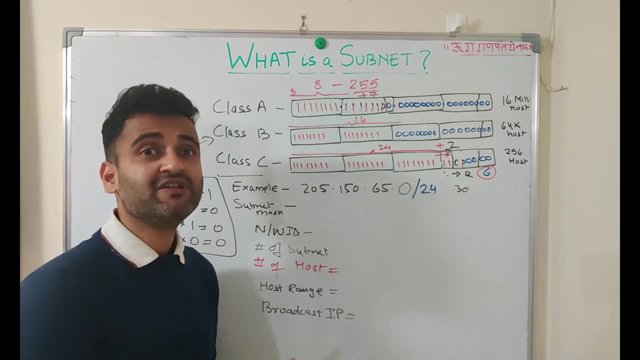 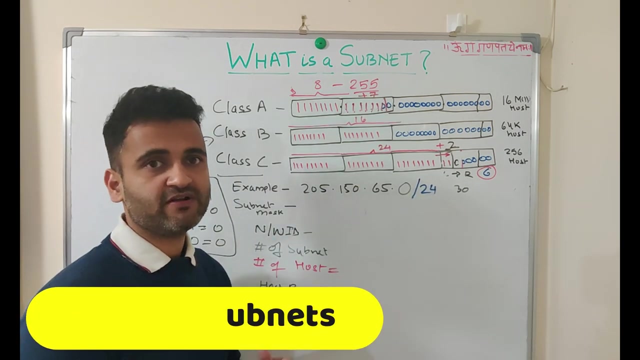 which is standard uh notation for a class c ip address, so its subnet mask would be 255.255.255.0. now i have been asked that you create 10 subnets- 10 subnets- out of this particular ip address. just by looking into this particular ip address, you derive 10 subnets out of it. so now how you will. 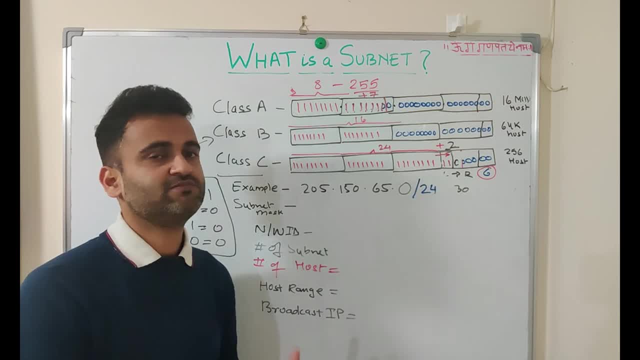 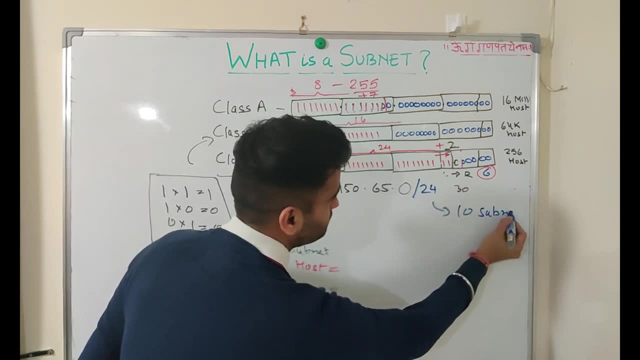 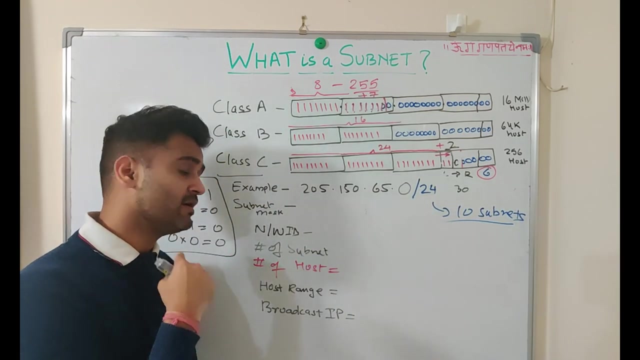 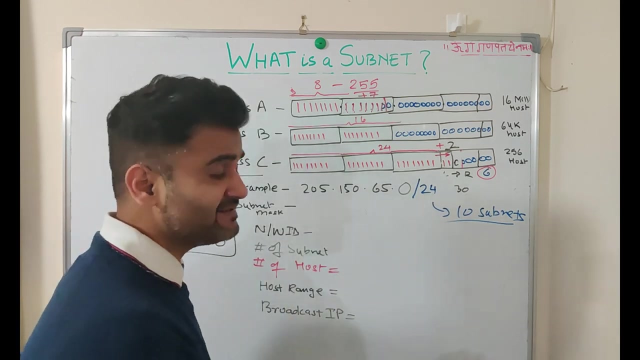 do it. so the mechanism would flip a bit, but i will try to explain it. uh, so, as, as the question says, create 10 subnets. okay, so we clearly know that. we clearly know that we need 10 subnets. so, as we remember, uh, the, the formula for creating the subnet was 2 to the power n. okay, so in this case, 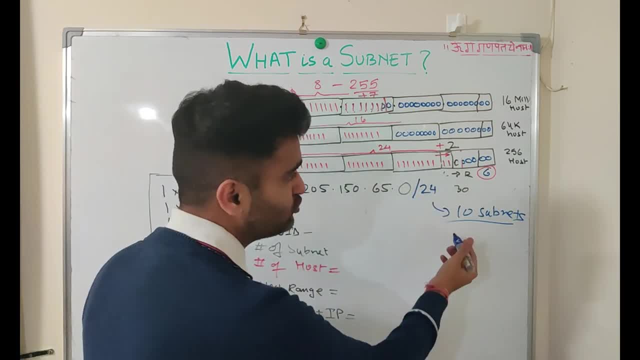 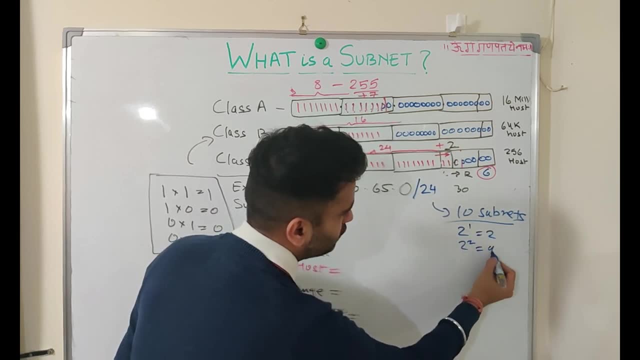 we have to remember the power of 2 table, okay, and try to see where 10 fits into that. so if we take 2 to the power 1, it's 2, 2 to the power 2, it's 4, 2 to the power 3, it's 8 and 2 to the power 4 is 16. 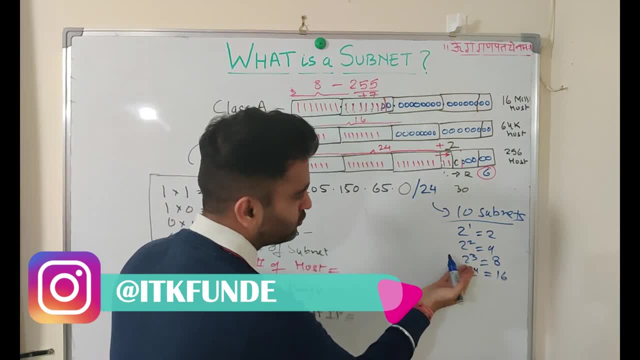 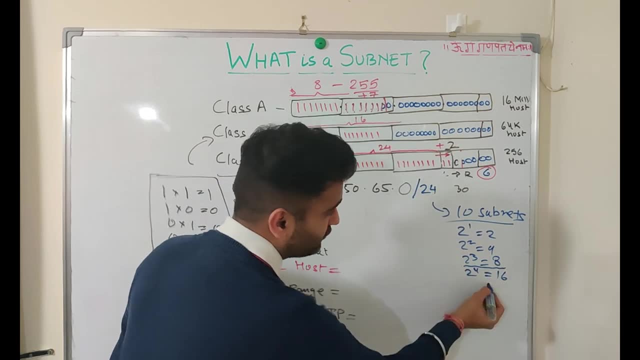 right, so we have 2 to the power 1, 2 to the power 2, 2 to the power 3 and 2 to the power 4.. so in order to create 10 subnets- you cannot use until up till here- you have to use this particular uh subnet. okay, so what it is. it is using four bits, so in: 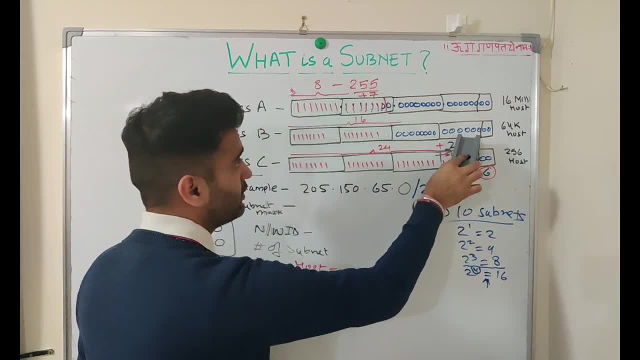 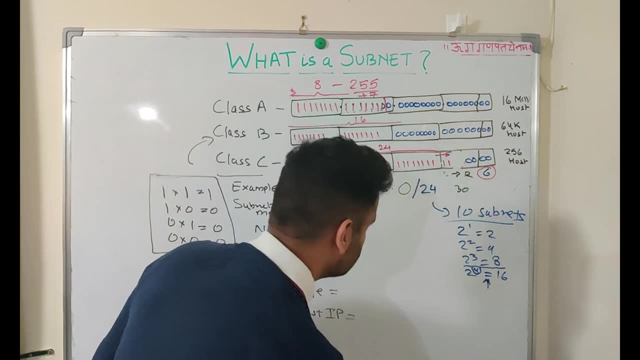 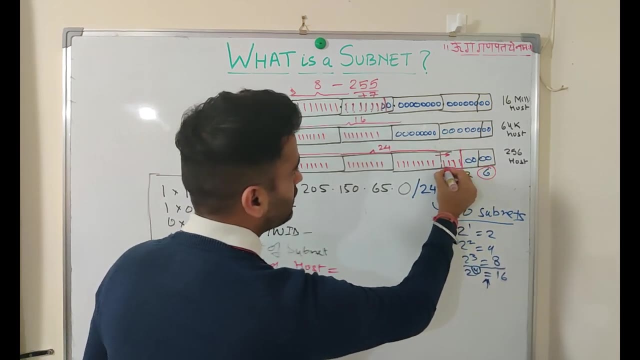 this case, instead of- you know our previous example- we have to now go and we have to now take more uh space into this particular octet. so now we are saying that we need four bits. okay, so one, two, three, four, okay. so what will be your cider range now if you have to get 10 subnet, so if you have to derive it? 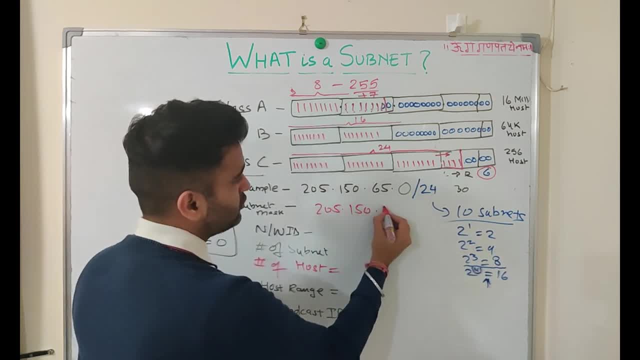 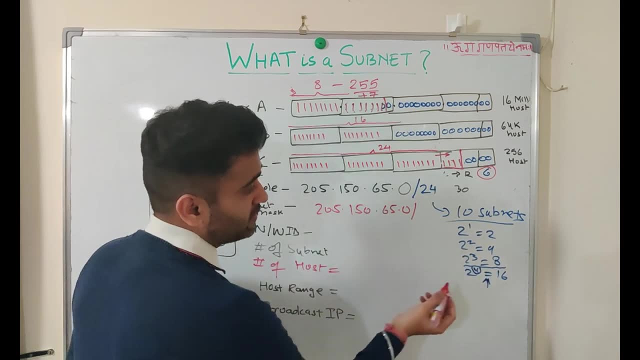 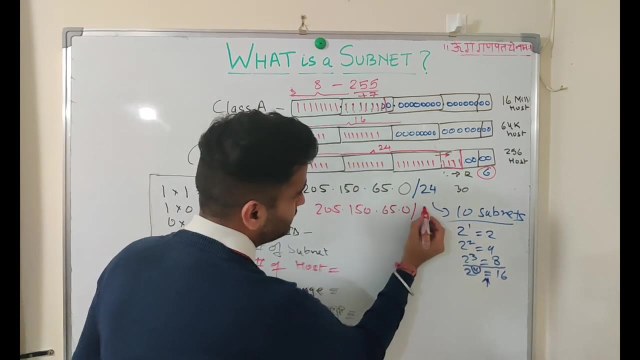 again, so it would be 205.150.65.0. slash. now. 24 was by default. now for creating four subnets, you have to encroach into your host. get some more out of that. so in that you will have 28, because what you 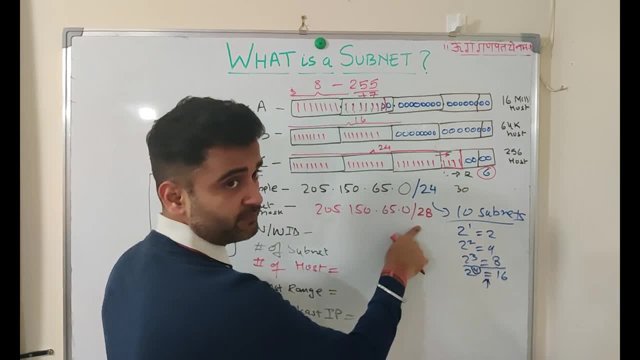 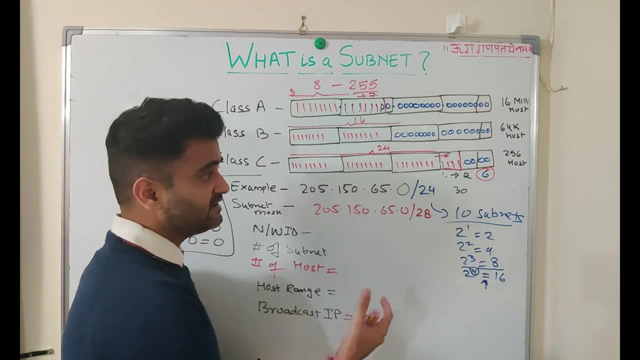 have to do is you have to take the subnets out of your 8 bits. you have taken 4 bits. okay, those four bits you have taken, and now your cider range has become 8. okay, so in this way, what you have done, just by getting the example, 10 subnets you have to create, you simply took that and you, uh, you know. 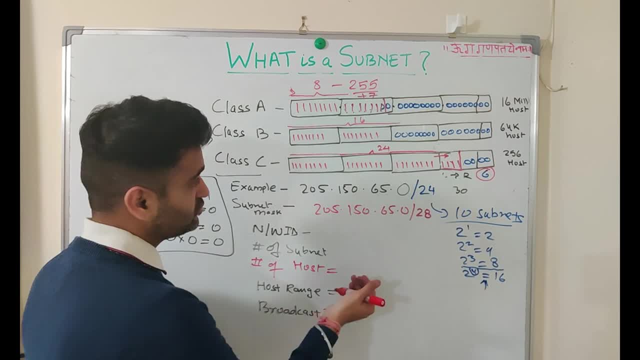 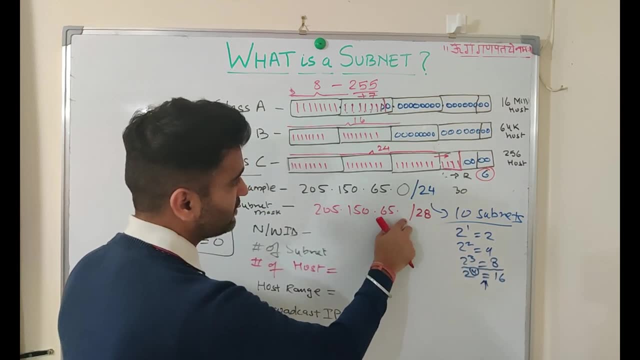 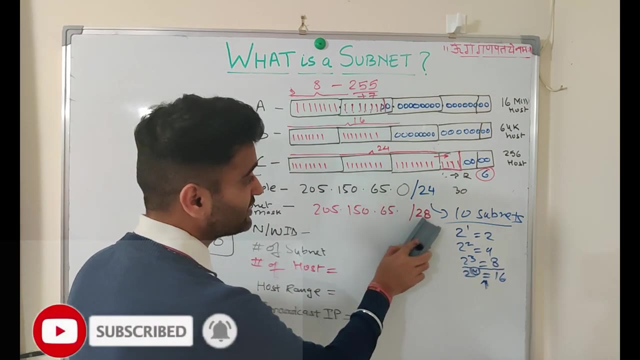 you maintain that now the next i next thing would be to get the network id. in this case also, you have to get, uh, your subnet mask, okay, so your sub, sorry for this mistake. so in this case, your subnet, uh you have to, maybe, uh, sorry, so in this particular subnet mask, your subnet mask would be slash. 28. 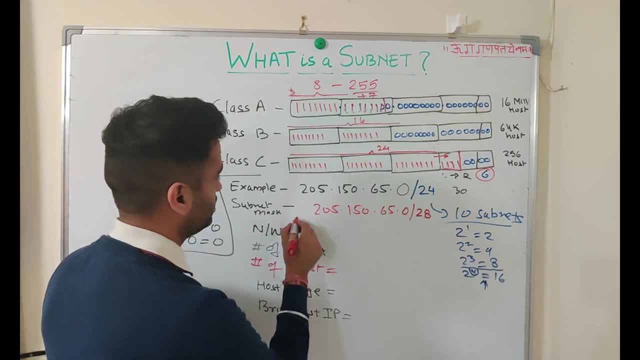 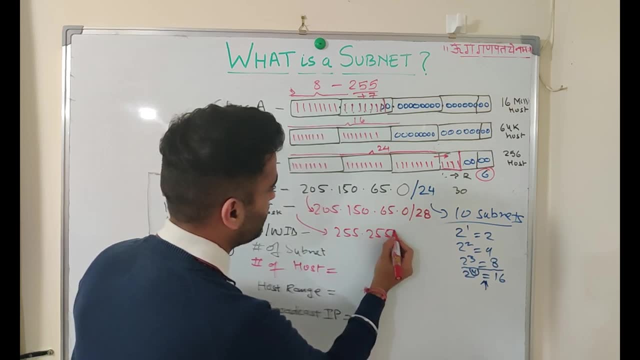 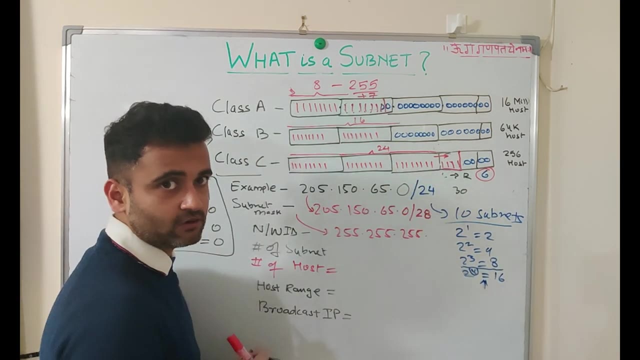 so what it would be? uh, so let me show you the subnet mask. so actually the subnet mask would be 255 dot, 255 dot, 255, dot. now the first four bits you have to add. okay, so first four bits. we have to always go from left to right, okay, so from here you have to. 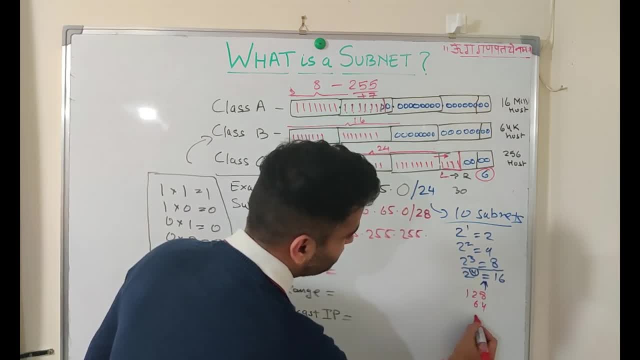 add those bits so it will be 128 plus 64 plus 32 plus 16. why? because it is 2 to the power 7, 2 to the power 6, 2 to the power 5, 2 to the power 4.. so 1, 2, 3, 4 bits, okay. so if you add this, 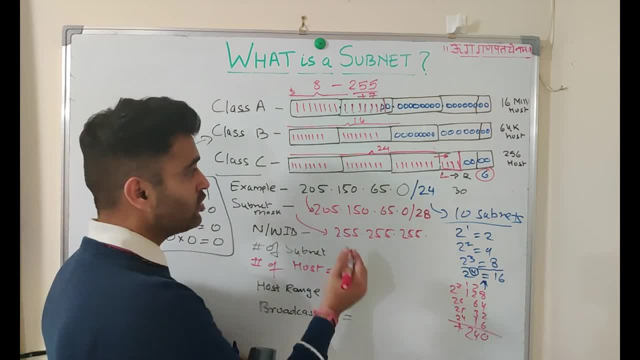 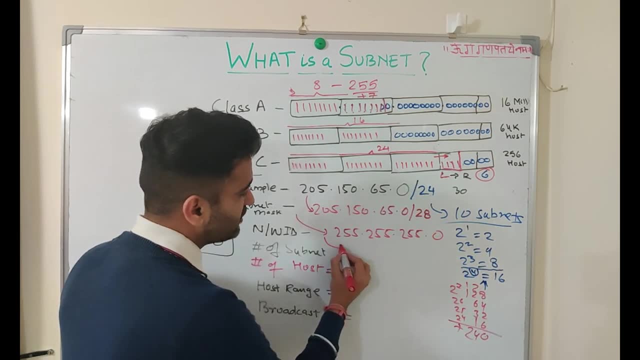 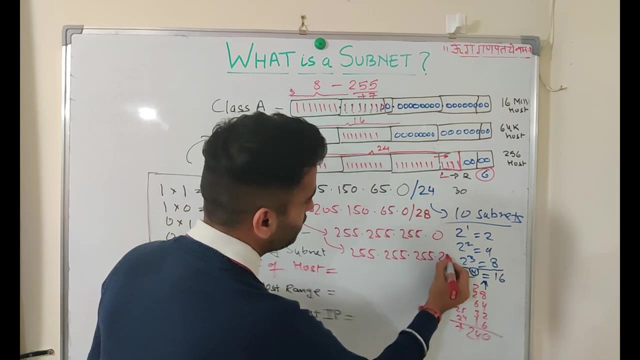 so if you add this, it comes to 240.. so now, instead of your initial subnet mask, which was like this because it was slash 24, now you will have the new subnet mask, which will be 255, dot, 255, dot, 255, dot, 240, because you have now derived that you need 10 subnets and 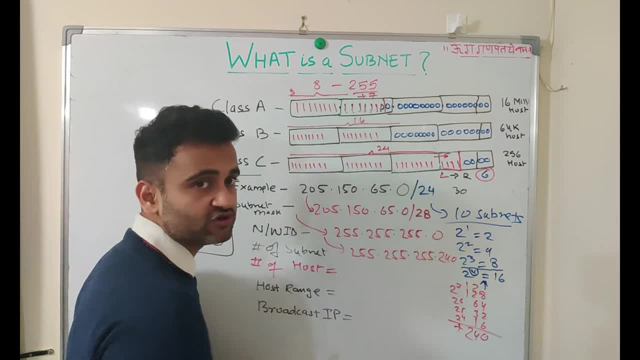 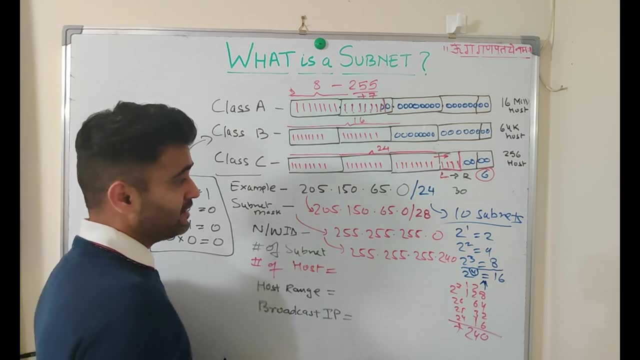 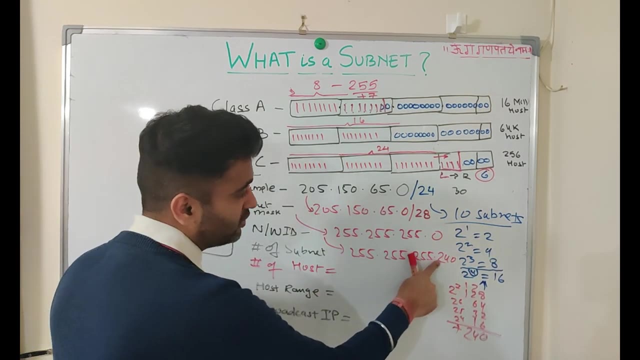 for 10 subnets to be accommodated, you need four bits from your host octet. okay, now you got this far. now what you have to do? you have to understand that. what would be your network id? so for that again, the again the same formula applies. you have to take this particular subnet mask, put it in here. 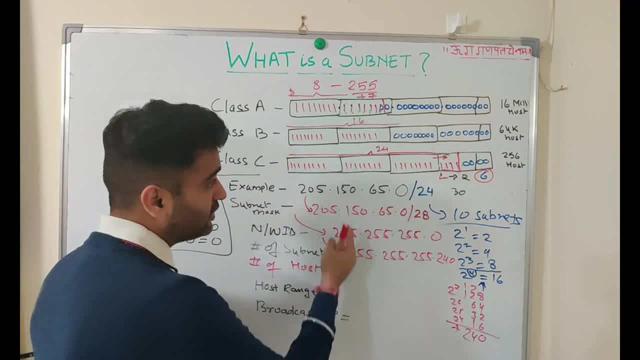 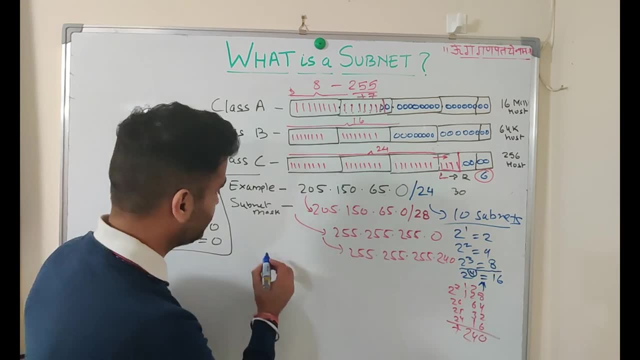 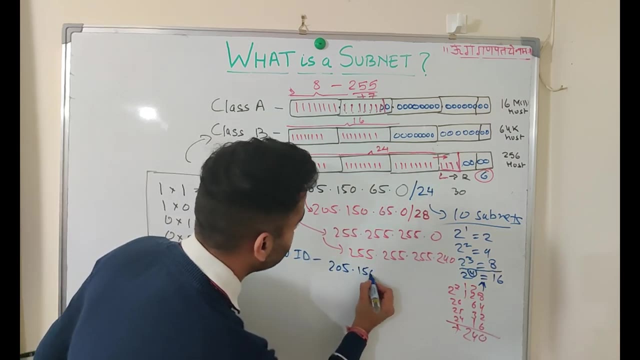 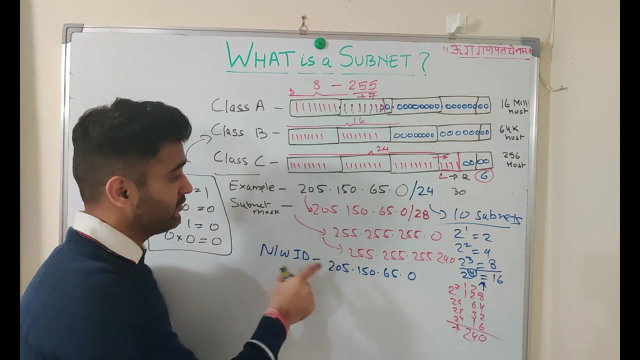 and do the logical and operation. okay, after doing that logical and operation, whatever will be the outcome would be your network id. so, in this case, what will be your network id? your network id would be 205.150.65.0. again, the logical and operation. regardless of what you take for now, if you do an 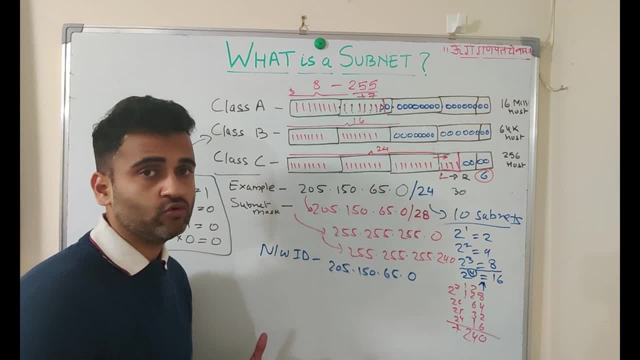 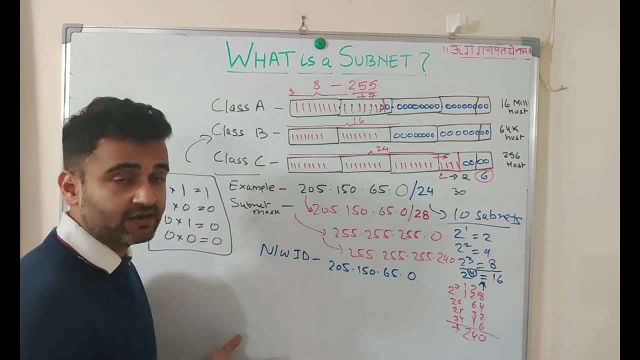 end operation, maybe on a calculator or just converting it into a binary. then it will result into this particular ip address, which will be your network id. now the next part is: we already knew from the beginning that we need 10 subnets. that's why we took 4 bits. 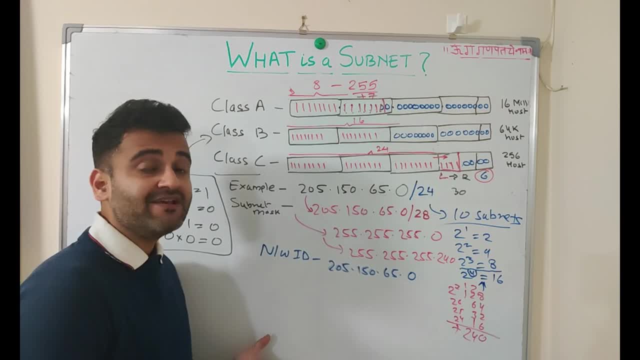 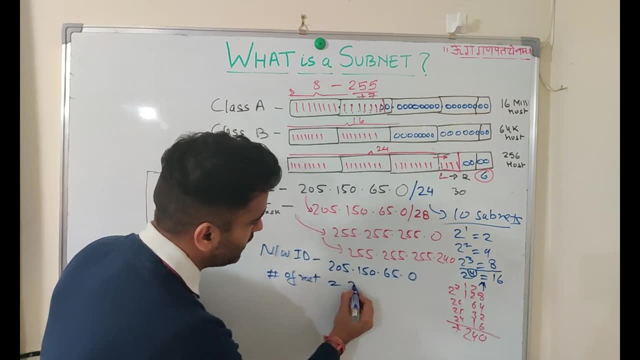 out of this particular octet. now how many are remaining? that will decide how many hosts i can have. so i told you the number of networks is 2 to the power n, which denotes your network bits, and then network number of host is 2 to the power n minus 2 to the power n. 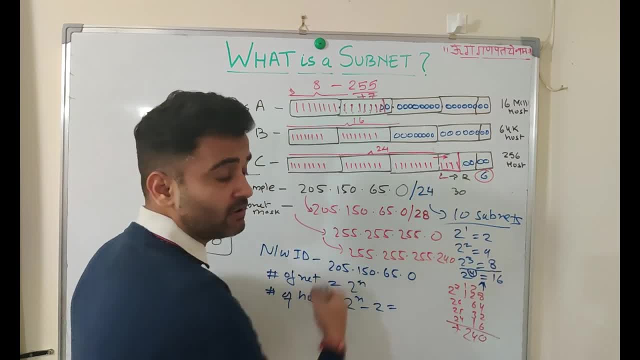 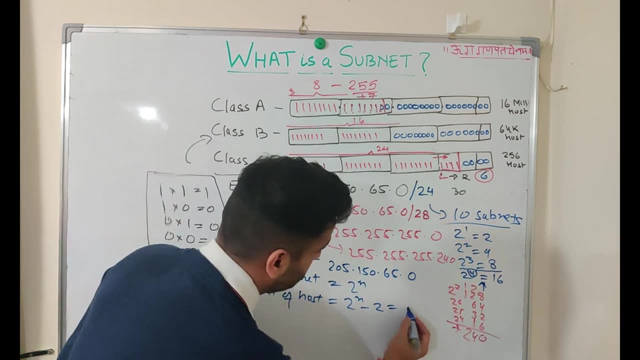 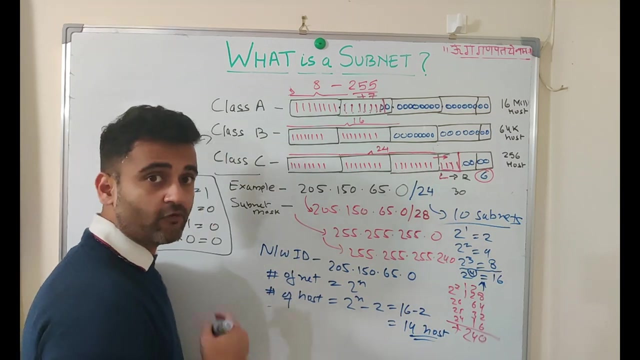 minus 2. so in this case your number of uh host bits are 4, because you have already taken 4 from here. so in this case your uh, you know your, this particular number of hosts would be 2, 2 to the 4 to the 8 to the 16.. so 16 minus 2, so you can have 14 hosts. okay, 14 hosts you can have. and here again, 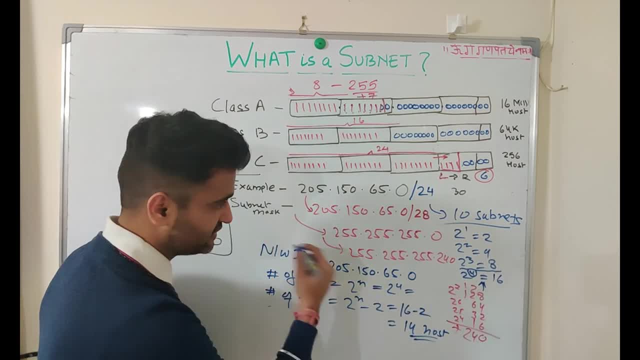 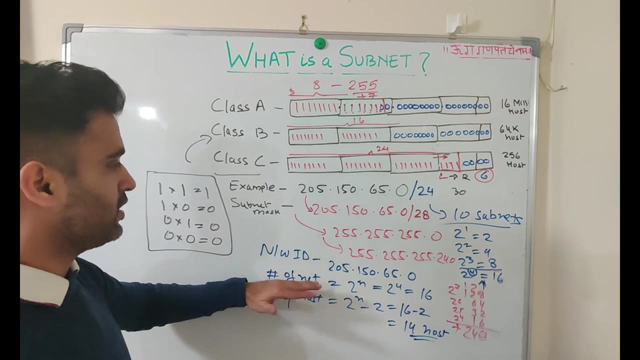 we have already covered. but uh, just for, uh, uh, just for understanding purpose we will have, we can have maximum of 16 subnets, but the actual question was we only need 10 subnets. so that's fine, but we have to accommodate that with this. so now we have 14 hosts here. okay, now, based on your number, uh, your subnet, number of subnets. 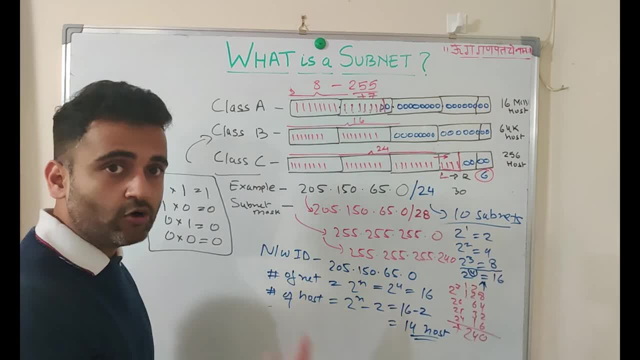 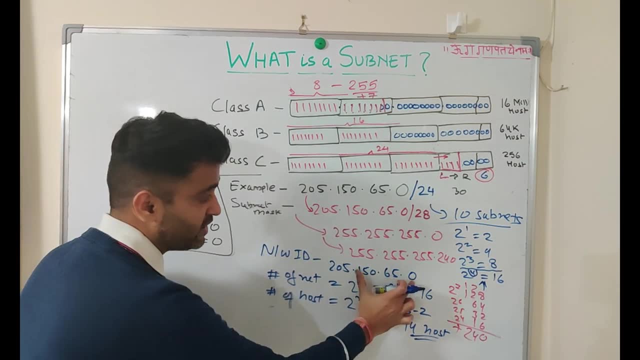 and then number of hosts, and your network id is already there. now you can derive your broadcast id, so your broadcast id will be: you just calculate this. okay, so your first id ip address is 205.150.65.0. after that you will add 14 hosts, so it will start from. so host range. 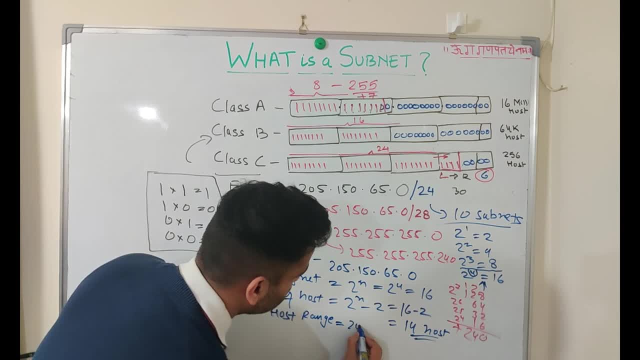 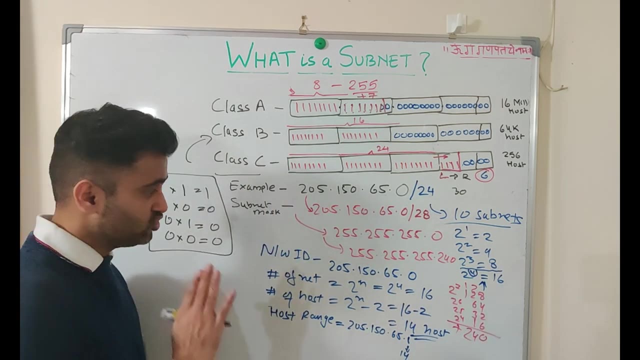 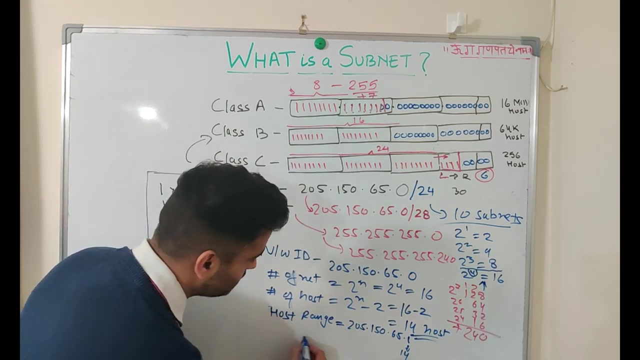 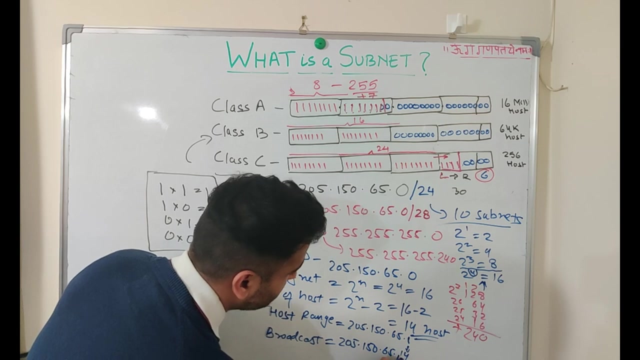 host range will start from 205.150.65.1 and it will go till 14, right? so in that case, what will be your host range, broadcast ip? your broadcast id will be the last ip. so that would be. i hope you guessed it if i have made this tutorial in a better way. so it is 205.150.65.15. 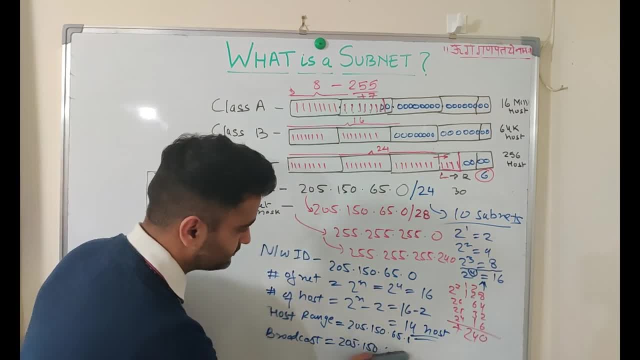 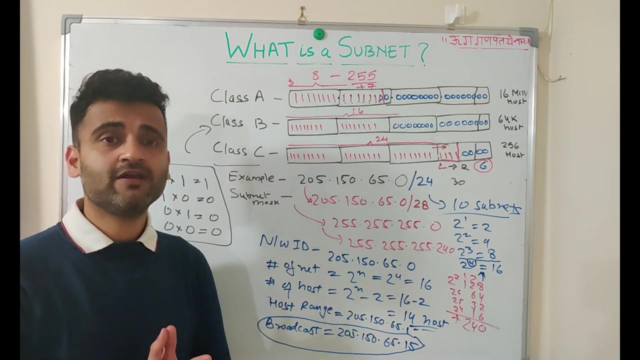 okay, let me write it clearly. so it is 205.150.65.15. okay, so this is your broadcast ip, after giving 14 to the host, one to the one to the network. so, friends, i hope with these two examples you are able to understand subnetting to a better detail and going forward. 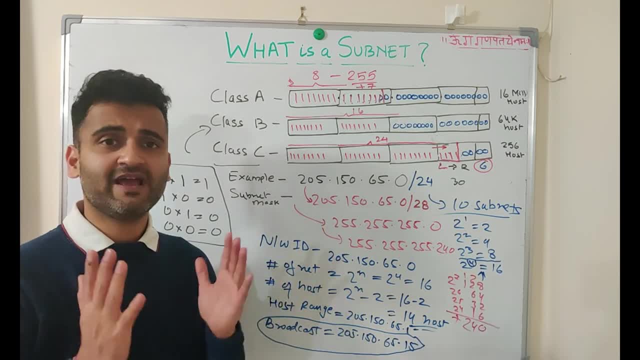 if you want to learn more, you can explore subnetting to a wider detail. it has various subnetting to a wider detail. it has various subnetting to a wider detail. it has various- you know various- levels. so once you start your journey, you will find various different scenarios. 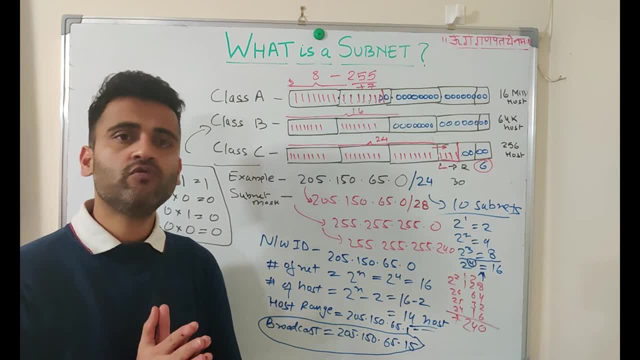 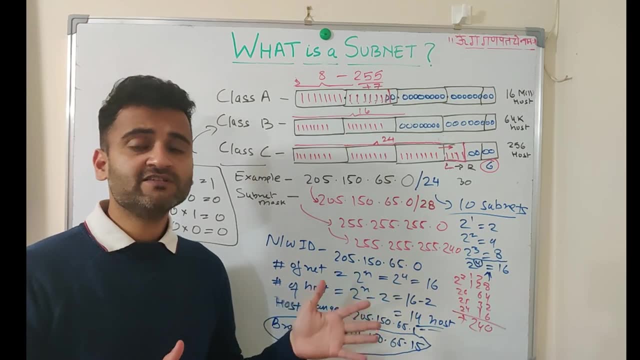 which you can learn as you go forward, but this particular video would give you a good starting point. at least, i hope so. so just to quickly recap: uh, we started with ipv4 basics, then we went into a layman example and understood how subnetting works, and then we understood the basic fundamentals. 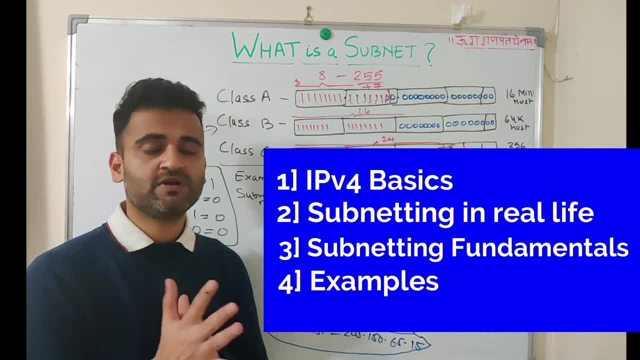 of subnetting, what is, uh, you know, network id, host id, subnet mask. and then eventually we understood how we take it to the next level. and then we went into a layman example and understood how subnetting works. and then we understood how subnetting works. and then we understood how subnetting works and then we 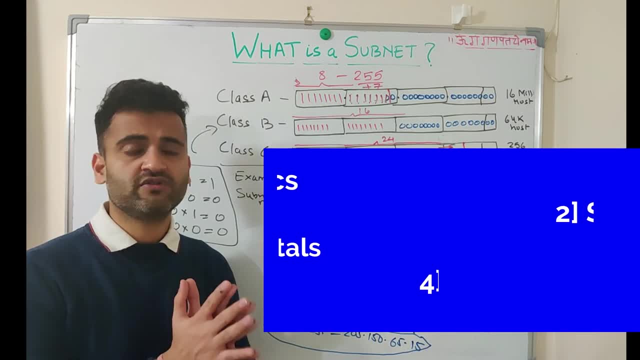 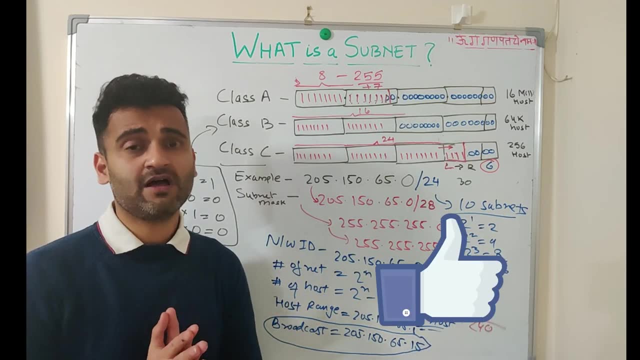 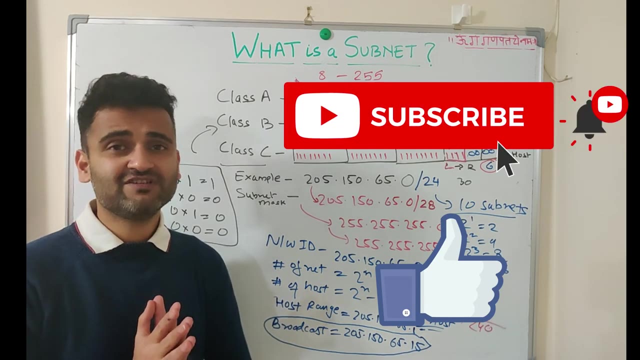 take it and derive subnet mask, broadcast id, network id, host range, everything, taking uh examples. so i hope you like this video. if you did, please hit the thumbs up. let me know in the comment section below what you would want to learn next. and yes, if you have not yet subscribed to this channel, please. 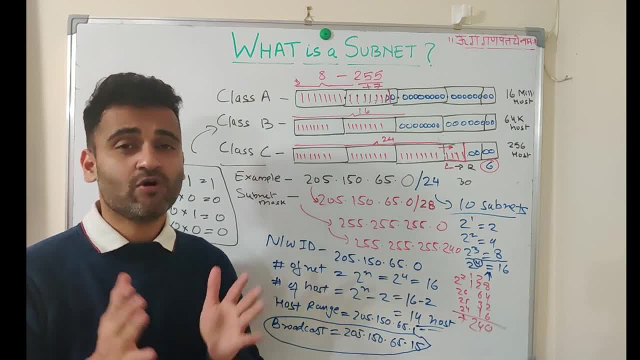 subscribe, because we make it interesting for everyone. so until then, thank you so much and keep hustling bye. for now, 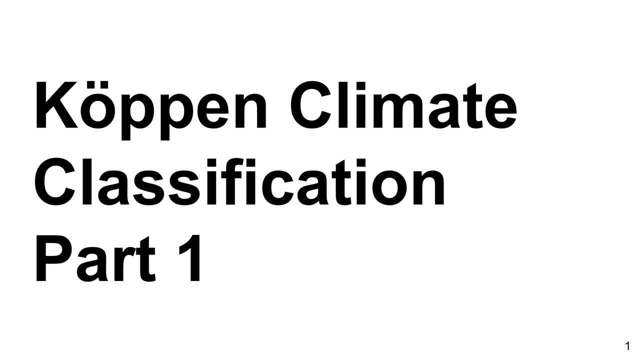 Hey, this is Charlie Thompson, and this is the video for Lab 10 on the Kirpin Climate Classification, Part 1.. I know that Lab 7 was just absolutely brutal, and so we're just going to chill with the math for a little bit. Next week we'll get into a little bit more math, but this week 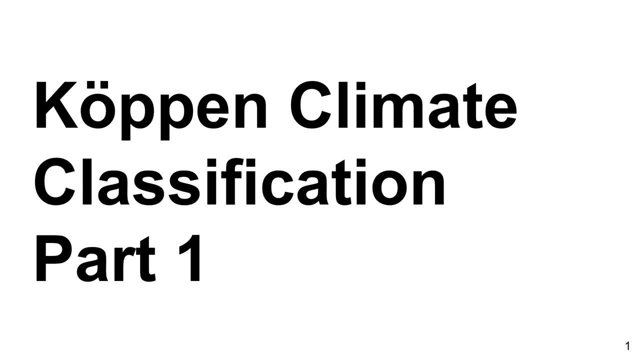 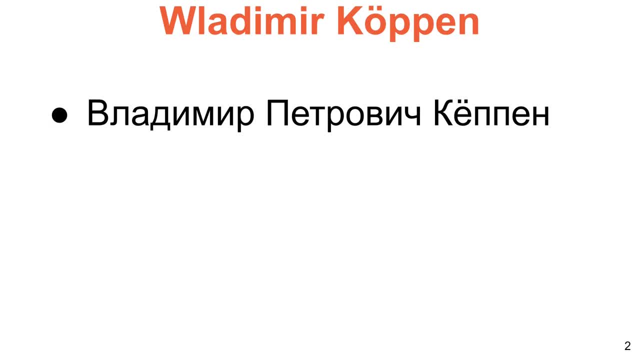 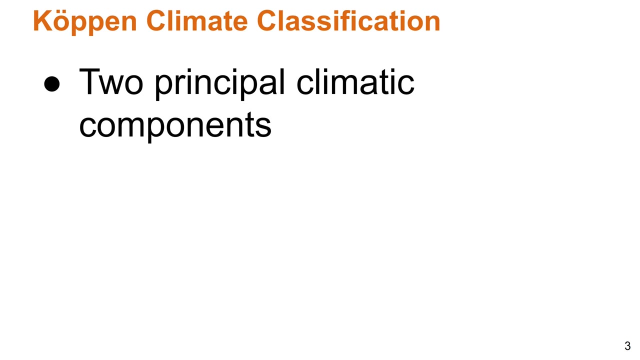 we're not going to do a lot of math, So let's jump in and take a look at the Kirpin Climate Classification System. So Vladimir Kirpin was a Russian-born German meteorologist, Vladimir Petrovich Kirpin, and he developed the Kirpin Climate Classification System, beginning in 1884..